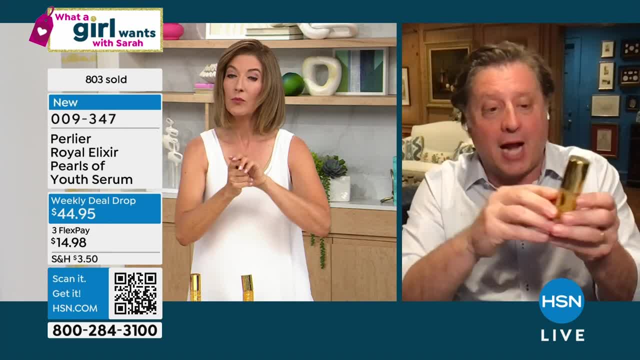 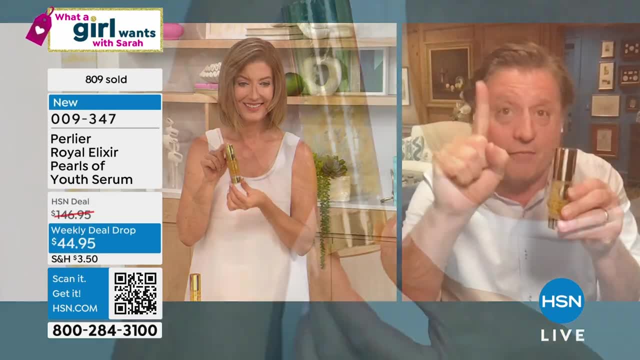 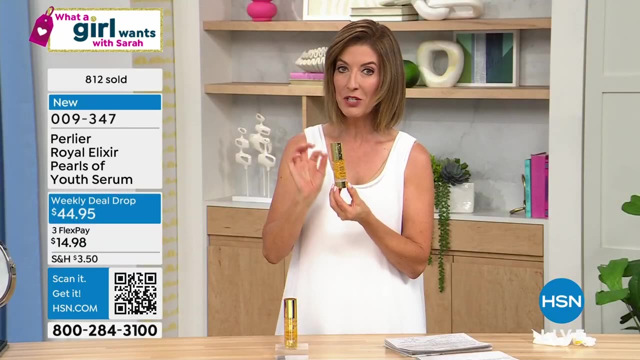 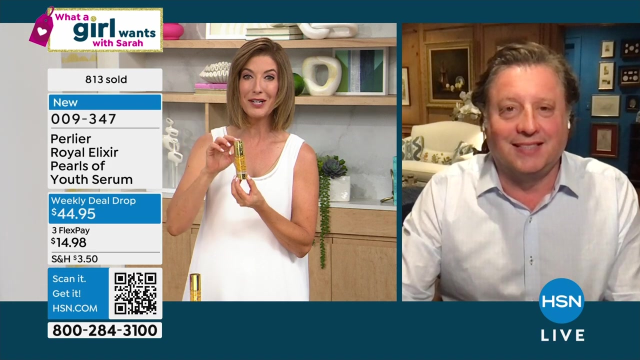 Not alcohol in it, Without real alcohol. We used to have alcohol to actually burst these little bubbles, but now we don't. We've reformulated these bubbles and we can say: deep lines and wrinkles for the first time. Don't need it. It's everything you want: The fresh, living royal jelly, the honey, the botanicals. If you want to see improvement in your deep lines and wrinkles, look no further. You're getting a lot. You're getting $100 off the price. Skip, that's one way to say thank you. during our customer appreciation month, You're giving everyone $100 back. I don't know if anyone else can come close. 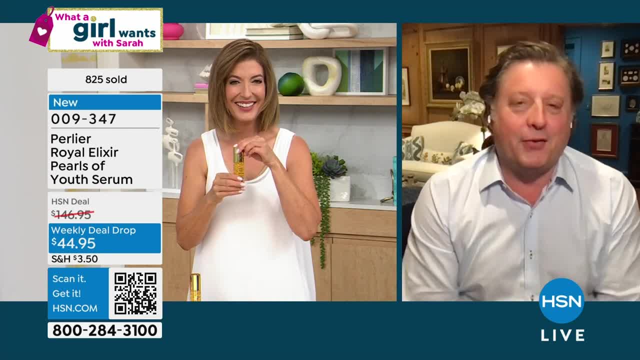 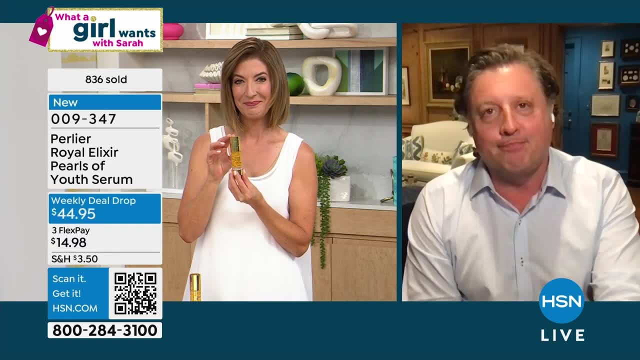 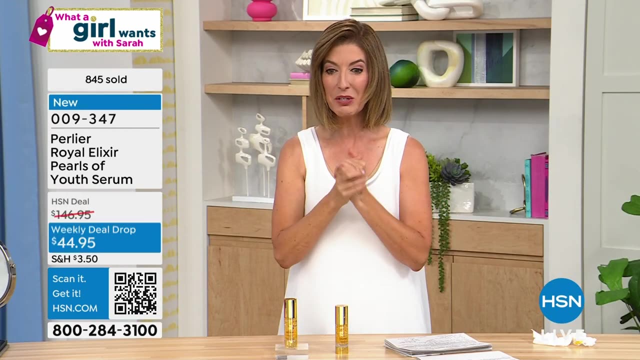 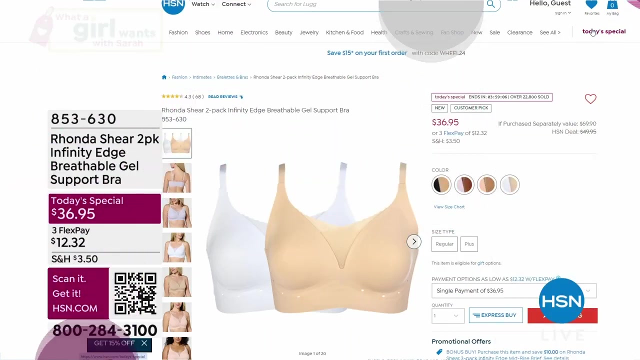 So you've kind of set the bar very high. Well, thank you. Thank you for having me. I really hope all of you get to try this And again, it's the best way I know how to say thank you for the last 28 years. Let's skip. We look forward to your full shows. However, in the meantime, you can shop that online and you can find all of Great Perlier's items. 009347 is your item number. Welcome into our second hour of What a Girl Wants: Happy Tuesday. Oh, I've got to check in. 23,000 of you shopping our best value of the day. I want to. 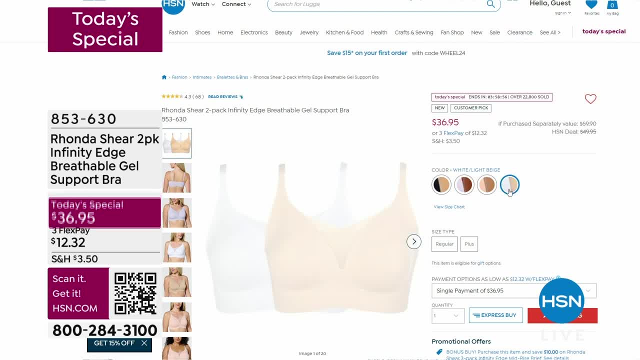 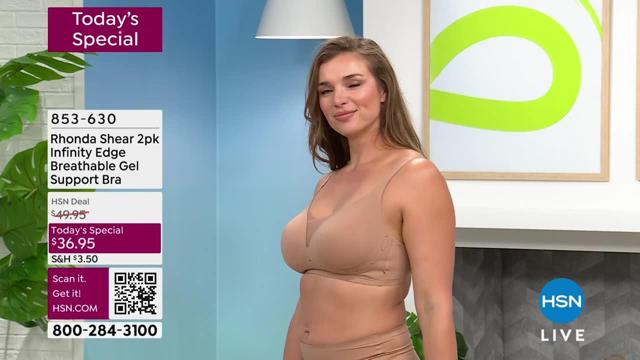 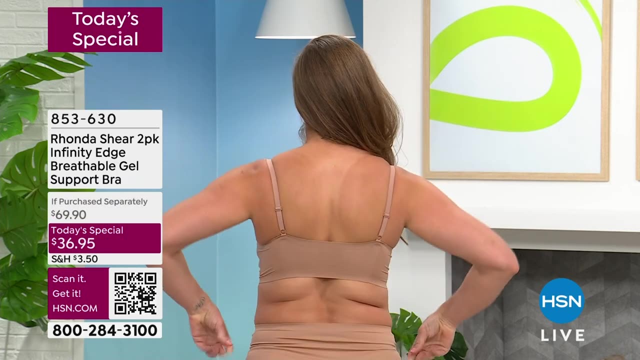 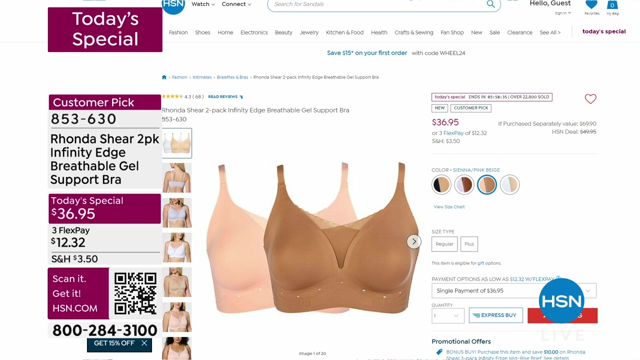 say hello. Linda is here, Glenna is here, Debbie is here, Tracy is here. Did you pick up on our today's special? I hope you don't miss this. This is the best value of the year. It's a two pack on the amazing Ron Deshir Infinity Edge Breathable Gel Support Bra. There is no more underwires, There's no more poking or prodding or tugging or twisting. Full coverage cups: You get removable pads. You get adjustable straps. You get all the beautiful invisible edge, The bonded seams You get. 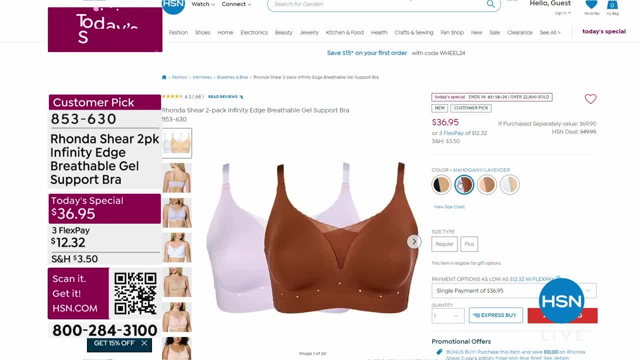 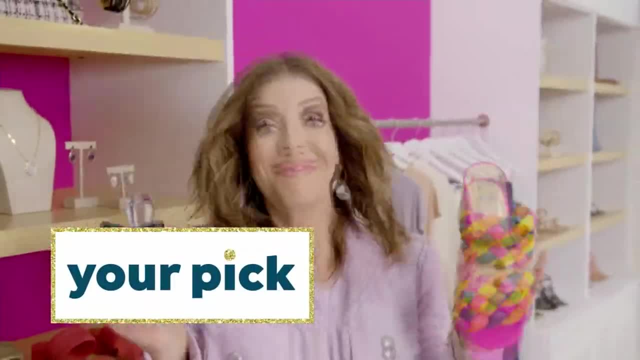 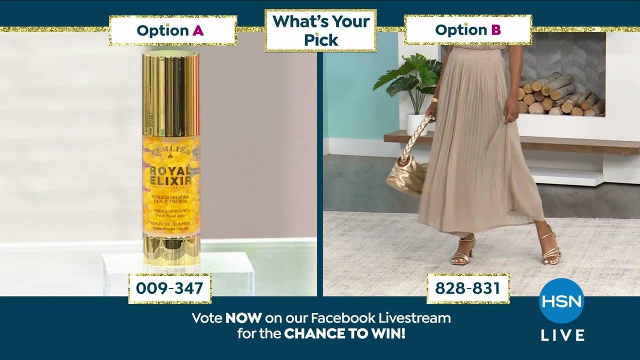 a two pack. that would be $70.. $70 and you get two for $36.95.. That is our best value of the day. Keep your orders coming on that one, because we are getting really limited. A full hour with Rhonda in about an hour. What's your pick of the show? Is it going to be Perlier or is it going to be pants? Let's see. T is going for option B, pants. Donna's going for Perlier. Tiffany's going for pants. June's going for pants. Sandy's going for Perlier. She says: I love anything. 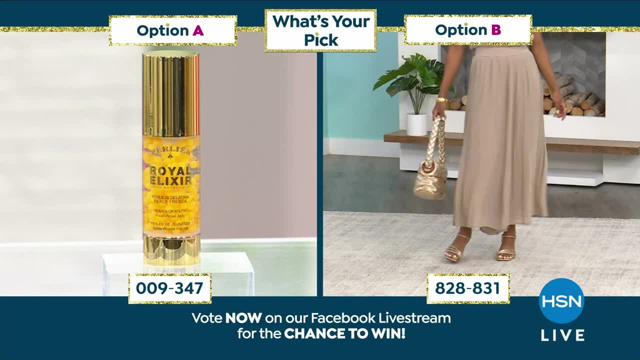 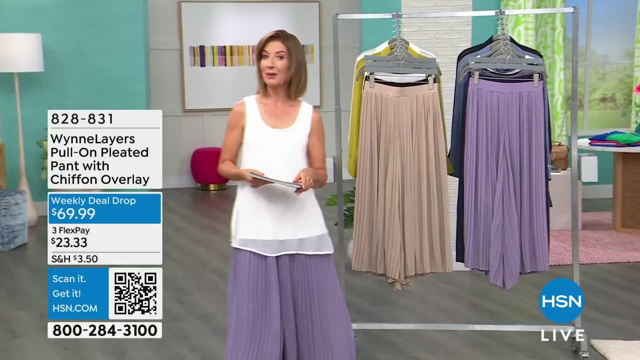 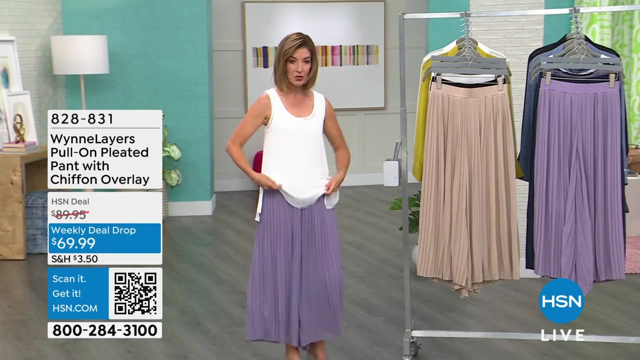 to do with skin care. Gotta maintain that youthful look. That's right. Write hashtag giveaway. We are streaming live on the HSN Facebook page and we would love to get that out for you. You can see the item numbers there and place your comment. You'll be automatically entered to win a $25 gift card. We're going to give away at the end of the show, but we have to talk about the pants Now. I had the wonderful opportunity to launch these pants back in May. 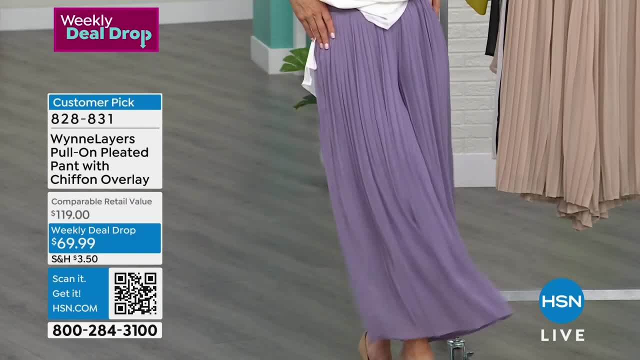 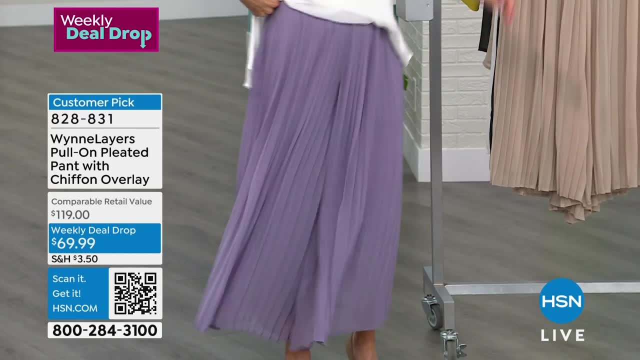 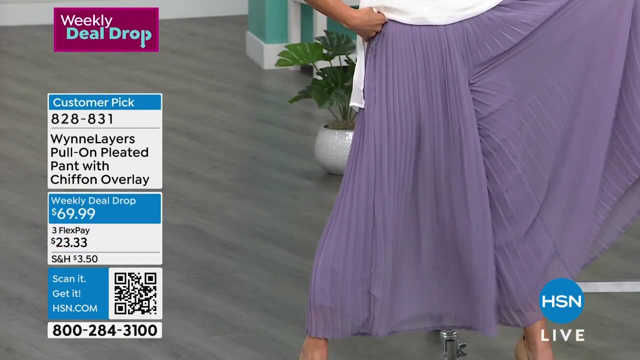 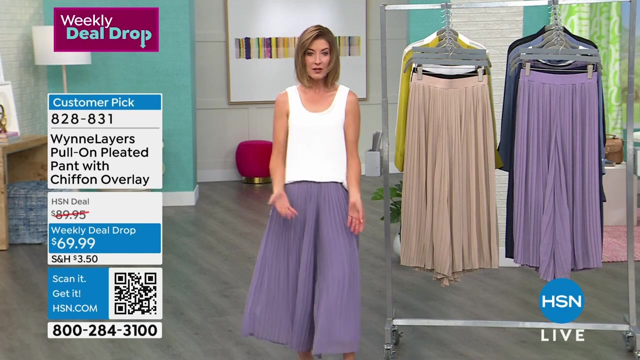 of last year. They sold out in one day. They are the beautiful pull on pleated pant with the chiffon overlay. I know it looks like a skirt. So you have all the beauty, all the elegance of a skirt but you have the convenience of a pant. Imagine that. And then look at those beautiful micro pleats that give you sort of a very kind of elongated, very sort of tall and glamorous and, I think, very Grecian look. This is 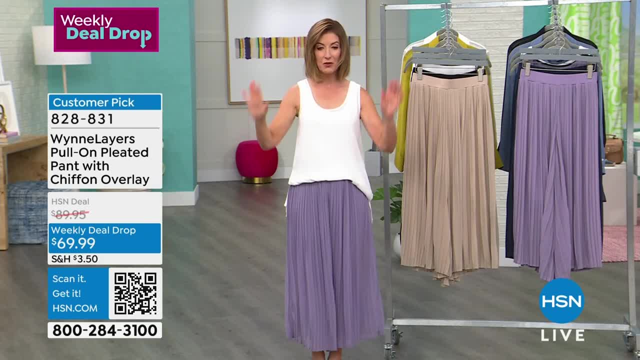 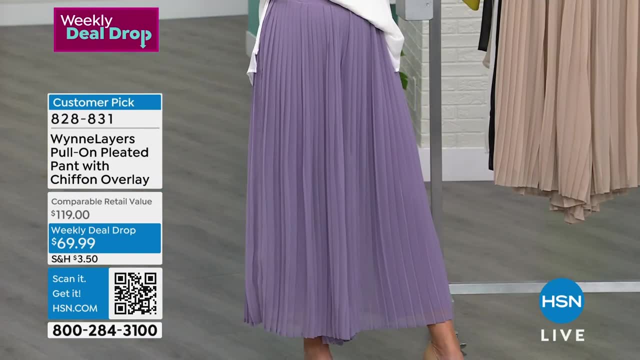 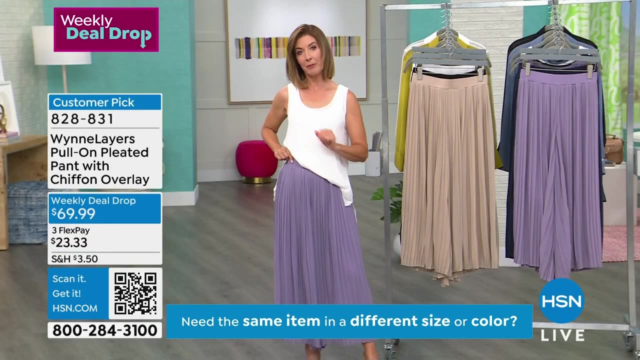 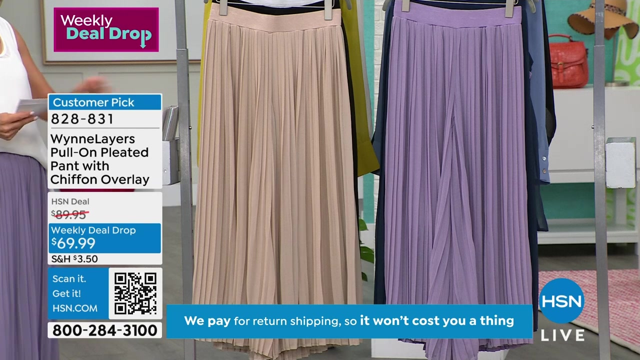 what we've done for our weekly deal drop. We're dropping it here tonight. You're the first to see it. We are bringing in new colors which you're going to love. We're also introducing a petite length for the very first time. This was such a huge customer pick. I was reading all your reviews. There was only one thing you didn't like about it: You wanted the petite length. So now we've got that for you. So let me walk you through the quick colors and sizes and we can get this out to you, because I know the colors and sizes are going to go very, very fast for you. 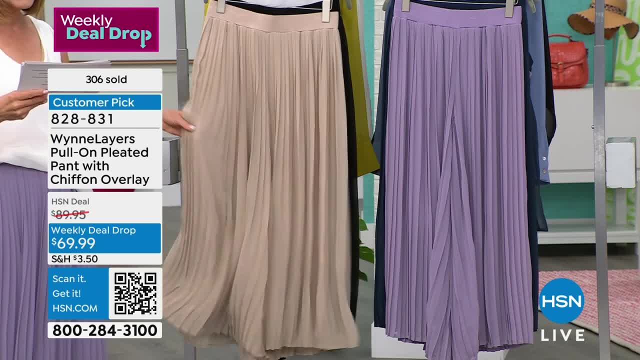 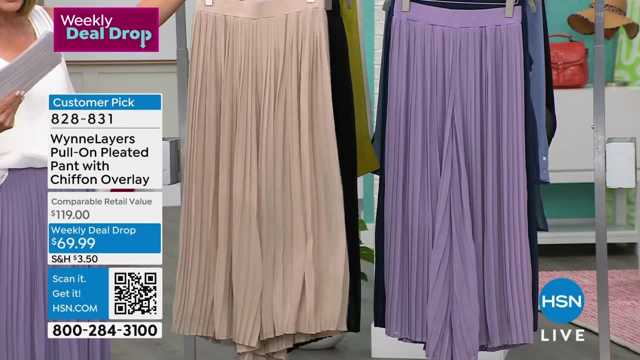 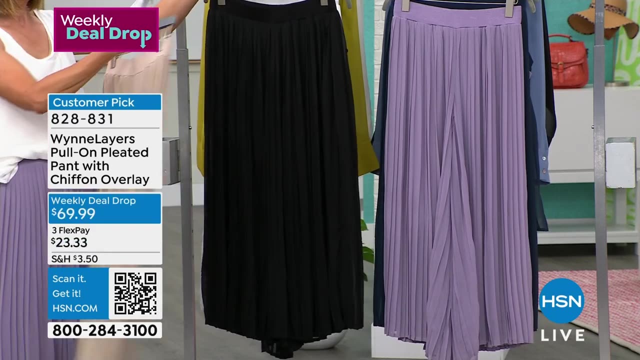 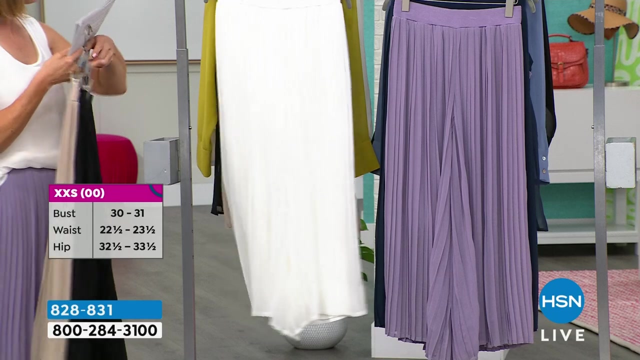 For all of our Marla Wynn fans. or if you've just been looking for the perfect summer pant- dressy, casual- you've got everything you could possibly imagine. This is called our linen color, which is so stunning. We've got a great black. Do you have a dressy pair of black pants? We're calling it sand, Okay, All right. And then we have white, which one is we're calling that cloud in the Marla Wynn collection. Now we have 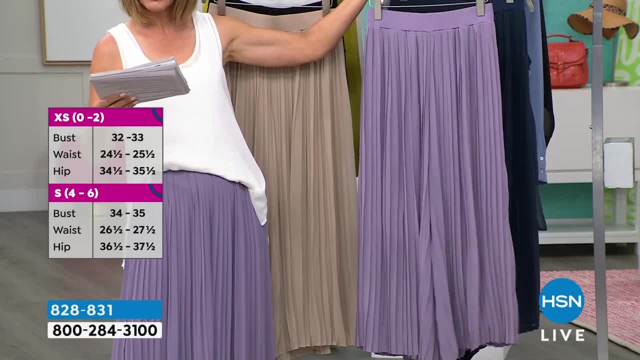 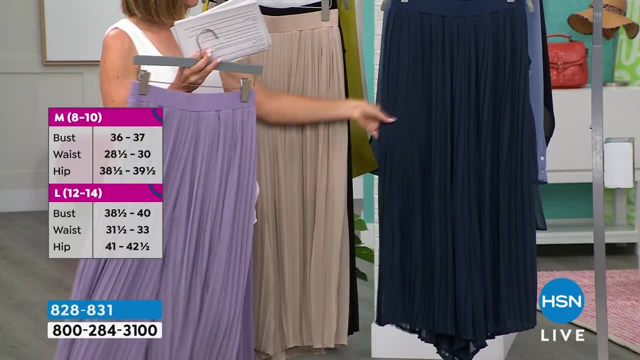 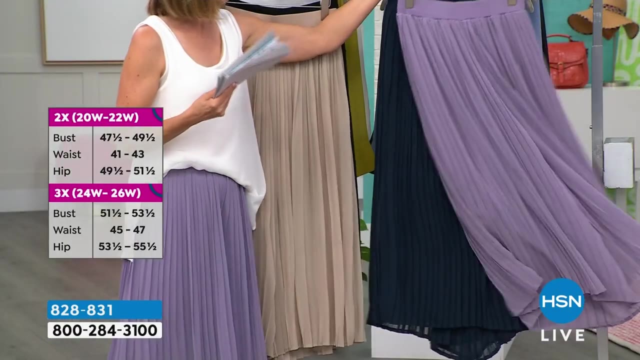 have this color, which I believe we're calling orchid. Okay, We might have a a color category challenge going on. I looked online at the color, so I'm not sure what you guys have: midnight blue. So these are our colors, And then now we have them in petite, which is 21 and a. 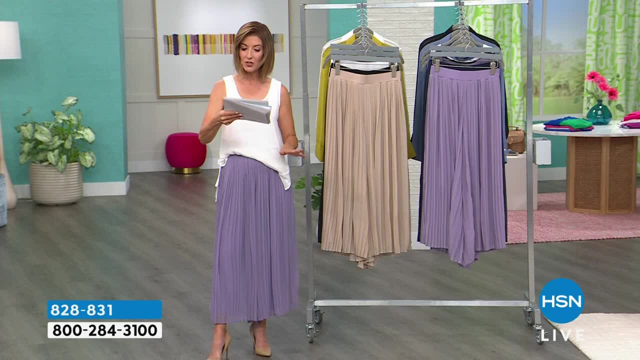 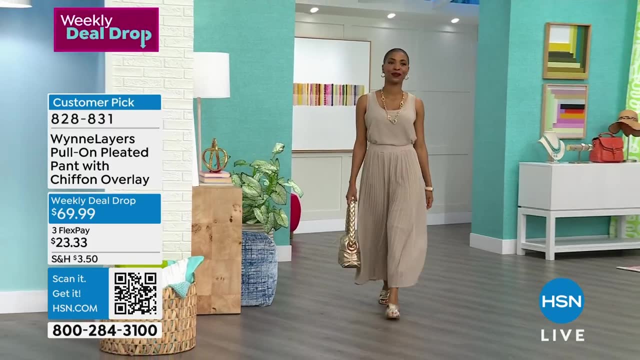 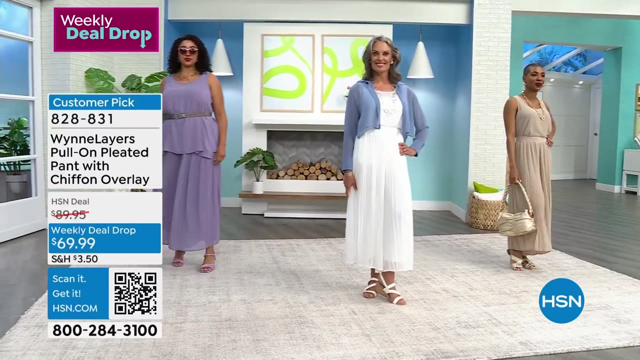 half inches in length. I have them in the average length. That's 25 inches in length, And we have a huge discount. This is $60 off the regular retail price. Come on out, Amy West, stepping in for the amazing and talented Marla Wynn. We've loved Marla Wynn's collection here for 15 years. 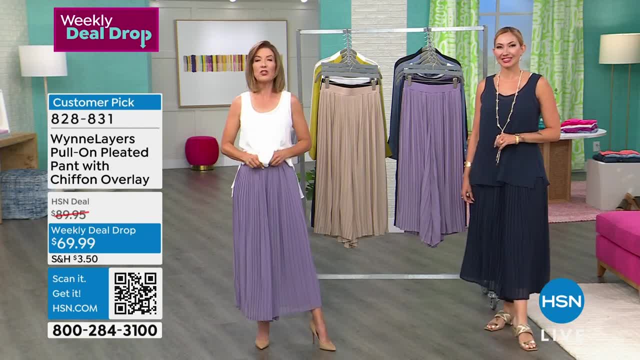 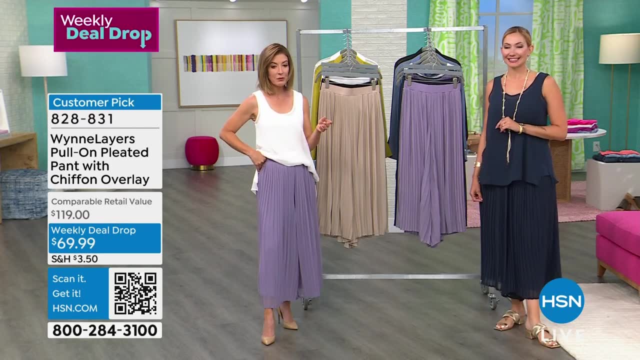 at HSN And- and I knew the minute that she came out with these pants- I said: Marla, I think you have discovered the perfect pant for everyone, And we- we were so busy We have not been able to show these to you in about a year. 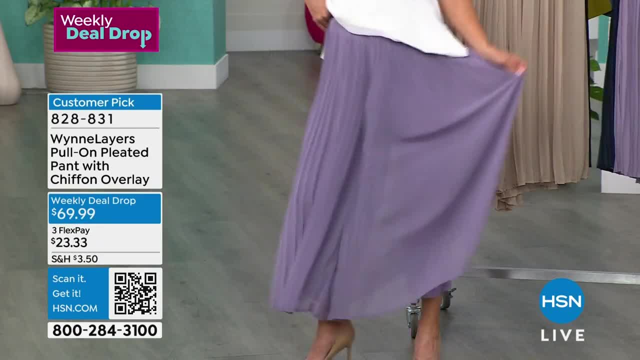 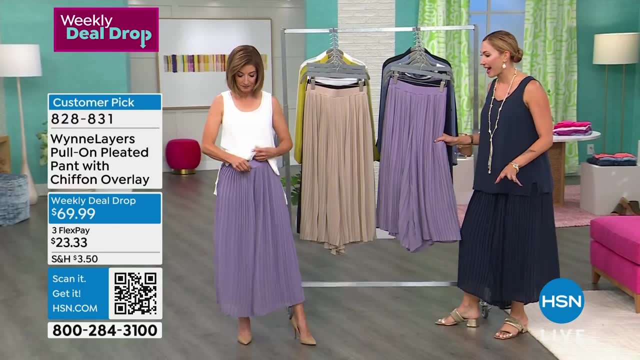 I'm so glad You're the first to see it. So, Amy, tell us all about it. We have an incredible price. This is $60 off today. So excited that we've gotten these back. I love that we have new colors, Sarah. 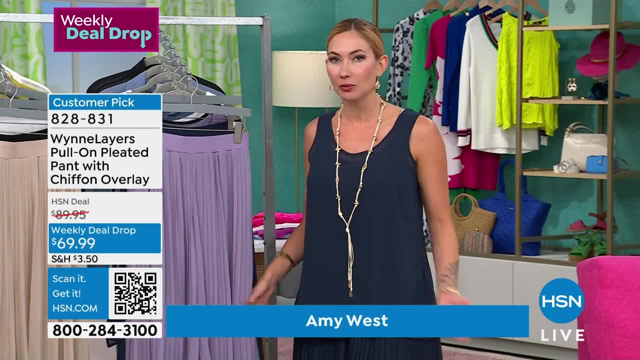 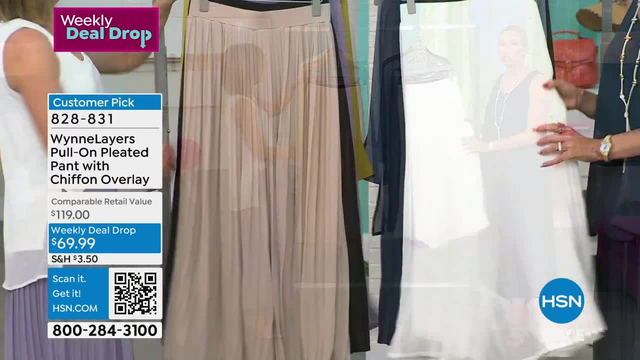 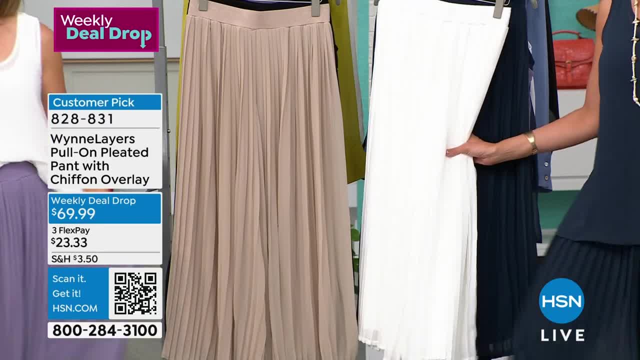 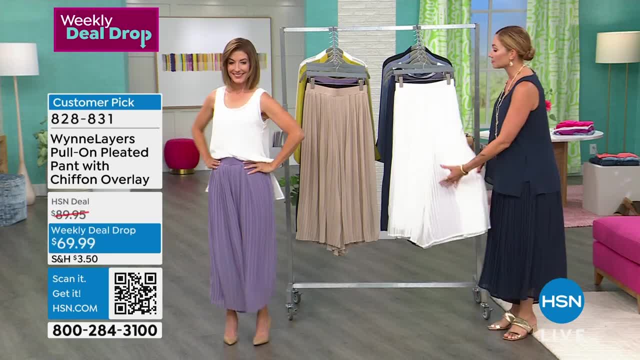 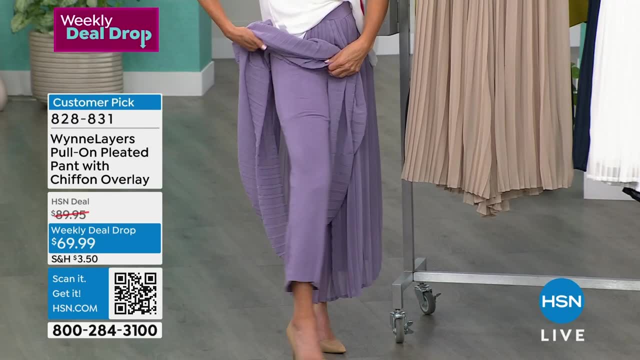 So you don't have to worry about any like wardrobe malfunctions If it happens to be breezy maybe, a beach wedding maybe. if you're out- And one of the things that I love about it that you're not there- you go. Oh, that's a great shot. I wanted to show off that really. 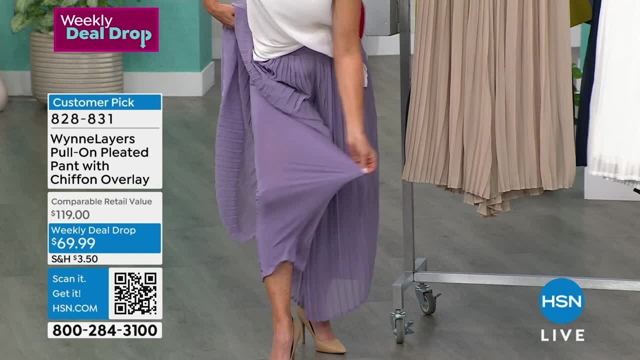 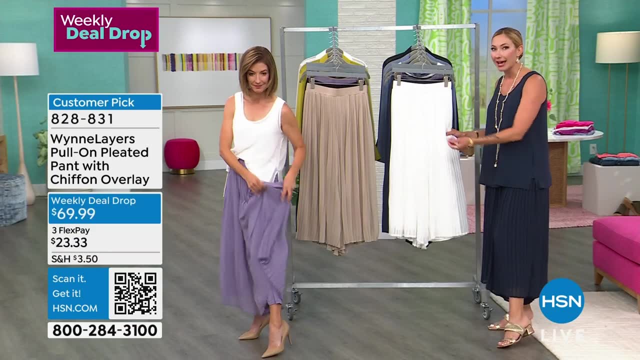 great Jersey knit pant underneath, So everything is completely opaque. There's no see-through, no grin through. You don't have to worry about finding a slip for underneath your skirt, because we have these great Jersey knit pants underneath. And then, of course, these are actual. 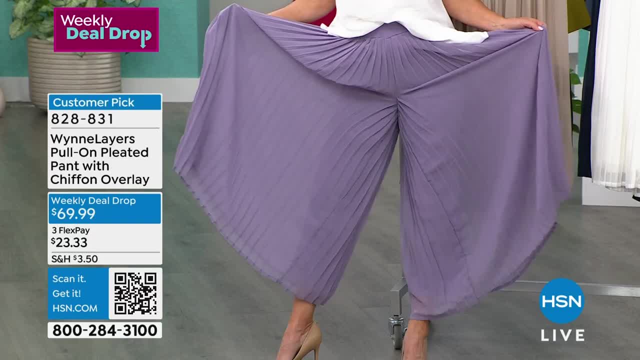 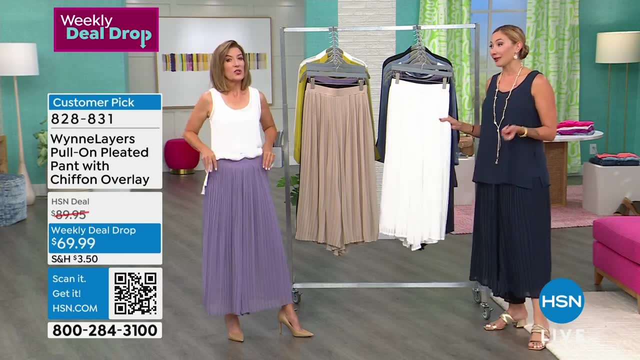 pants, So it gives you that look, but then with the confidence of having pants, I love that we have that nice wide waistband and it really is fun to style. You can make this very dressy. So many pretty ways to wear this. You can wear like a graphic tee with it and a jean jacket. 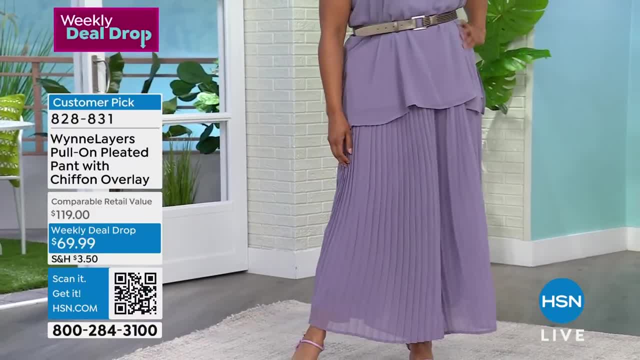 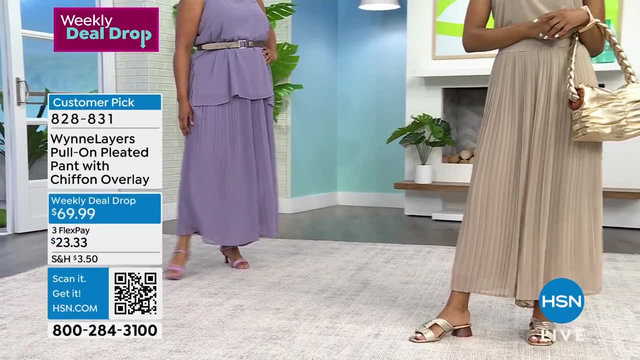 and it would be very fun as a casual look with some sneakers. Marla always loves to put in sneakers with her, her designs and with her collection, So I think this one have a lot of fun with it. It's very timeless, very elegant And, honestly, I think it travels really well. 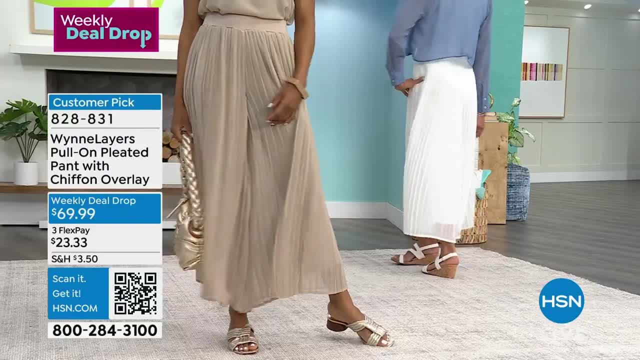 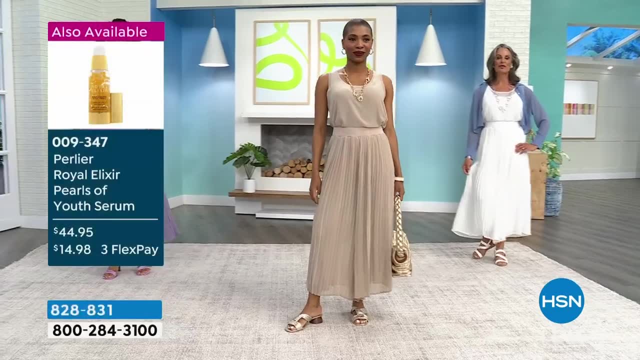 also because when I pulled mine out of my packaging I didn't even have to steam it that much. So this is something that I would take with me traveling, because the pleats- they kind of mask any kind of wrinkling. You can wash it and not worry about the pleats Major, You do not have. 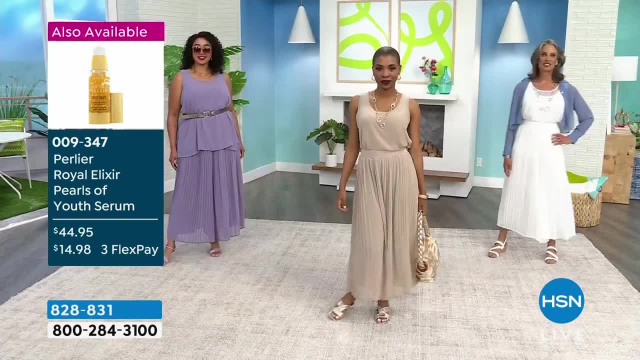 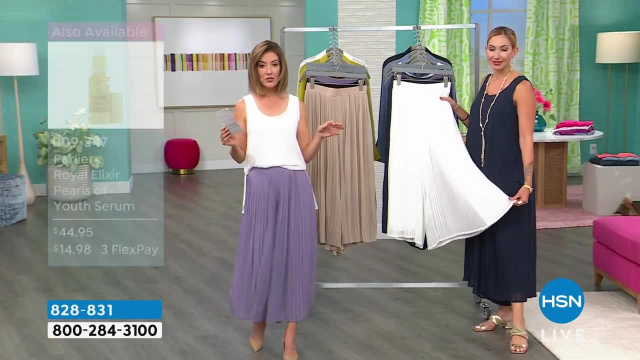 to iron these pleats at the most, just shake it out, hang it in the shower While you get ready And that's the magic machine: wash, dry them flat. First time ever in petite. first time ever in all these great colors. Okay, I think we decided that if you want the sort of 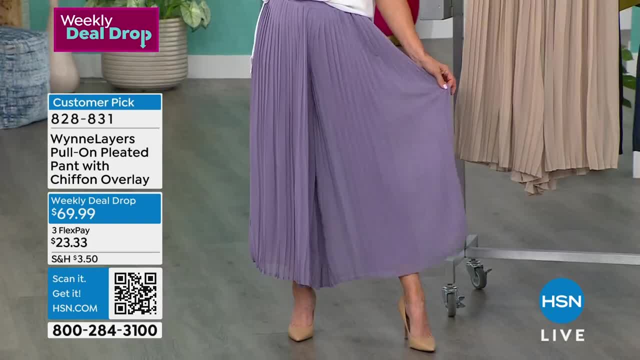 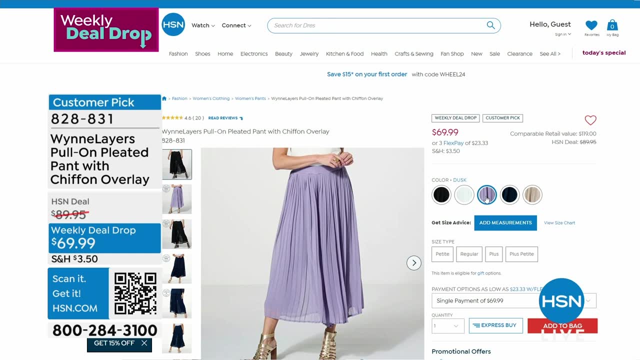 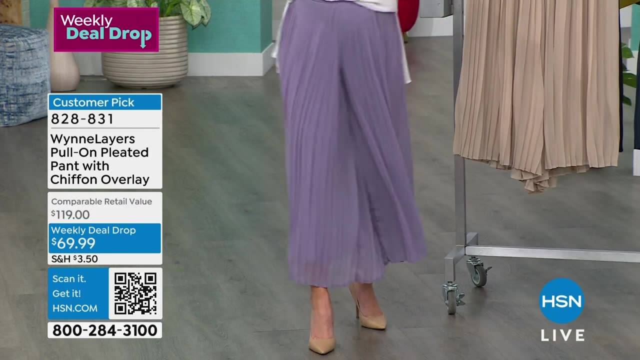 lovely purple shade. uh, it's called dusk, and I think it's called dusk online as well, So you can go ahead and shop the dusk color. It is a beautiful soft lavender with just like a hint of gray. It is so pretty, It's so original. I love that it's light. I love that it's breathable. 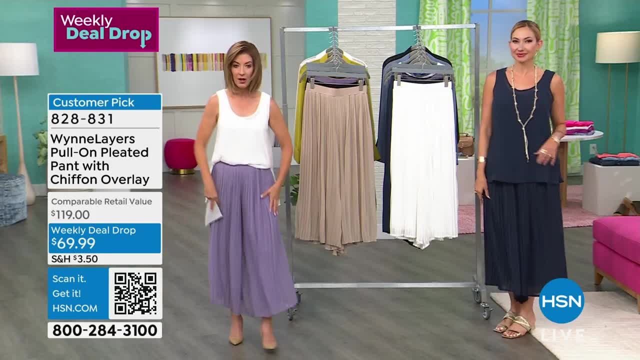 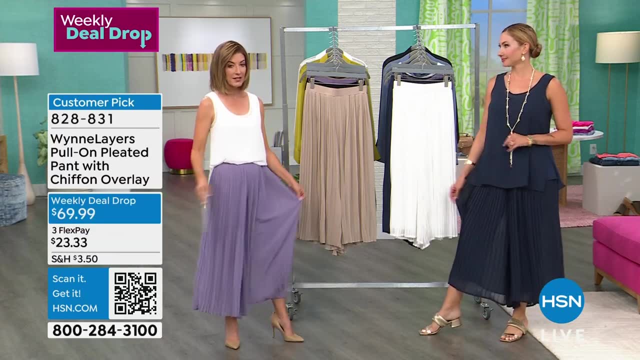 I love that. it's kind of like that effortless style You pull it on. Nothing is sort of squeezing your legs, Nothing is tight, Nothing is stiff, Nothing is heavy, Nothing is hot, but it feels like nothing's touching your leg at all. Uh, so far out of the gate, I think it's the black. 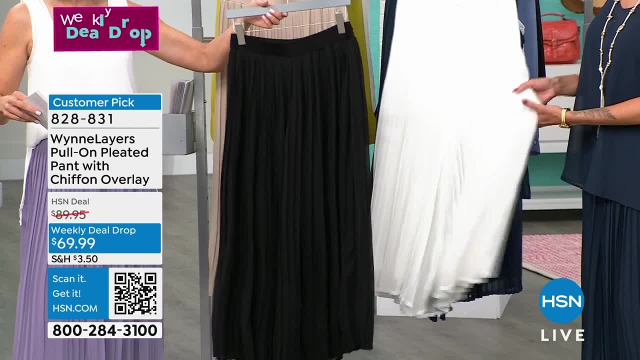 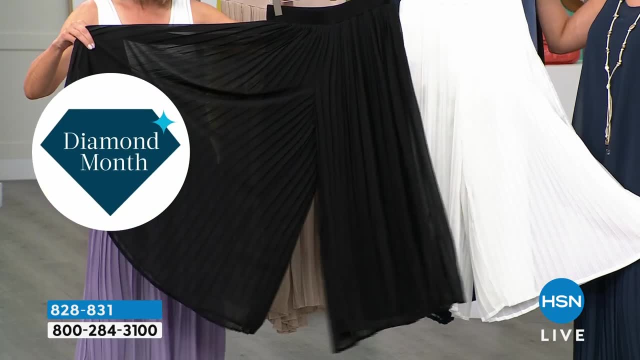 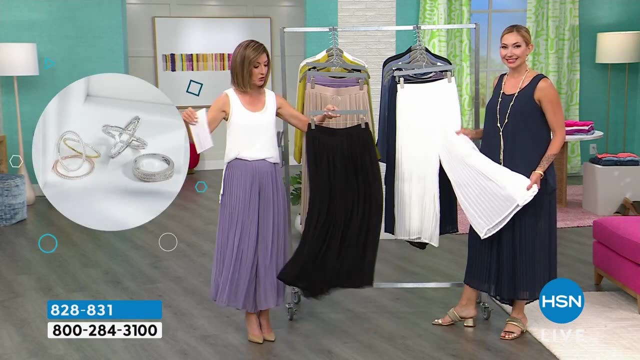 that might be, uh, one of our best sellers. I would not be surprised if black and white go very quickly. So this is black And remember, this is a pant that looks like a skirt. You get all the illusion. You get that pretty kind of fluid, gorgeous drape. but then the practicality. 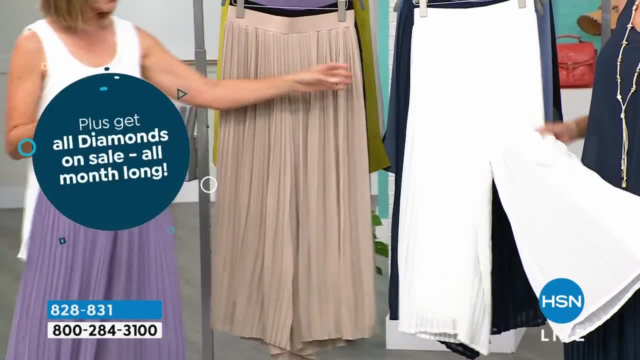 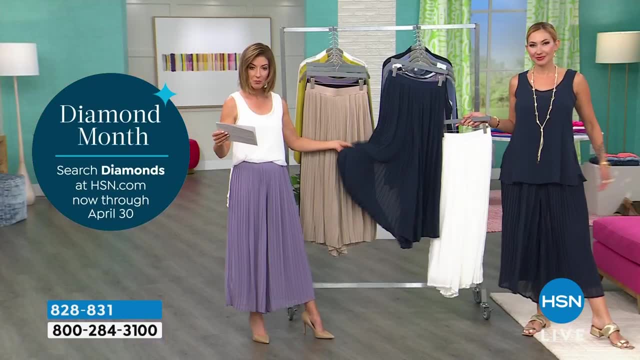 of a pant which I think you're really going to love. uh, after the black, it's the midnight blue that they're loving, And you can see the midnight blue on Amy. It's a nice deep Navy, and look at how pretty that colors. These are saturated, And then even the lining on the inner pant, cause it's a. 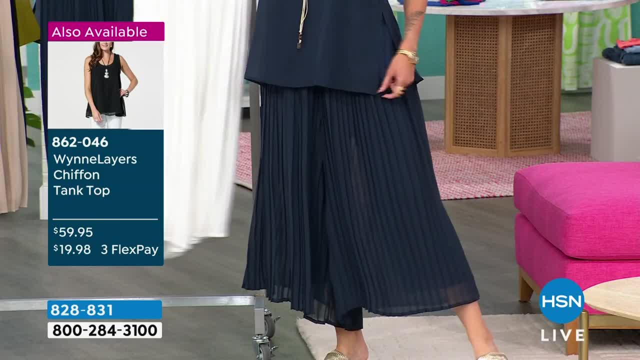 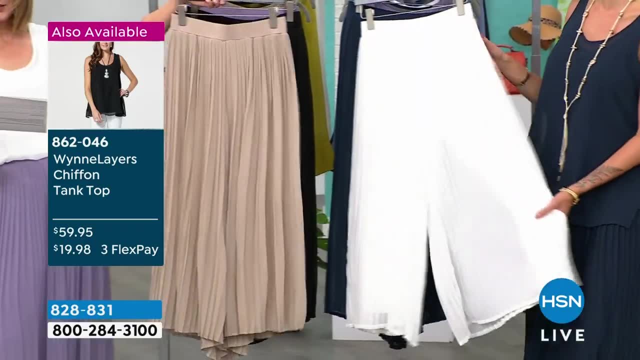 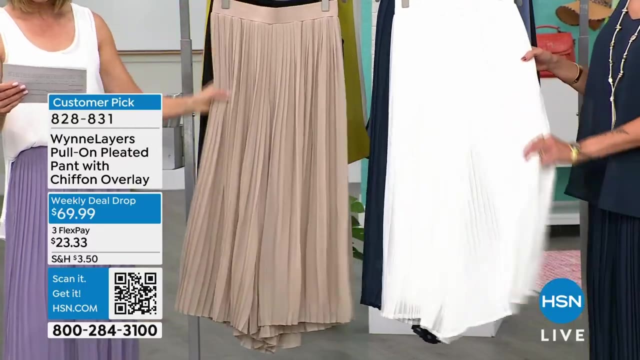 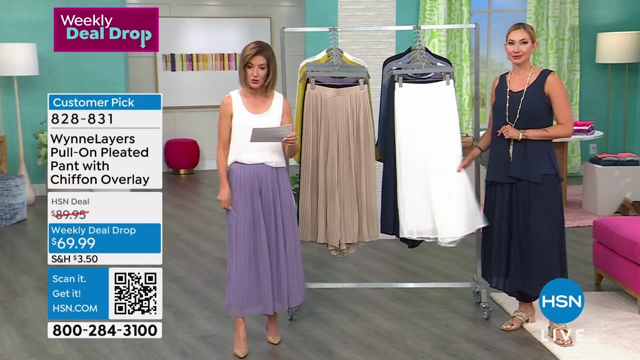 true kind of Jersey knit pant. underneath is fully lined. The white is so elegant. We're calling that cloud And then our. are we calling this one sand? We're calling this one sand, I believe. So here's what you should do: Jump in extra, extra small through three X. petite is a 21 and a half inch and average. 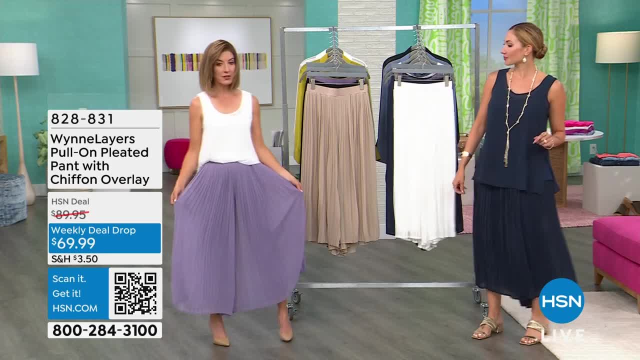 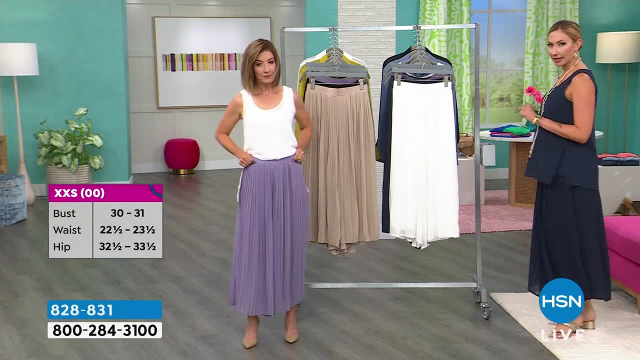 is 25.. So let's talk about what everyone's wearing. I'm wearing the average at the 25 and a half in seam. I am five, six, What are you wearing? I'm actually wearing the average also, And I am five. 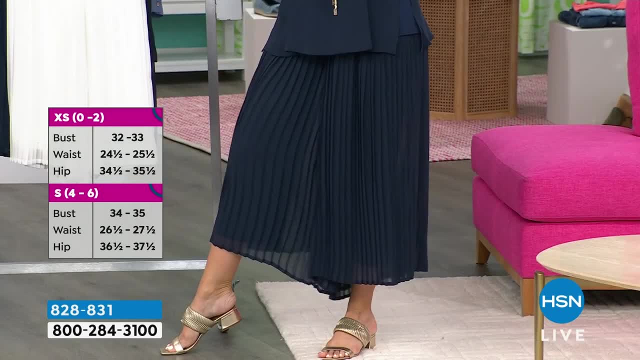 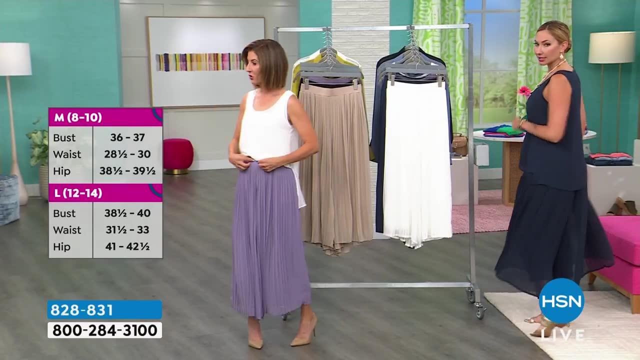 nine, I'm an immediate And I usually range between like a six, eight, 10,, depending on the day and the pant. But with Marla I'm always mediums in the pants. So okay, And I'm wearing extra small. Let's see how our 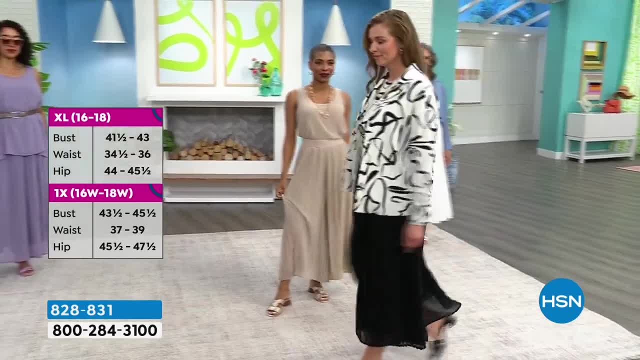 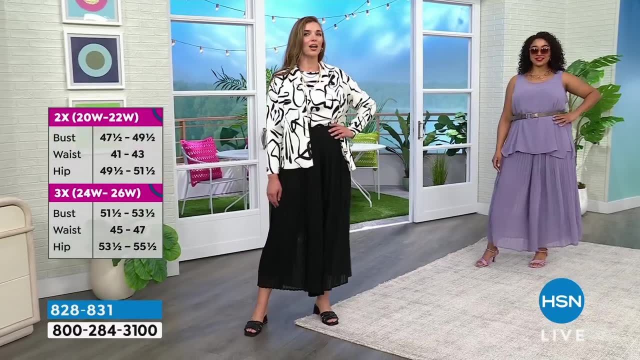 girls are all decked out for summer. All right, Let's start with Diagmara. She's doing the model walk, which means like: look at me, Look how cute that is. Are you in the medium? She's in the large. 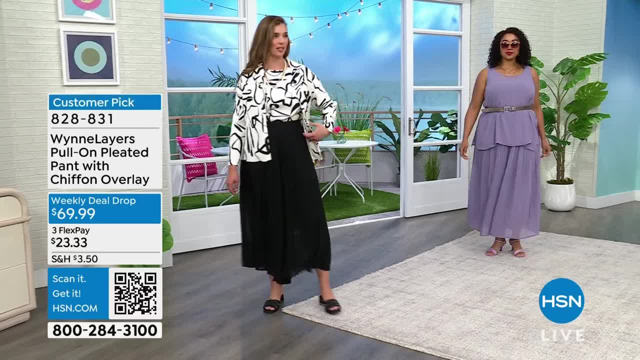 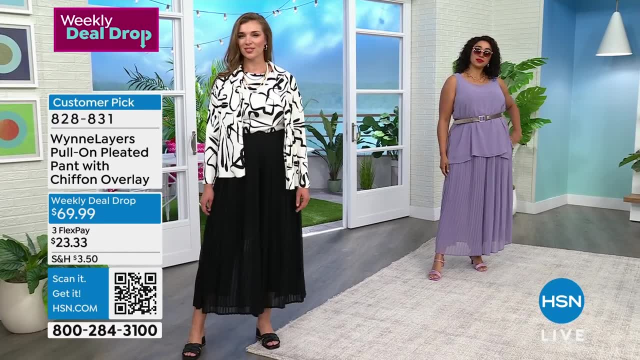 today. Okay, So just to show you- and you are- how tall five five, nine, and she's got the average length on. In fact, I don't think we have any petite models here tonight, So you can imagine it would just be. 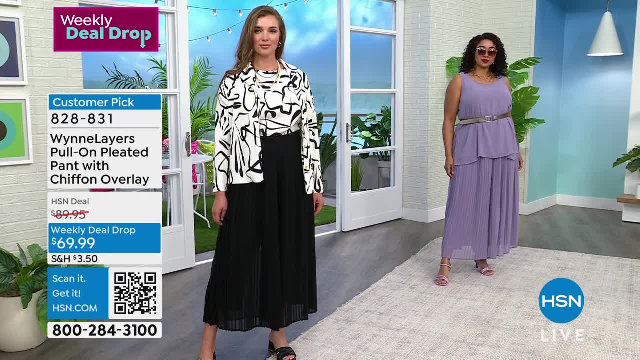 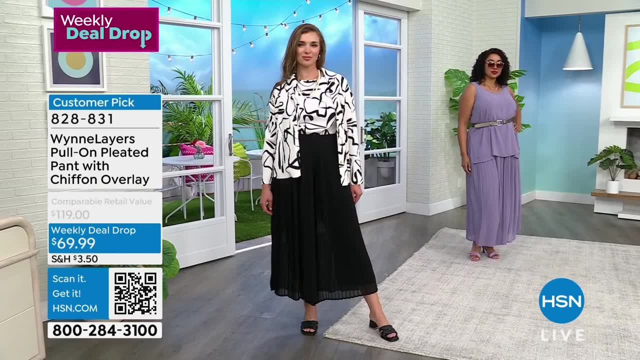 about four inches shorter. if you want the petite length, Kenya, are you in the one X, Kenya's in the one X, and we have the matching tank available So you can start putting together the quintessential Marla Wynn summer outfit right? Yes, absolutely, And if you're new to Marla's collection, know that. 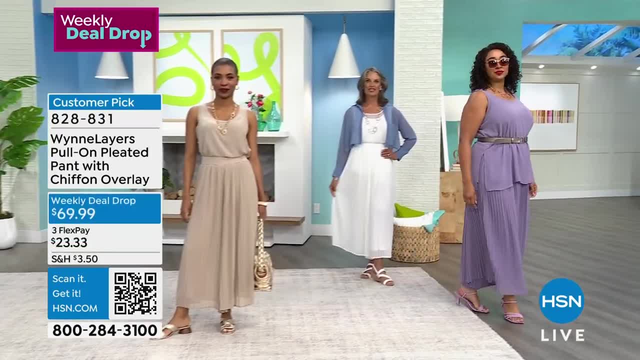 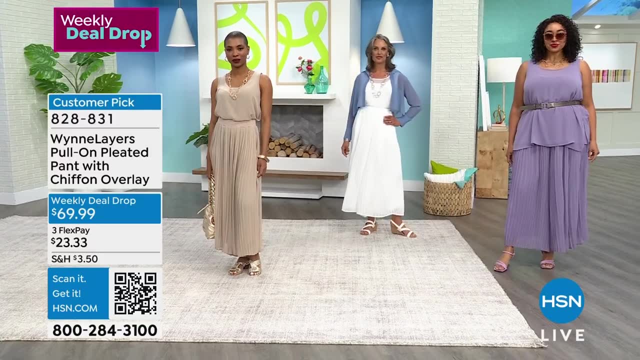 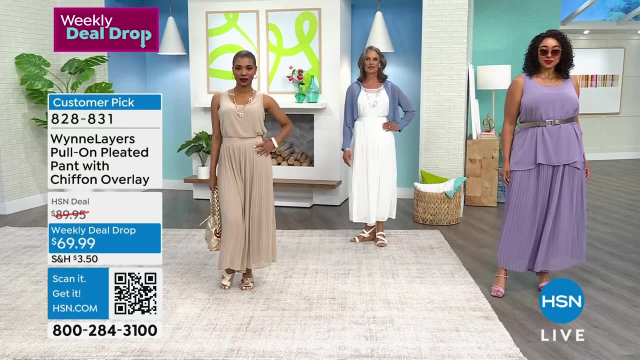 she designs seasonally and, you know, multi-seasonally, in many of the same shades. So some of her staples, uh color palette, will remain season by season, And then she brings new, new colors in each season. So they're all designed to pair well together. So as you build your wardrobe of Marla's pieces, 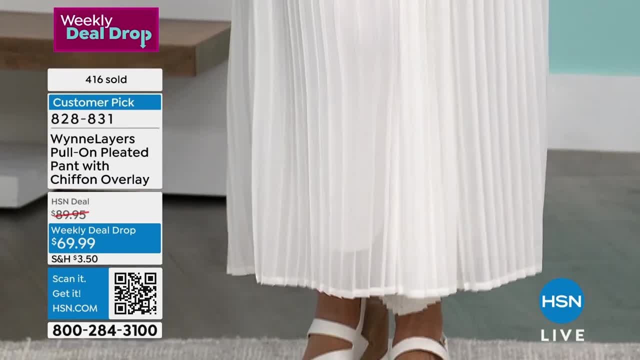 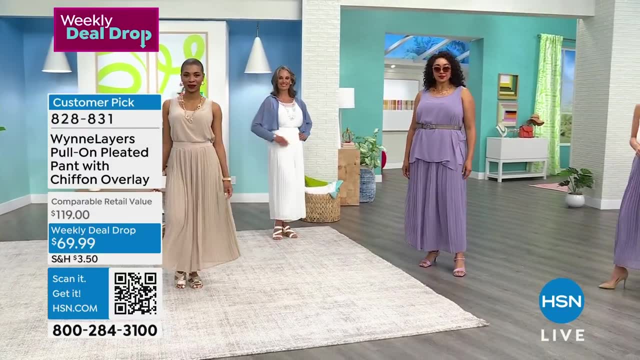 they will pair back together. She likes to call them girl animals for adults, because the colors are all dyed to match and they really do pair very well together. But she's also designed the beautiful tank which we're going to see in a moment, which also pairs perfectly with this. 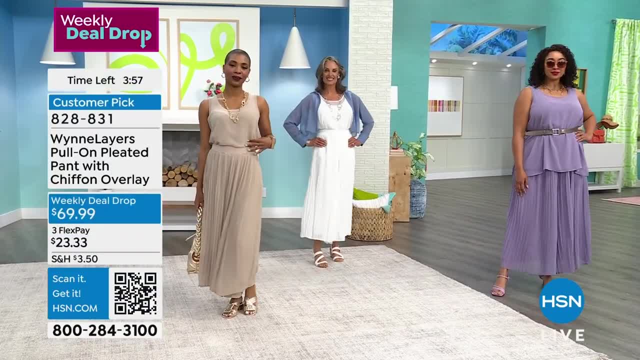 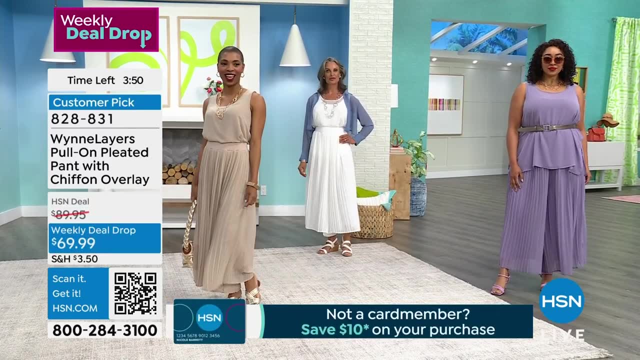 because it is that same chiffon top With that underneath, the Jersey knit underneath. These are so beautiful. Now, Shay is in that beautiful sand color. Uh, Shay, are you in the extra small? She's in the extra small and she's. 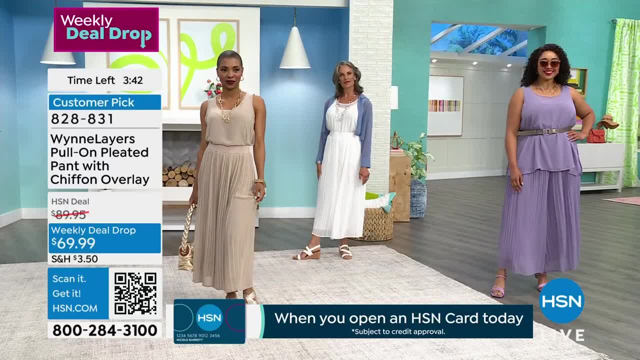 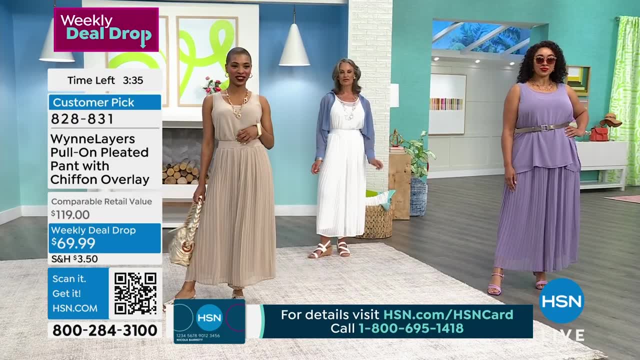 also wearing the average length. Now, how tall are you, Shay? She's five five. but I'll tell you what it's. it's not a full length pant. It's supposed to sort of just give you a little bit of a crop So you can wear all your summer sandals. You don't want it sort of dragging on. 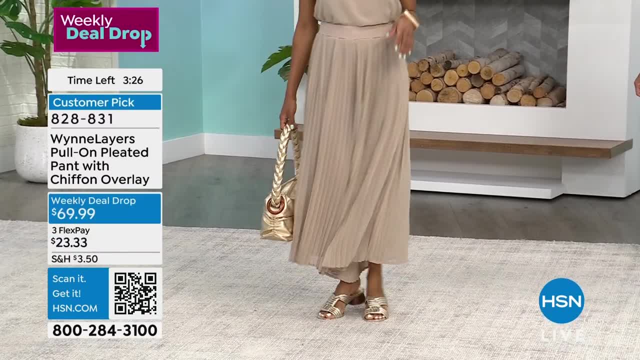 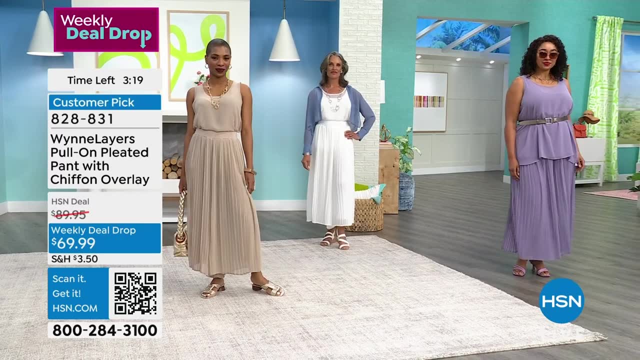 the ground or on the beach or on the sand. So you can wear it at the average length. but if you're really petite, go ahead and go for that petite length. And then we've got Diana. She's wearing it in. uh, the white is just so. 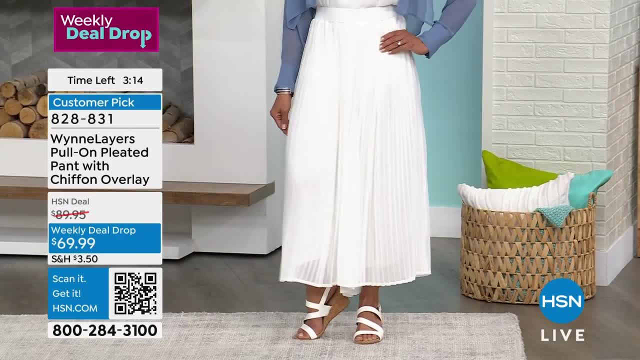 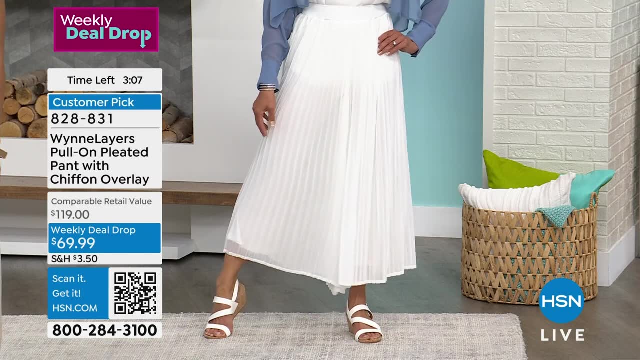 dreamy and so fresh. Is that not what you want for every like summer vacation? Yes, You want that sort of. it always reminds me of how they dress around the Mediterranean. You know everyone's wearing white in Greece, in Italy, And we know that Marla does take a lot of inspiration from. 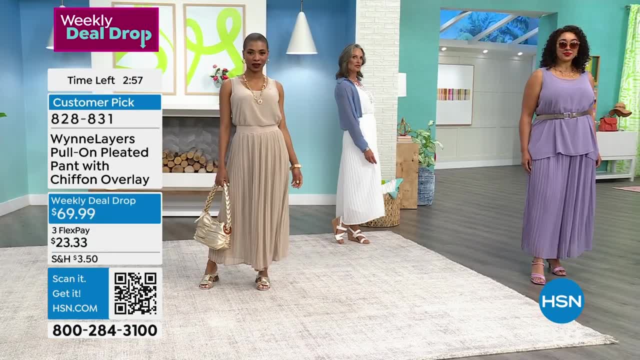 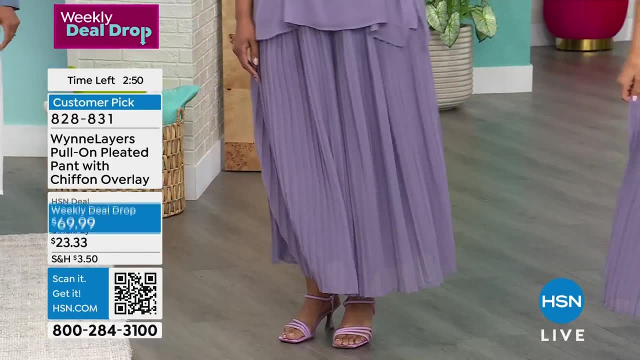 her travels as well as her time while she lived in Paris, So she's wearing a lot of inspiration from Paris. So, if you're new to Marla's story, she actually lived in Europe for over 20 years and she takes a lot of inspiration from the Parisian style And it's just very cosmopolitan. 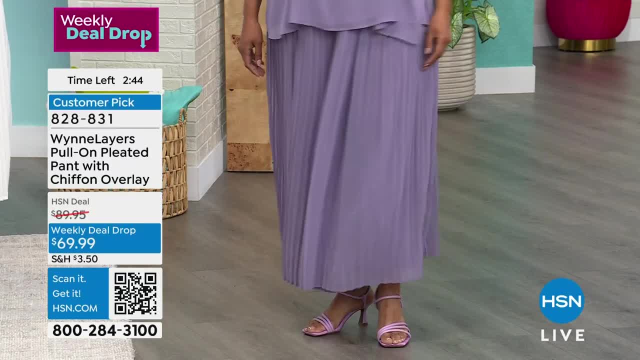 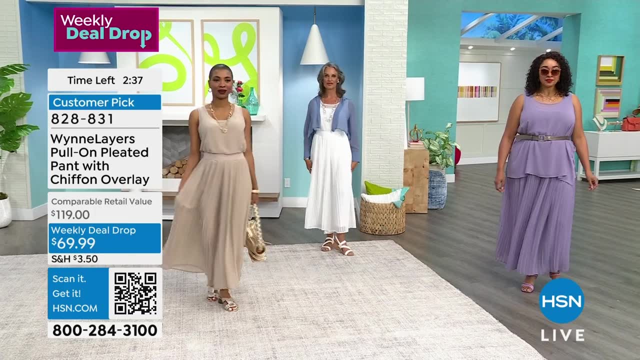 in all of her efforts, with her designs, with this collection. So you're going to see a lot of influences from that And really she just finds she has a way of creating these classic, timeless looks that make a statement but that also are super comfortable. They are like wearing. 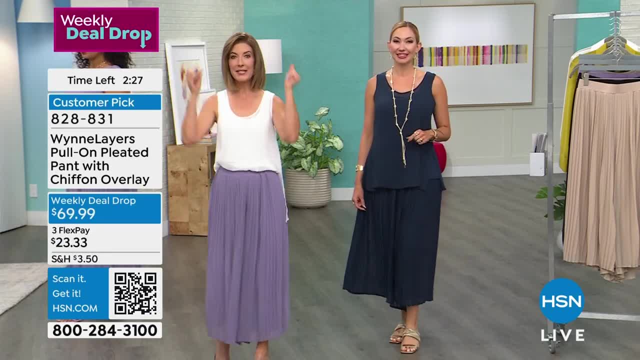 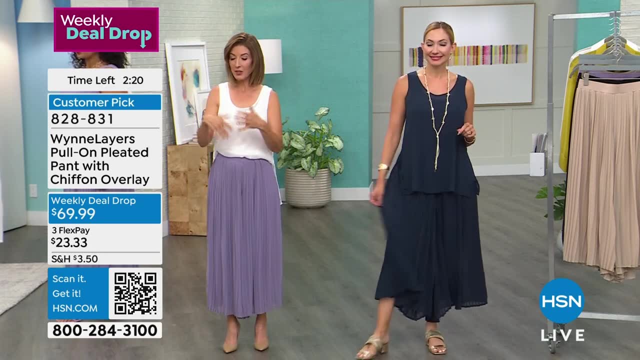 hardly anything at all. If you're someone in the summer, you feel like everything is getting really hot, Everything is getting really humid. You can't bear to put on any clothes. I know who you are. You're, you're living in, you know, maybe the middle of New York. 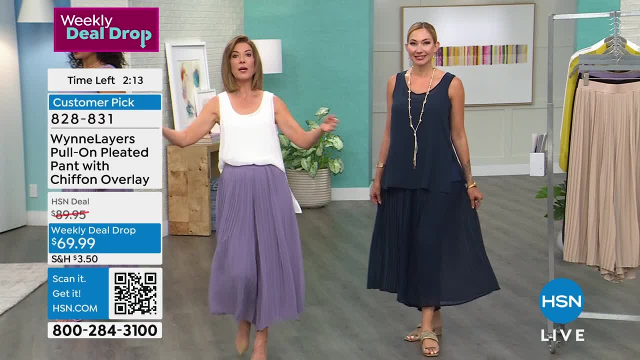 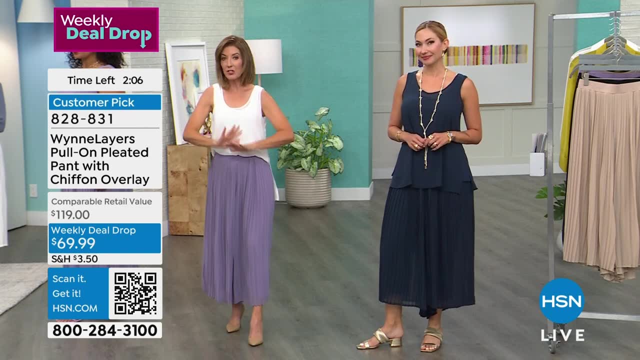 City, but you still need something that covers right. You still need something for that wedding. You still need something for that graduation. Maybe you don't want to be head to toe in a dress. It feels a little too fussy. This is the perfect little sweet spot. It's like that happy. 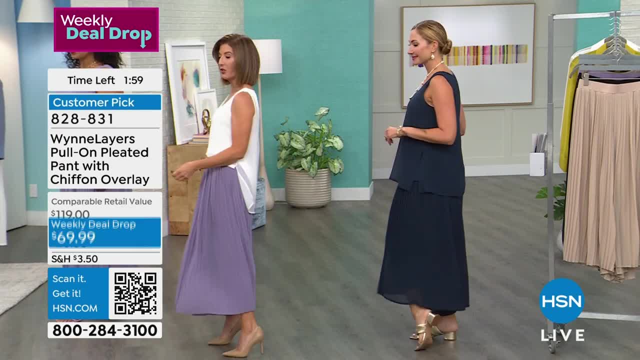 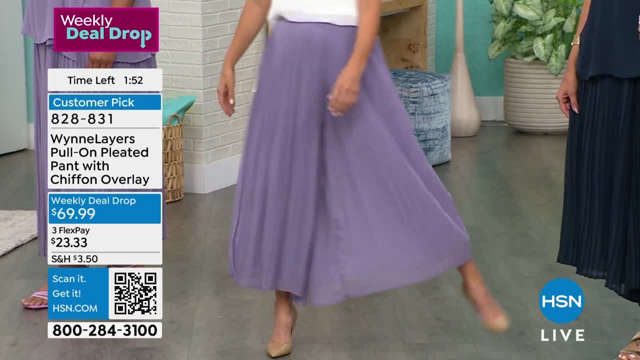 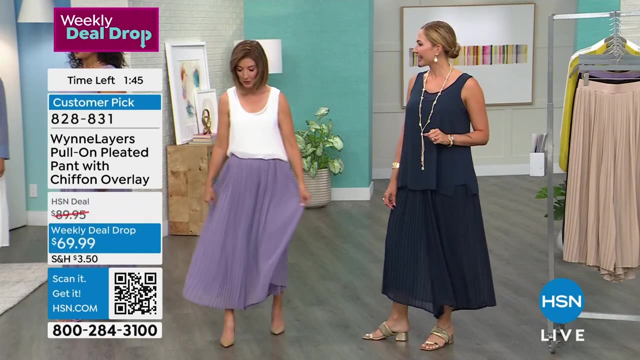 little space in the middle where, oh, it looks like I'm wearing a skirt. No one would actually know that I am wearing a pant unless I decided to get on a horse or a motorcycle or started climbing stairs. You know, maybe when you're sightseeing and you're checking out all the 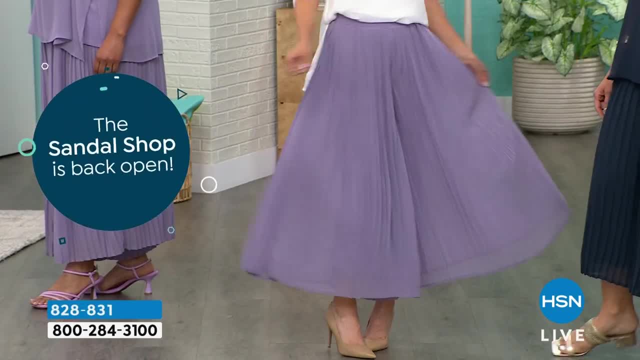 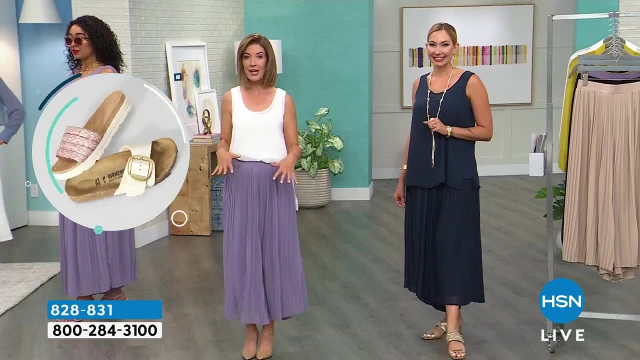 temples and the palaces and all the old forts and all the old castles. I mean something like this you would just live in. It could be as elegant as you want it to be, but you could also just throw on your tennies and just grab your cute little t-shirt, a fun little summer hat You're. 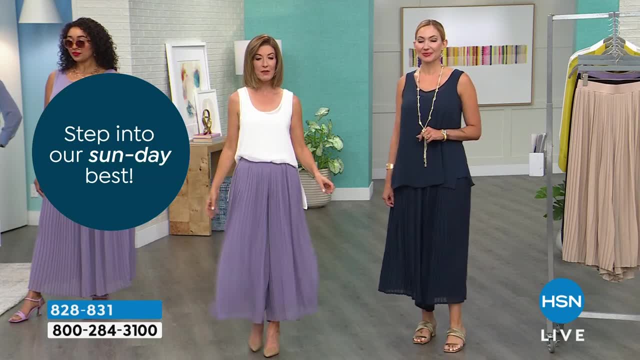 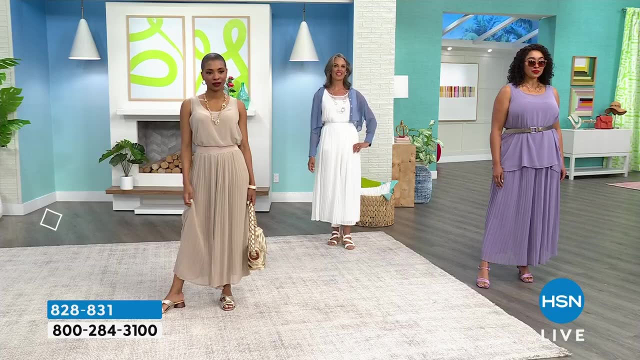 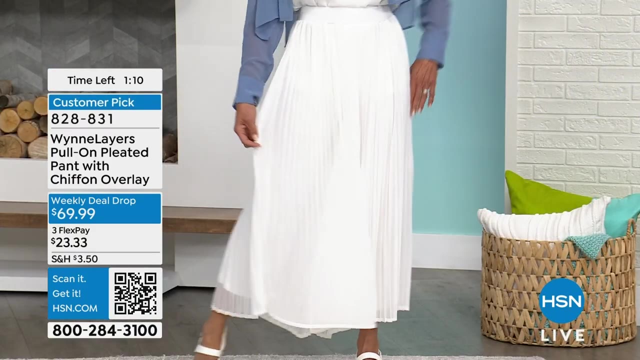 going to love it. It's not as fancy, it's more of a little bit of a tie-dye that just goes on the door And this is perfect for your beach or your pool or your little cruise vacation. It is machine washable. I would not be surprised if colors and sizes go very quickly. We've been 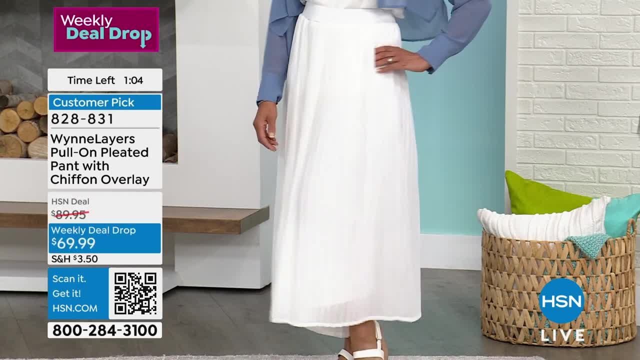 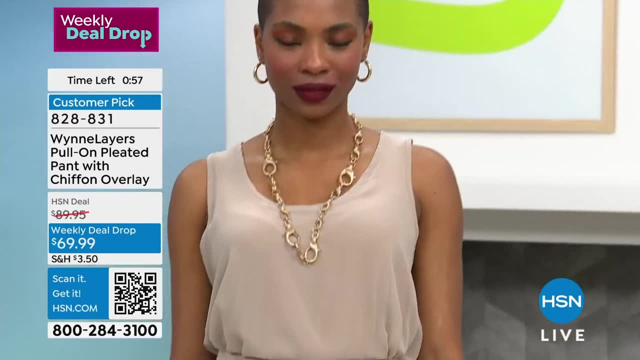 waiting a year to get this back in stock. You're the very first to see it. White, That beautiful dusk, is the purple, We've got the sand, We've got the black And we've got the sort of midnight blue and we have the matching tank. I will give you that item number as well. It's 862046862080. 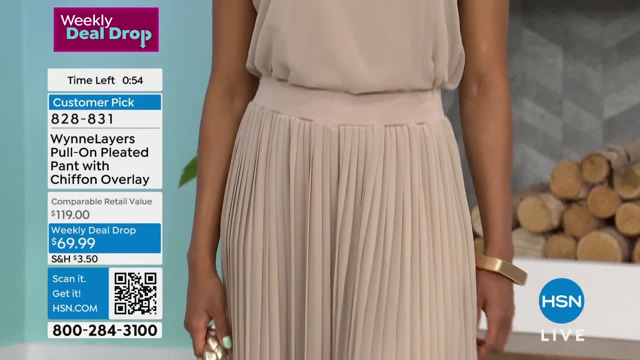 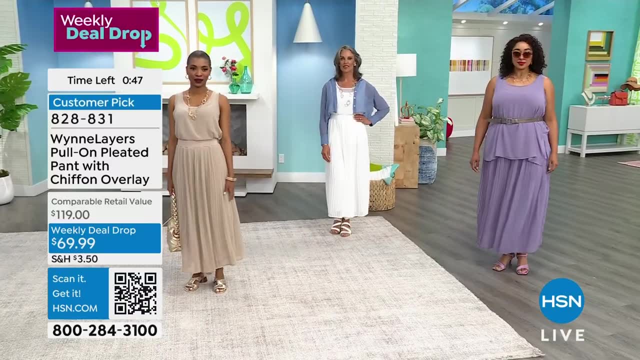 2046.. We'll talk about the matching tank in a moment, but I want you to have the perfect dress. I almost want to call it a dress, but it really is the perfect pant for summer. It really is, and I loved how you were describing like all the places you can wear them. I have a trip to. 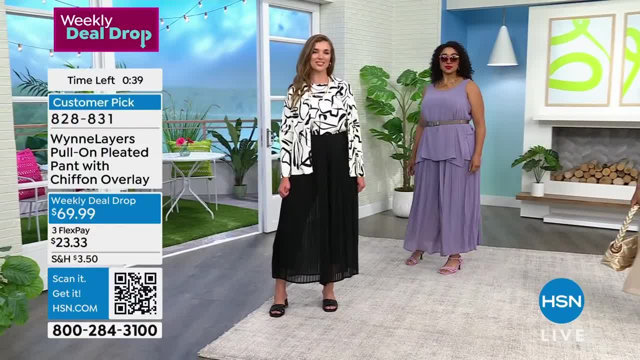 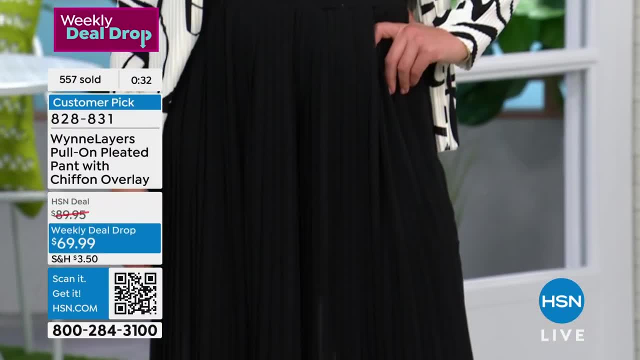 Italy this summer. We're planning with our kids and I'm already thinking about my wardrobe. What am I going to be wearing? And this is really that perfect piece, because you can have a lot of versatility in the way that you style it and it just looks so elegant, no matter which way you 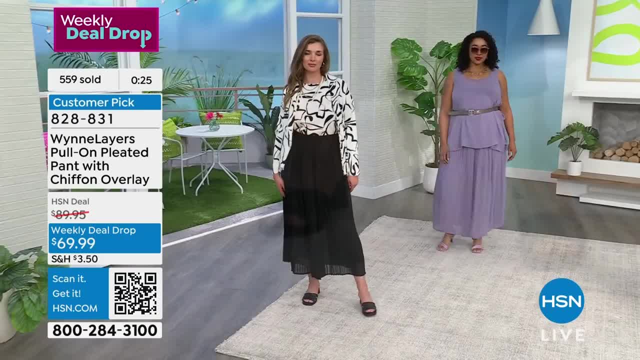 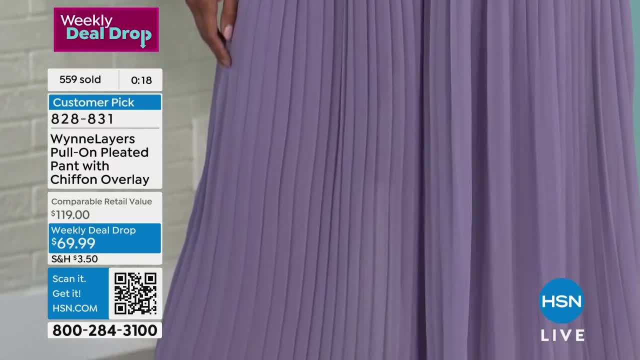 style it. Plus, as you mentioned, you can care for this in your home. You don't have to dry clean it, and usually when you see something this elegant and especially pleated like this, you would think, oh, I can never put this in a washing machine, but you absolutely can Hang it to dry. 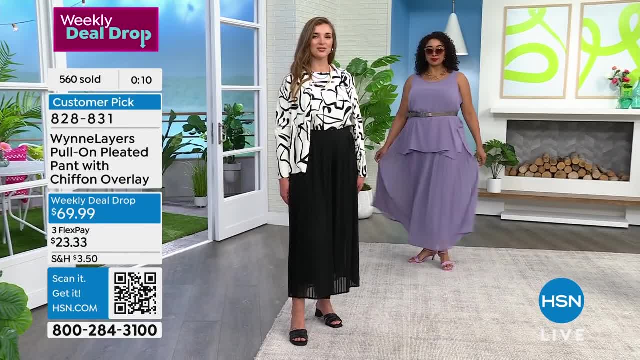 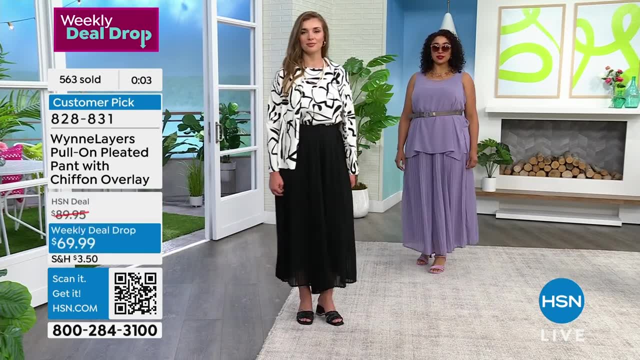 Don't actually put it in your dryer. You want to hang it to dry, Lay flat to dry. but yes, so much versatility, so beautiful. You have to read the reviews on this piece. People are beside themselves. People love this. You're loving black, You're loving the dusk. Those are the 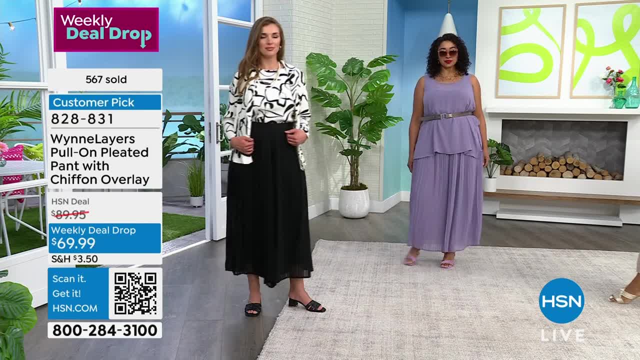 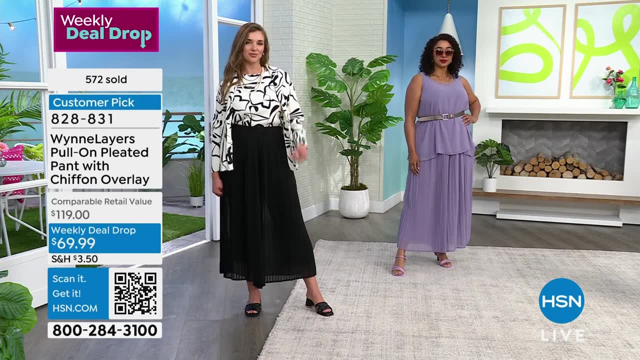 first out of the gate. A lot of you said washes beautifully, very comfortable, very pretty, very timeless. You love that. it's very upscale and classy, super feminine. Also, even though these are pleats, they do not add bulk. because the pleats are so small, They're called little. 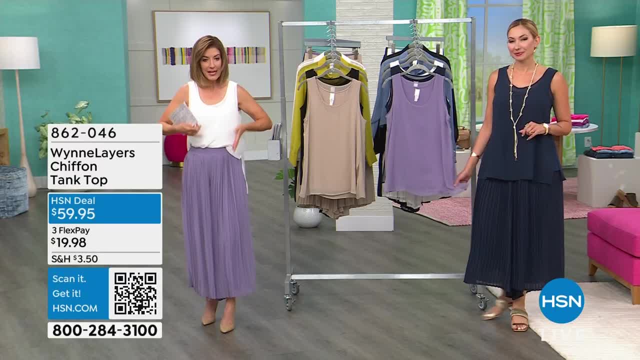 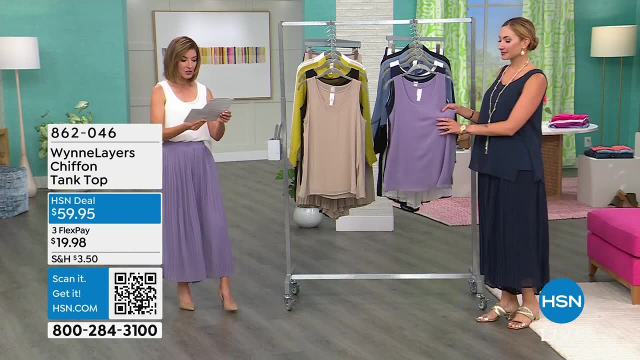 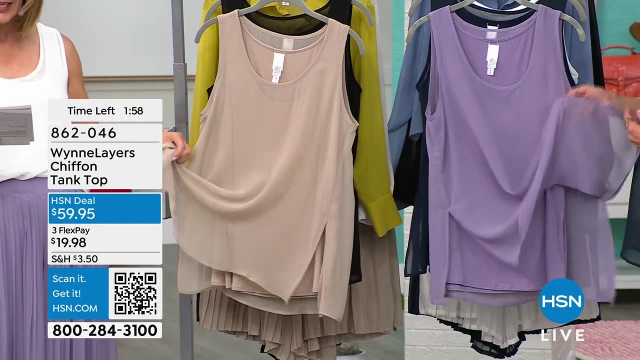 micro pleats so they actually just add movement and they actually kind of give you that linear look, that kind of column style dressing. So let's get to the tank. So let's get the tank out here. This one also has a built-in layer, so just like the pants have like a second pant built right in. 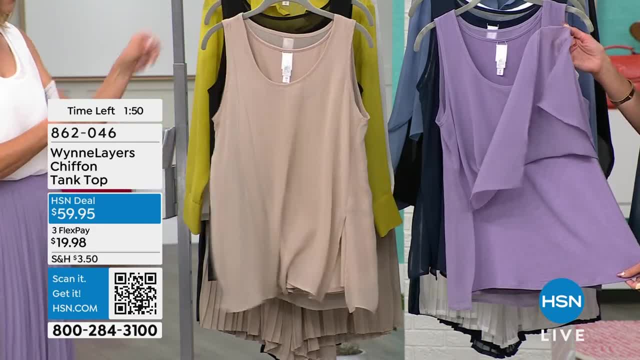 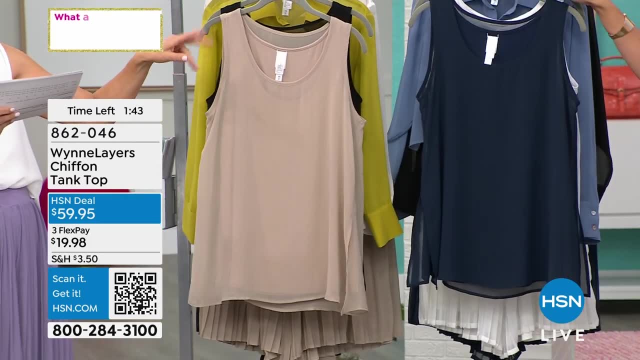 so they're not see-through, so does the tank. We have it in the sand, We have it in the black, We have it in that dusk color, We have it in our midnight blue and we also have it for you in the. 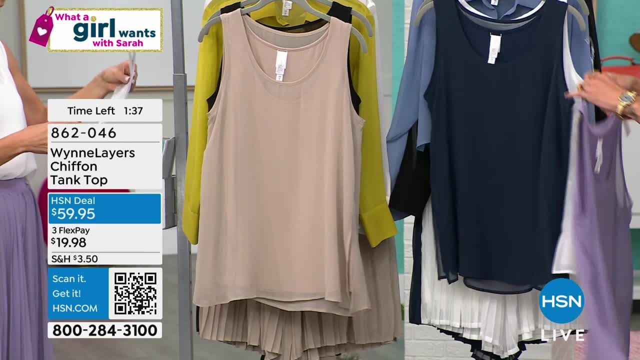 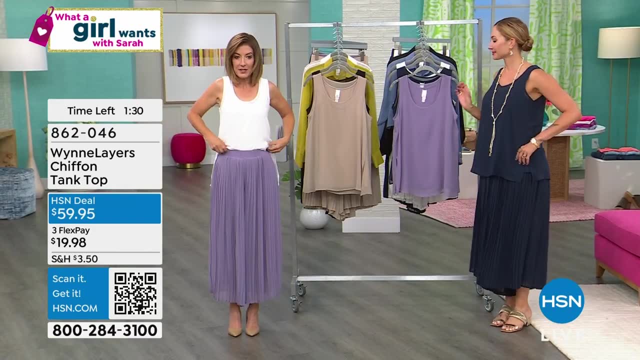 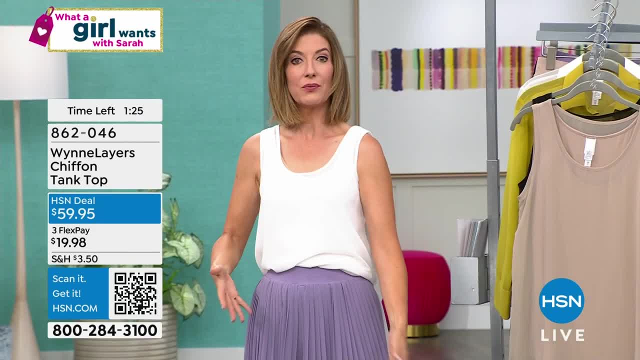 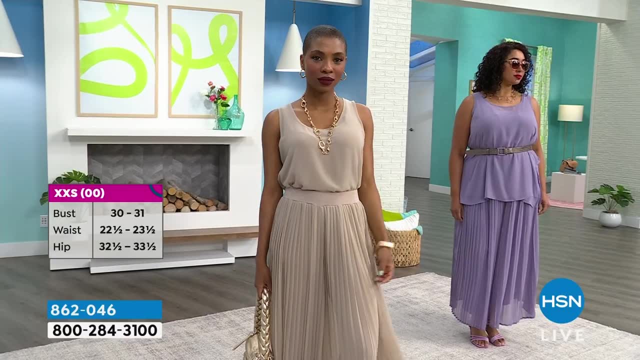 in all the way around, or you can go ahead and just let it flow. You can do tone on tone, or you can go ahead and mix it up. but if you love Marla Wynn and you love layers, this is exactly what. 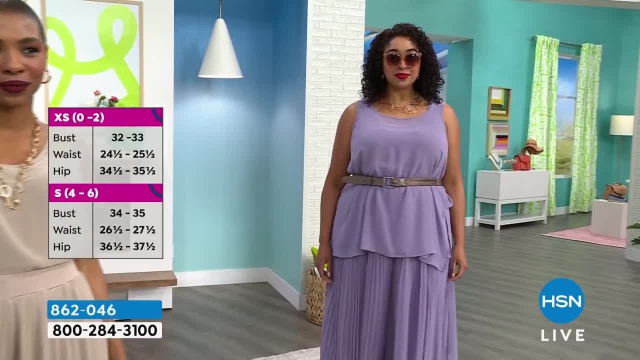 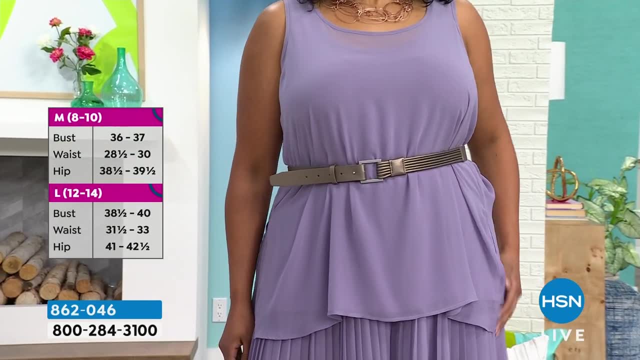 she's known for. Yes, absolutely, We love Marla's layers. This is a great, just essential tank piece because you're going to wear it with everything. I threw it on. I had my jeans on earlier. I was like, oh, this is so cute with jeans, You can tie it up. if you want, You can tuck it in It's. 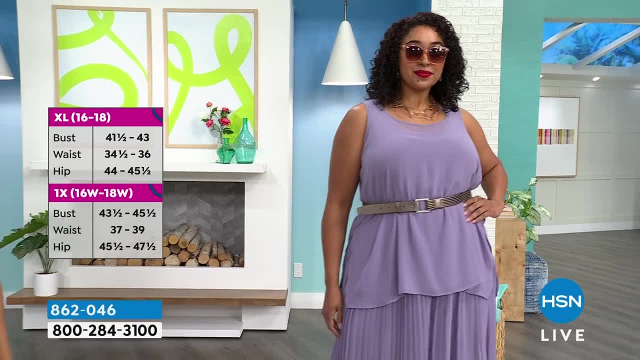 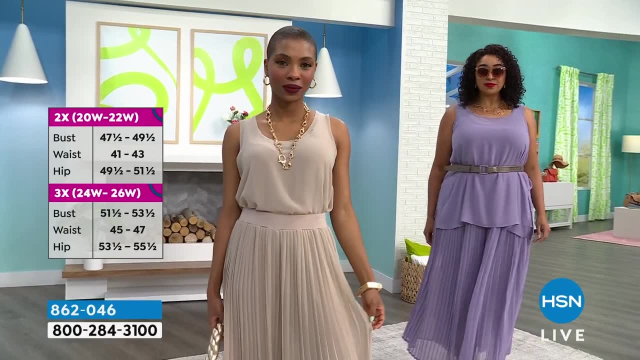 such a nice thin layer with that jersey knit underneath, and the chiffon is very light so it's easy to tuck in without creating bulk, and paired with the pants, it gives it a dress or a jumpsuit. look to it, which I think is so wonderful, and it's a great length just again to have that. 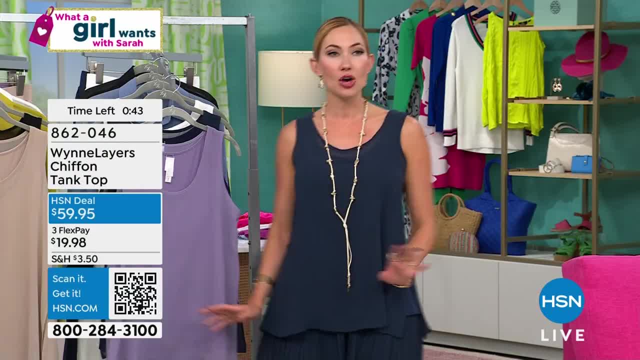 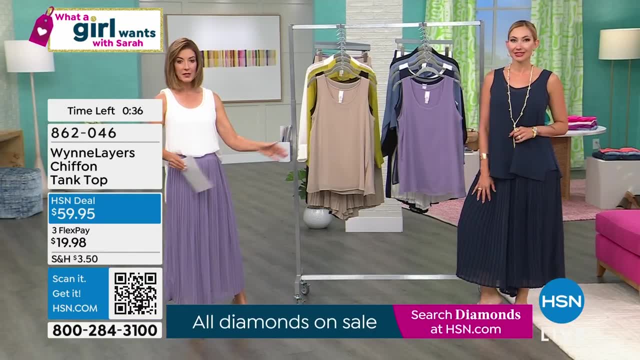 effortlessly shaped, just very lightweight flows. Look at that. I love how I mean you probably just you feel graceful, You feel pretty, You feel like if you need to be dressed up, you can be dressed up, but you still feel like you can like live your life. Yes, 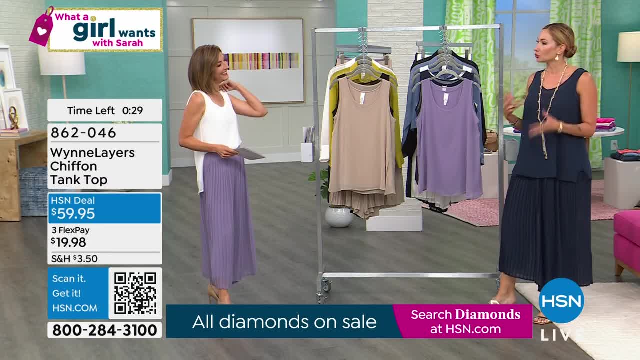 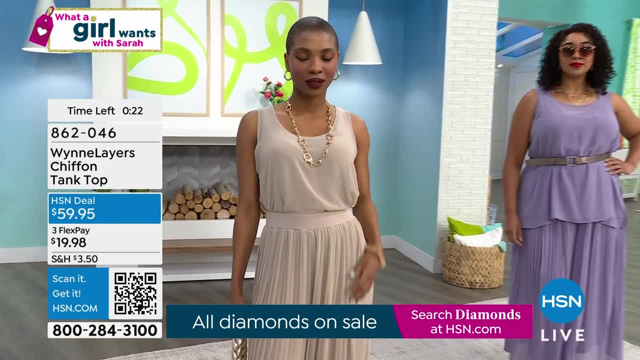 Yes, exactly. and again, and how you decide to style it, what jewelry you pair with it, can really adjust how casual or how dressy it becomes. and, of course, Marla, she has some amazing jewelry. I'm wearing some of it right now and you can find that on dot com, but all of her. 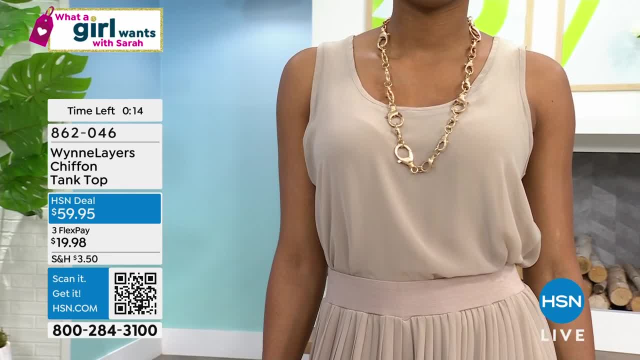 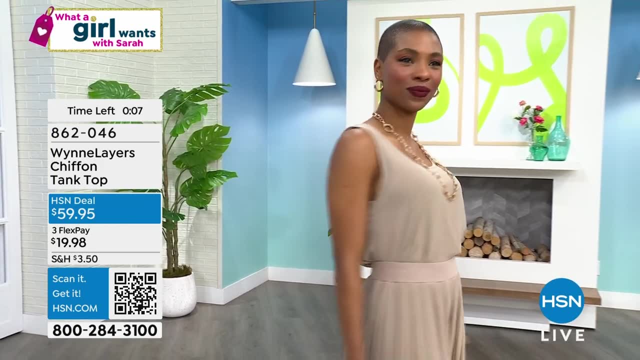 collection really pairs so well with her jewelry. In fact, it'll go great with the fit flops that we have coming up as a brand new weekly deal drop. Oh yeah, Fit flops coming up- brand new weekly deal drop- Those are amazing. I can't wait for you to get together and put your. 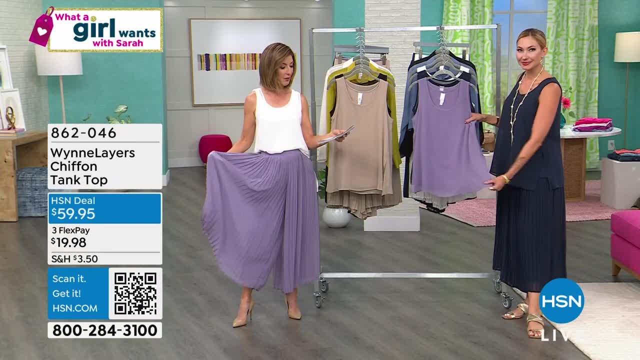 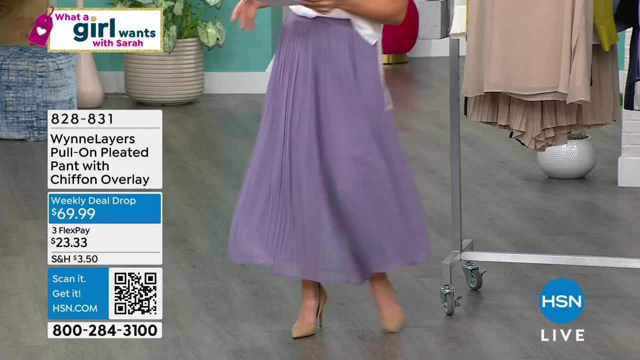 layers together. Let's give you the item for the pant one more time: 828-831.. First time we have this in petite and we have some new colors. More than 600 of you have placed your order. I mean, they're just so beautiful, They're just so graceful, They're so elegant. I mean this could. 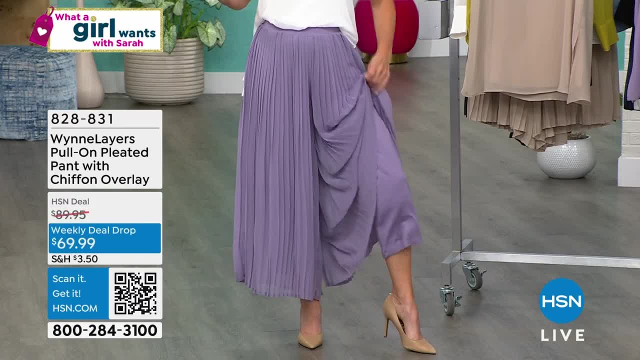 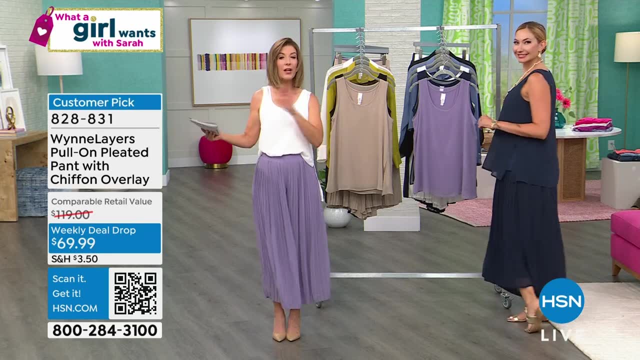 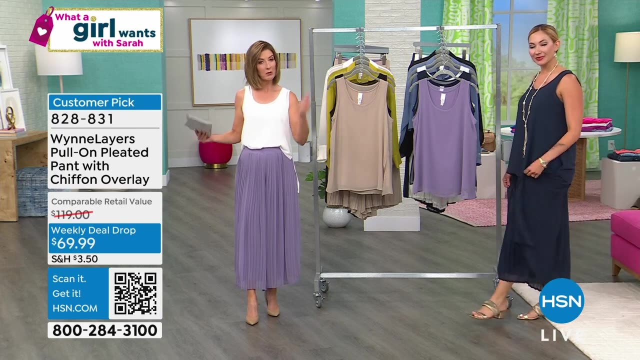 be glamorous. and remember it does come with the built-in stretchy, soft, lightweight jersey knit lining. so it just I mean they're. I can't imagine anything better. The regular price is $60.. You can't find anything like this at retail For $69.99, with Marla Wynn's quality, with her amazing. 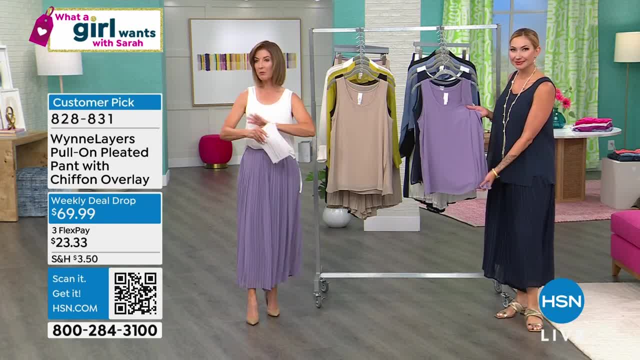 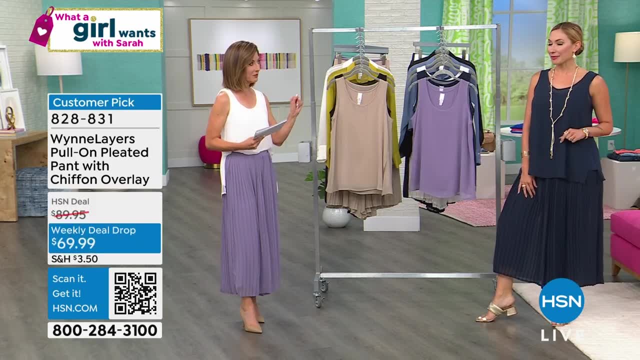 fabrics and her beautiful materials- impeccable craftsmanship. you're going to absolutely love this. So I hate that everything goes so fast on What a Girl Wants. but Amy, stick around, I'll be right back. She's got something else for you, That's right. Okay, let's talk. What are we? 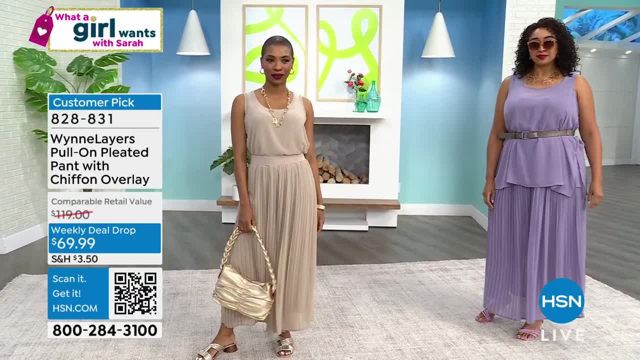 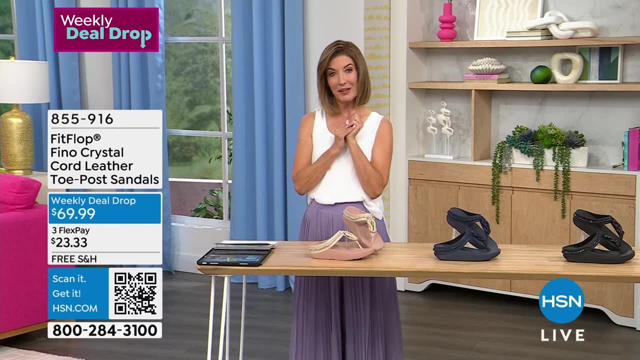 talking about? Are we going to? let's do it. Okay, I want to talk about fit flop. We love fit flop and we are going to give you a price that is like a today's special, but we don't have enough for. 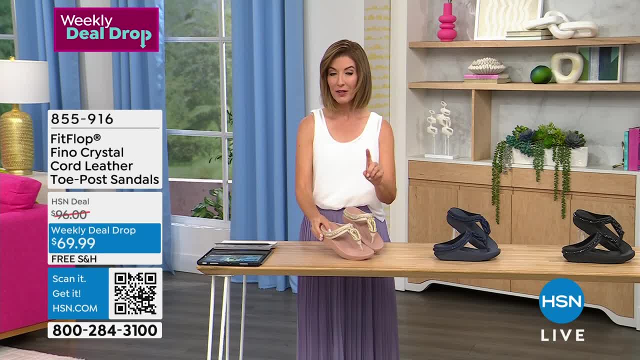 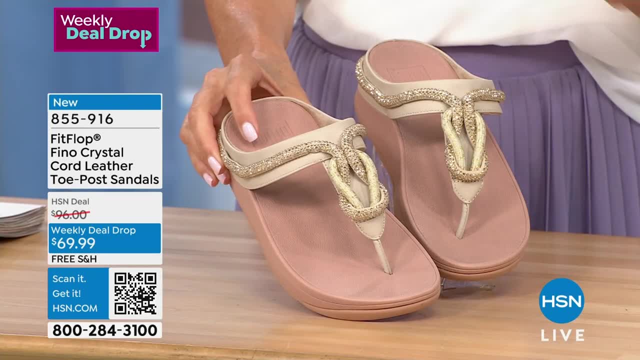 today's special, so we're going to call it a weekly deal drop. This is brand new. This is the newest style to hit fit flop nationwide. We have the best price in the market. No one else has this shoe at this price. They are also certified by the American Podiatric Medical. 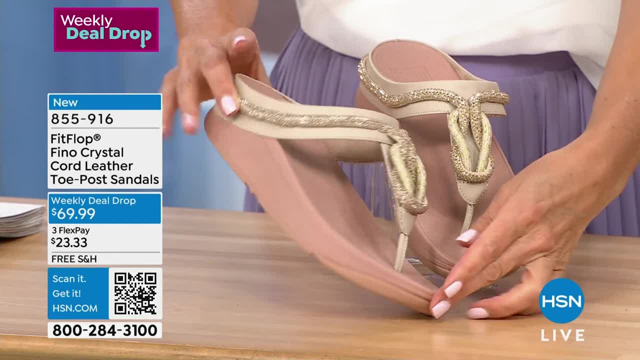 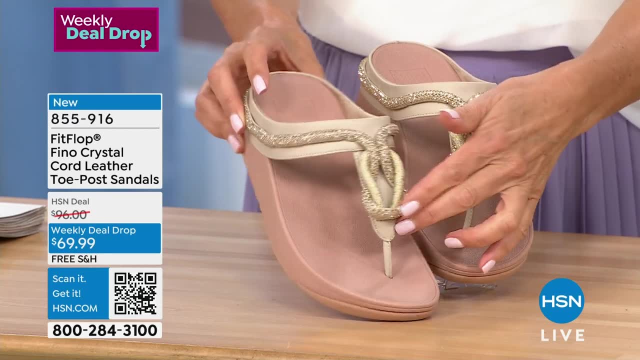 Association, the famous micro wobble board, everything that you know and love about fit flop. you're seeing in one of the most glamorous, one of the most decadent, intricate designs we have ever done: A little glitz, a little glamour, and it's a leather upper with that fabulous. 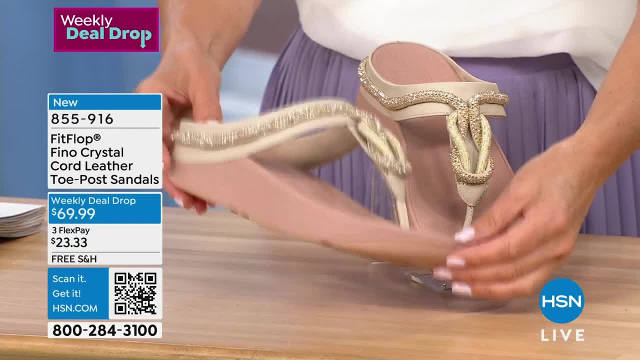 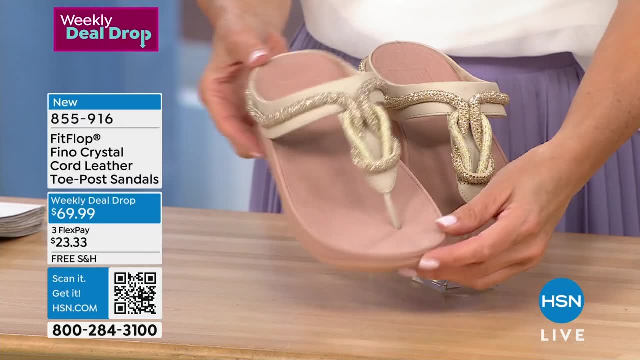 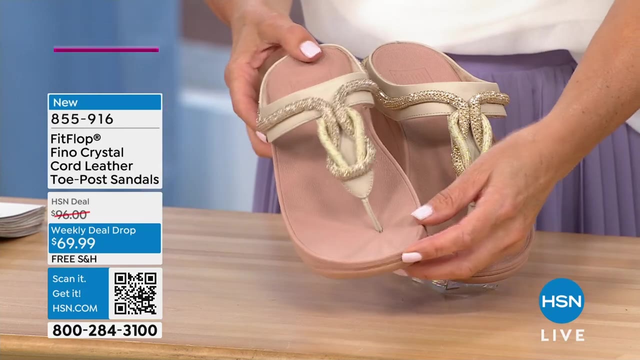 genuine leather toe post design. These are so comfortable. We have a weekly deal drop price of $69.99.. Do know this fit flop is never under $100. They are never under $100 and we're doing this for $69.99 with flex pay and free shipping. This is the cost of a fit flop. We have a weekly 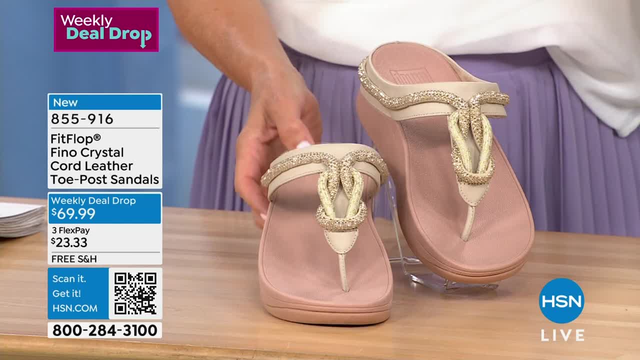 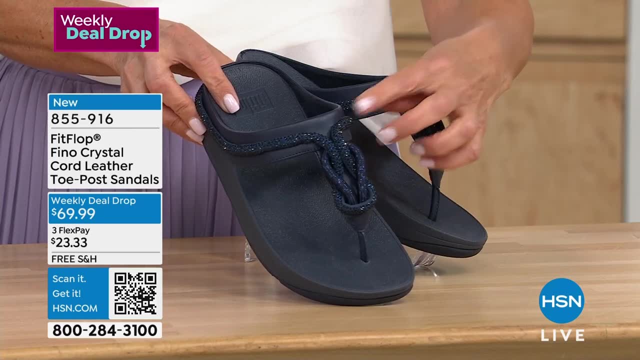 deal drop price of 3.99.. So if you're looking for some extra cash, you can purchase and add free to all of us. So we are the largest vendor in the United States. We bring you a direct order for any fit flop. We have a weekly deal drop at ftflcom. So if you're interested, 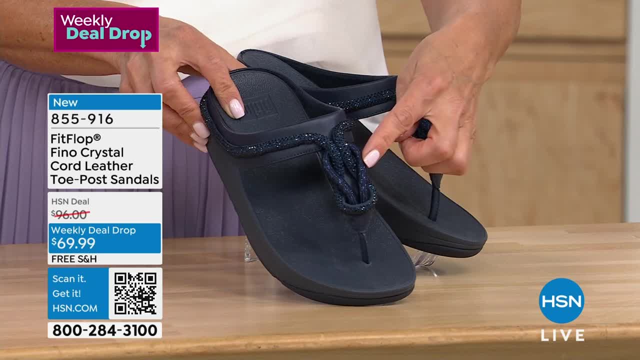 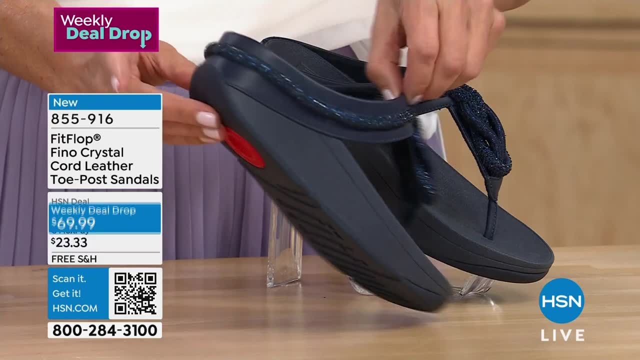 I have some desert go and if you're looking for a fit flop, you will find this at the dollar store And we're here to give you our daily deal drop rate. So we have free mail and post delivery And with that check we'll be right back out in just a moment. 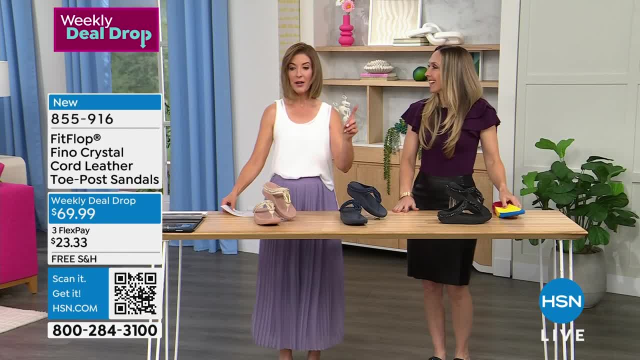 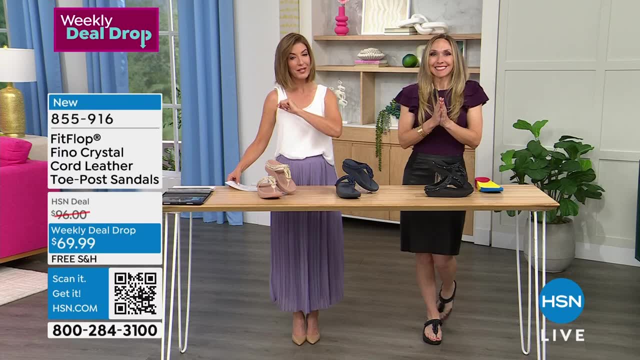 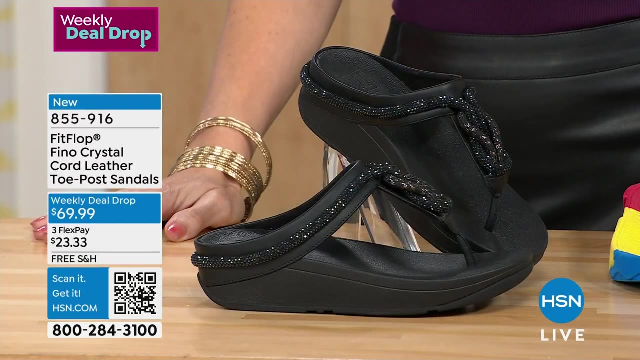 know you're gonna love the black. and not only do we have a brand new shoe at the lowest price in the market, we have special sizing just for you here at hsn. for the first time ever, we're also offering this in half sizes. so check out the half sizes, several available between 5 and 11. 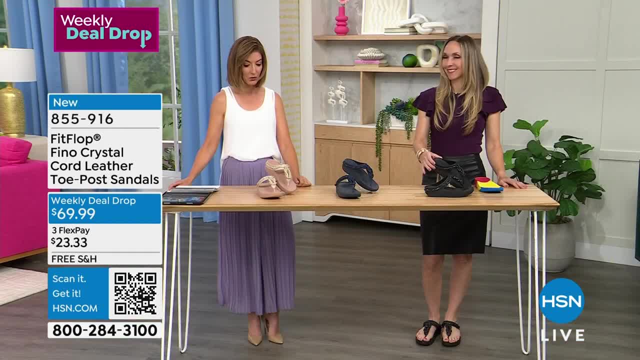 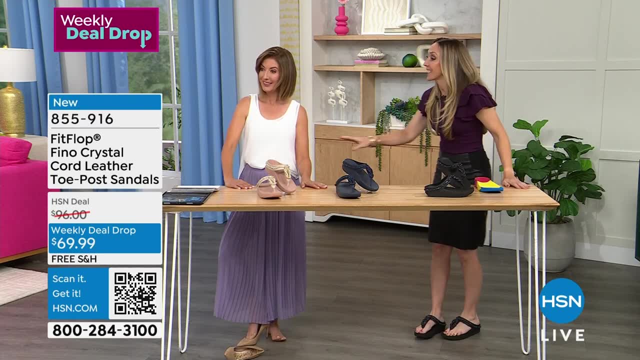 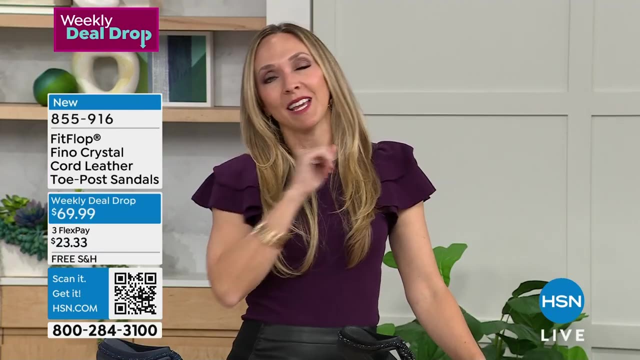 but randy harvey as our fashion expert, uh, you are the queen of fit flop. i know you. i know you own a few pairs, just a few. i'm gonna put these on right now. i was about to tell you that i saw your heels, my three inch heels, and i can happy when i'm here. i mean, i like to think it's me happy feet, it's not. 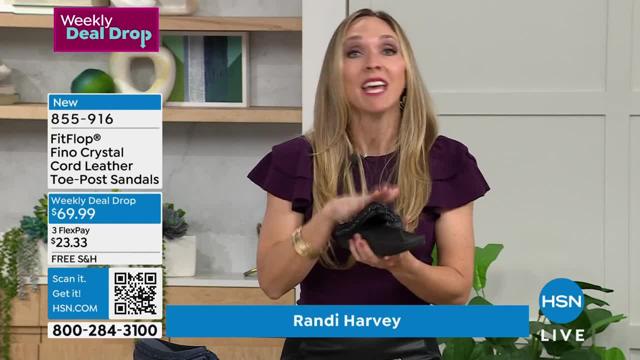 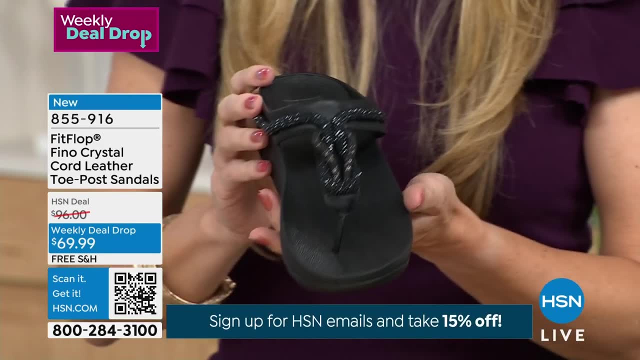 it's the shoes. i'm not offended because fit flop are amazing if you've never heard of the brand. so we were the first ones to mix high fashion with shoes that are approved by podiatrists. so this shoe, this gorgeous, beautiful shoe, is approved by the american podiatric medical association. so 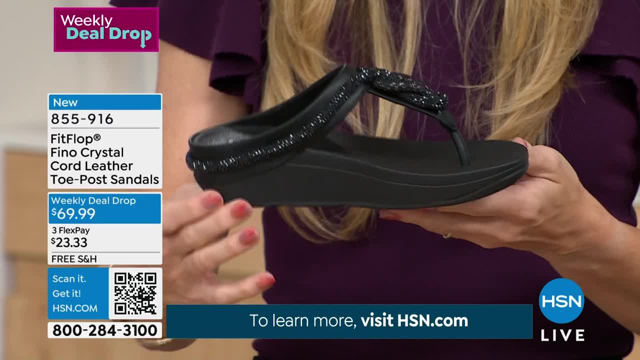 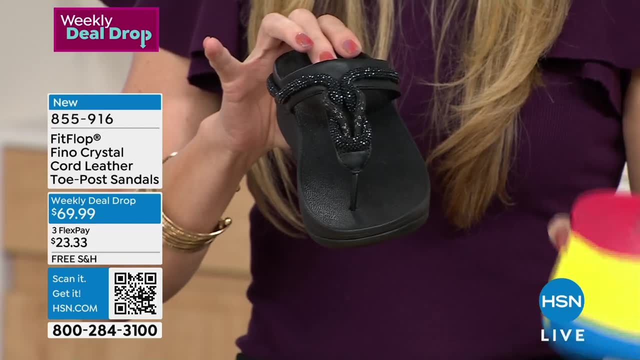 what does that mean? that means that this shoe not only looks good but promotes foot health, and we have an on-staff doctor of biomechanics who creates all the technology. i'm just going to show you the technology in this shoe. it's called the micro wobble board technology. this is a triple density foam. you have firm cushioning at your heel. 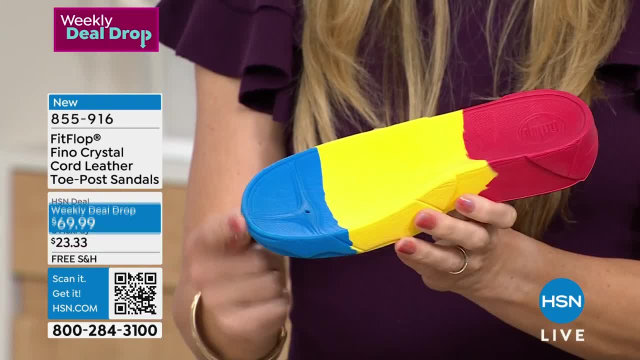 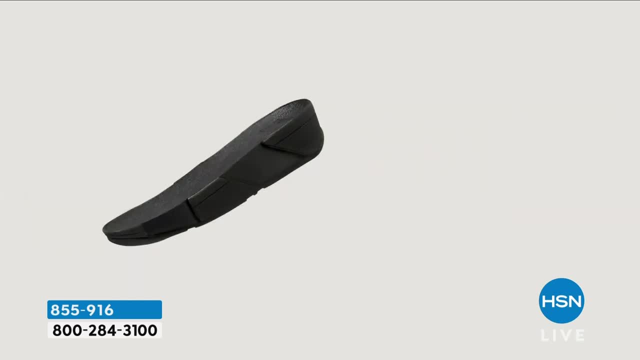 soft foam at the arch of your foot with a medium density foam at your toe box, and you notice that lift. it's to properly align your foot. so as you're taking that step, that strike pattern, everything, all that shock is absorbed. all of your weight is evenly distributed. 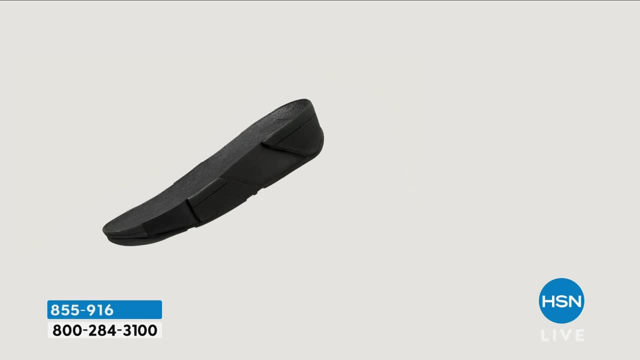 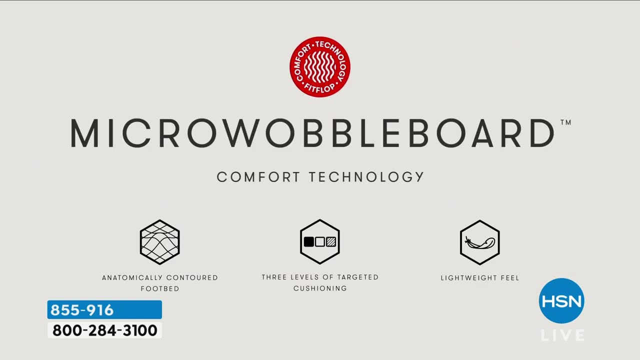 you're going to be able to do a lot of different things with this shoe, so i'm going to show you. so you get to wear a sandal that looks like this, that is good for your feet, that you can wear all day long, padded toe post. now, all this embellishment on the upper is gorgeous, but underneath you don't. 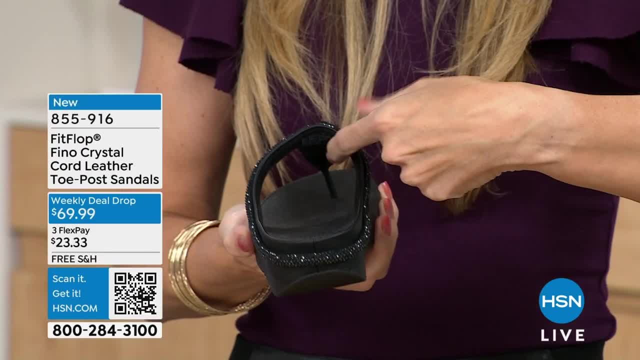 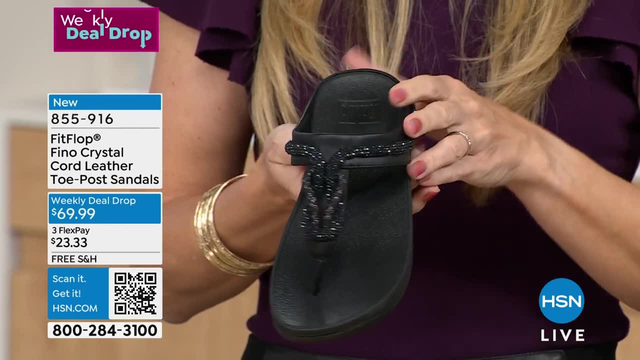 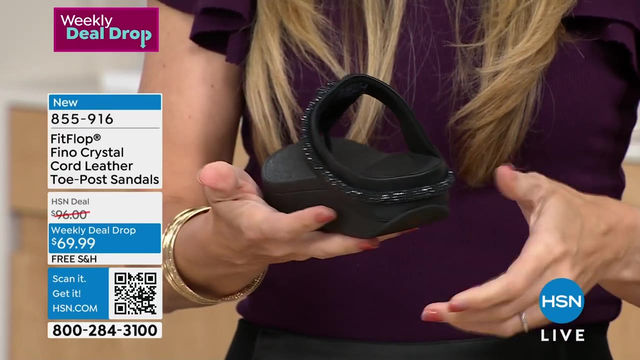 want that touching your foot right. so we have a microfiber lining that is super squishy and plush. it really feels almost like you're wearing a slipper all day: comfort and wear. this is so glam, feather, lightweight, so lightweight, with all of that enlightenment all the way around. on a weekly deal drop, and it's brand new. not kind of new. 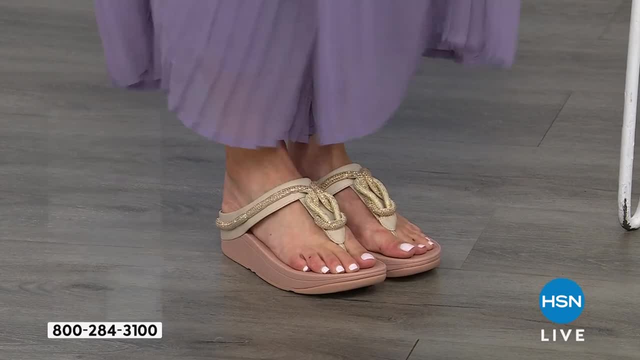 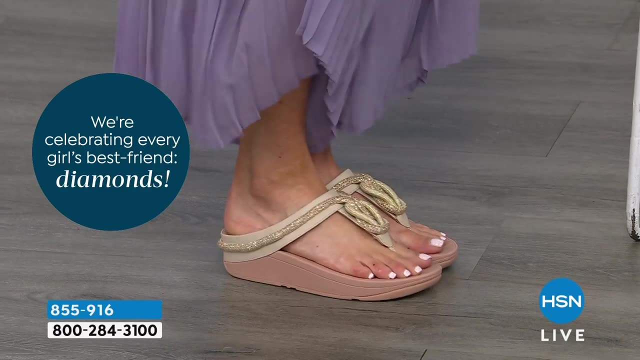 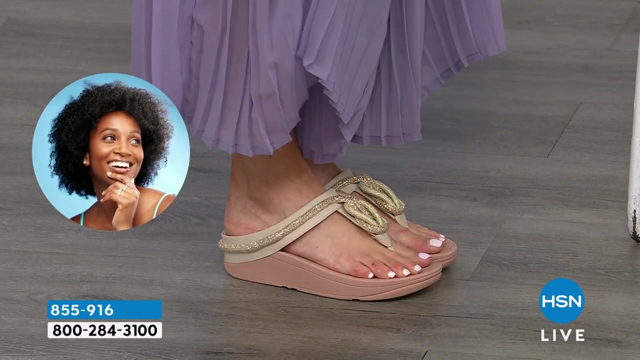 not sort of new, as in: i literally got. i was on the phone with you, sir. i got these shoes an hour before i left- you're the first to see it- yeah, and they just were shipped to me. i order flip flops, uh, in just about every single version you bring in. i also, uh, end up taking calls from my friends and 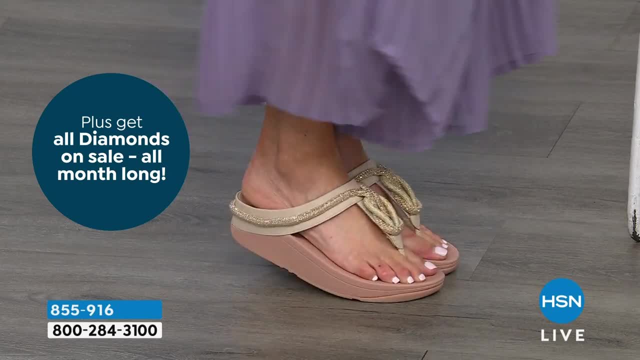 family members when i answer their text messages. will you just tell me when you have a fit flop moment, because there are about a hundred fans out there and they're all saying they're going to get a flip flop moment because they're about a hundred times more similar than i thought and so that's. 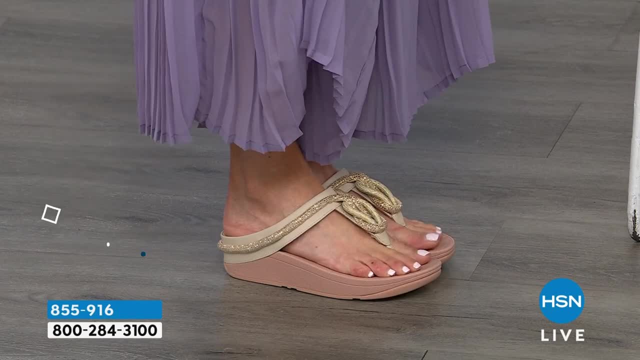 going to last you a hundred" ROE saya, our top territory. We're gonna thank you for bist agencies, from시죠 and ministries, motel dg for bringing them couture to you and dollars at retail. this shoe is a hundred dollars. it's all the technology. it's this really cool. 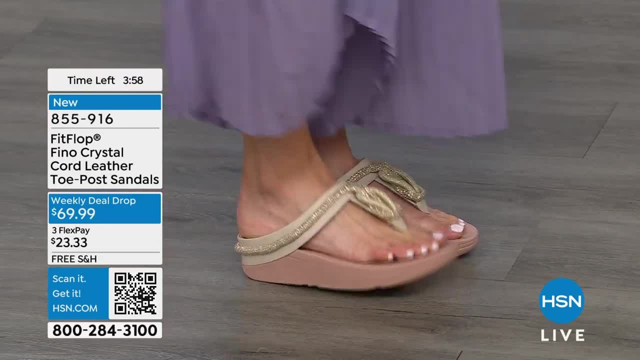 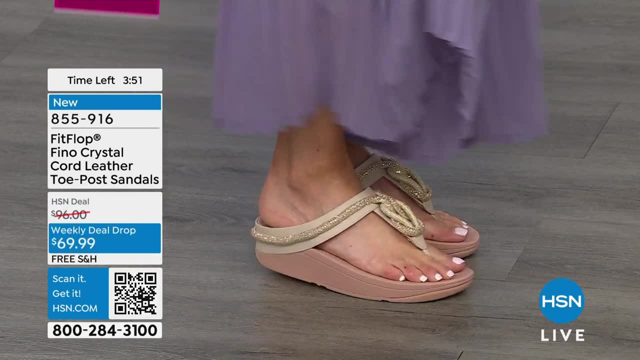 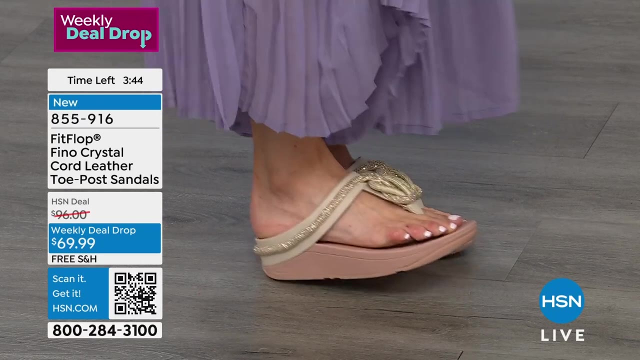 bottom. look how thick the bottom is. this is not flat. this is not a little piece of cardboard. this is not something that you're going to slip and slide on, or you're going to feel the pebbles and the bricks and the cobblestones underneath your shoe. you feel nothing but that amazing super. 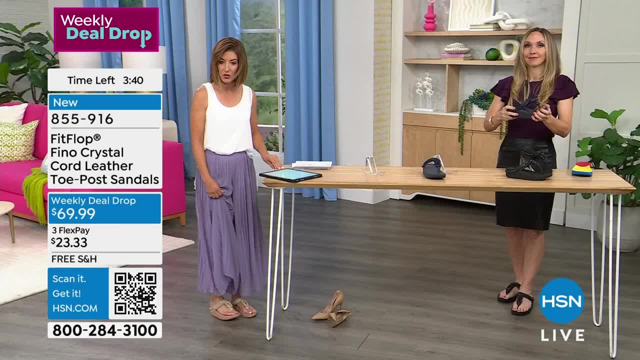 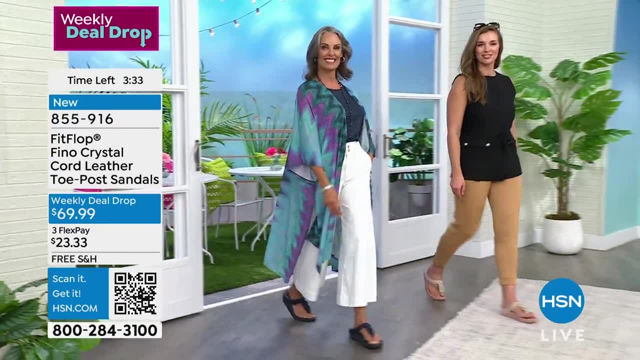 padded, super cushioned bottom and that's what fit flop is known for. they have the arch support, they have that sort of pressure relieving cushion with every step. it just kind of fits your foot perfectly and that's why these are going to go very quickly. they're usually a hundred dollars. 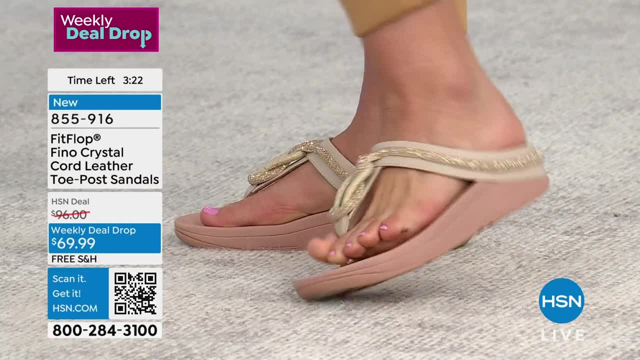 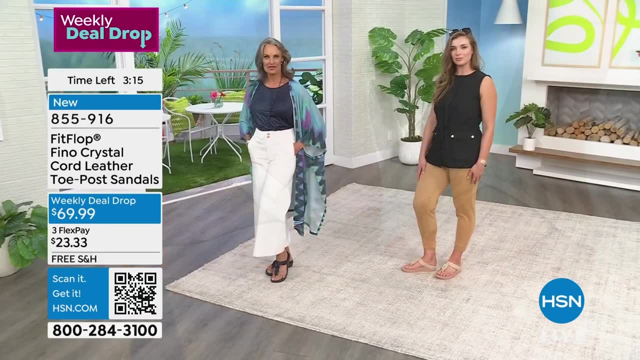 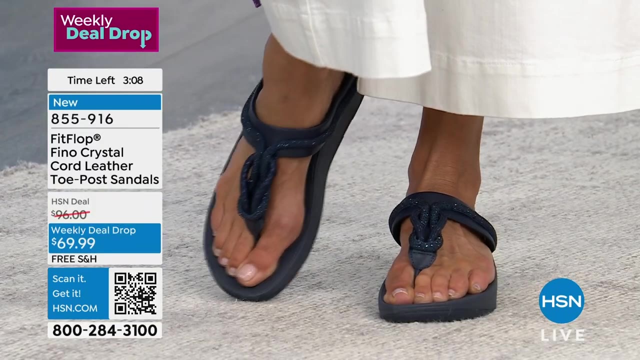 right now they're $69.99. we have all sizes and let's talk sizing: so exciting. so we have half sizes for you tonight, which we don't usually do, but due to your customer requests, customer demand, we've added a few more sizes for you that you can add to your shoe box. 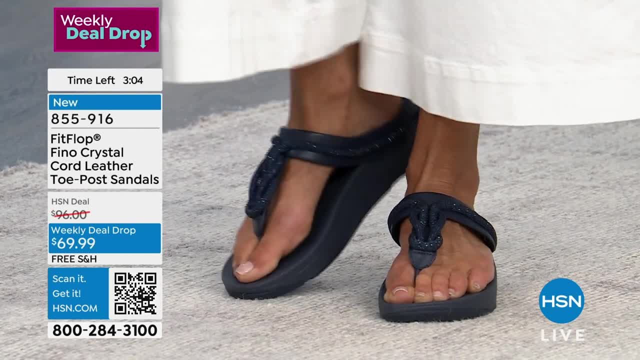 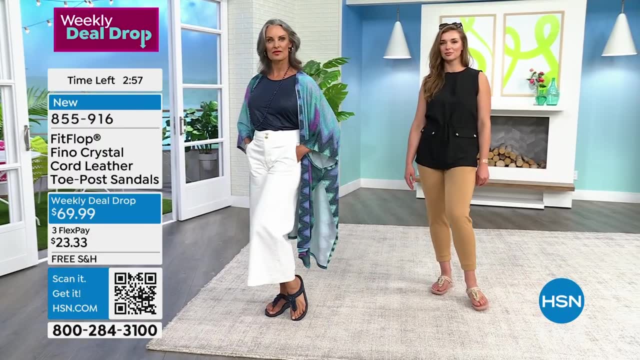 and how would you consider sizing fit flop? so we have whole sizes, 5 through 11. and then now we carry in this sandal just here to hsn six and a half, seven and a half and eight and a half. so if you see your size, go ahead and grab that. but let's say you're a nine and a half typical to normal. 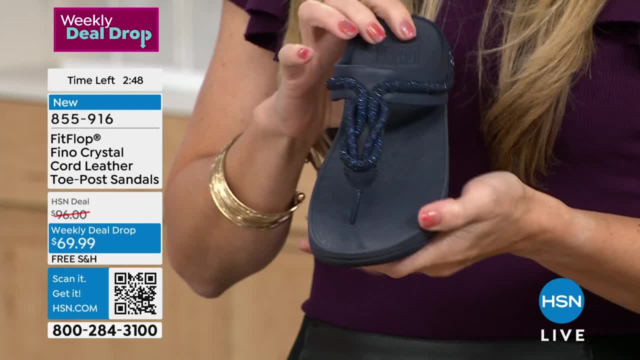 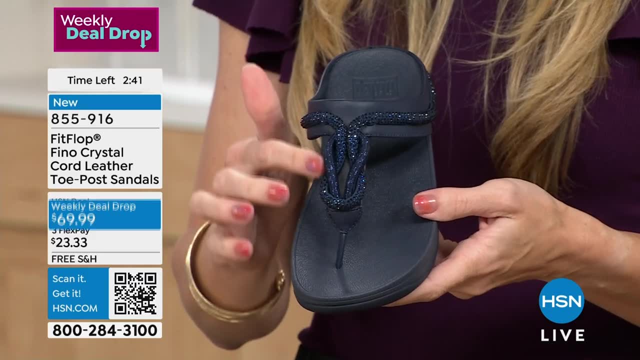 fit flop sandals. you're just going to size down to the nearest hole, but i am obsessed with this knot. this reminds me of those that jewelry, you know, those really long necklaces with the beautiful knots on them. so fit flop really has mastered that and i'm going to show you how to do that. 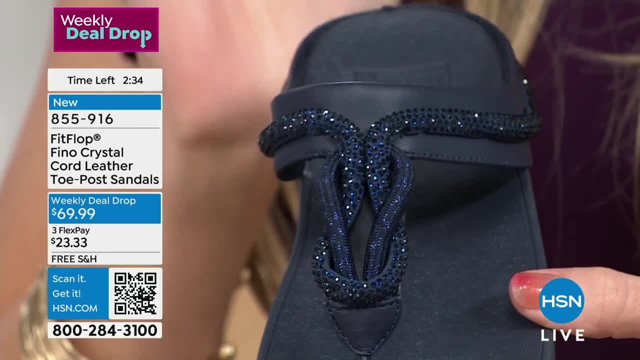 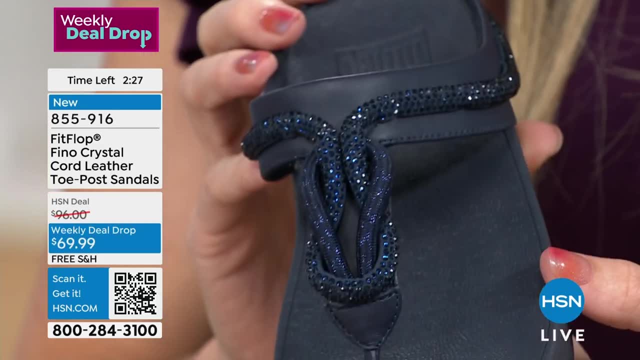 jewelry for your feet, and so this is that midnight navy. if you are a denim girl, if you love your jean shorts or if you love white jeans, this would be beautiful, very americana, with all the different holidays coming up, but a lot of us have black shoes, a lot our sandals, rather a lot of us have. 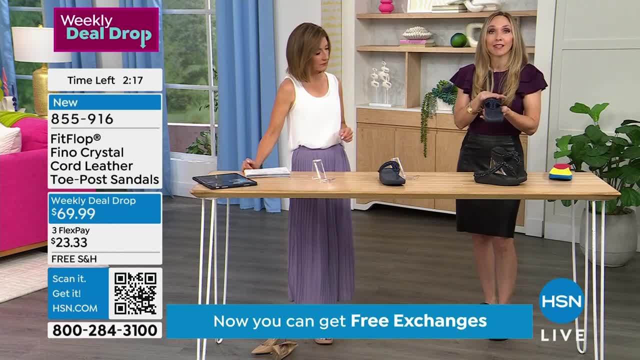 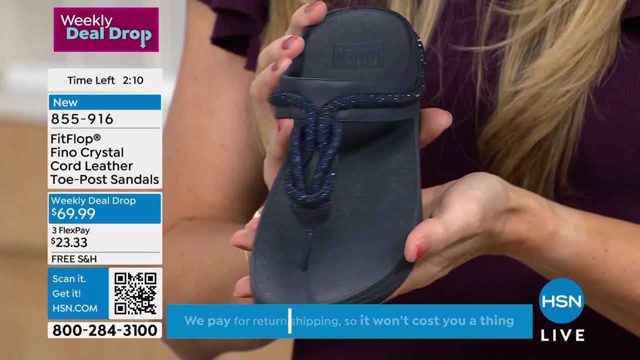 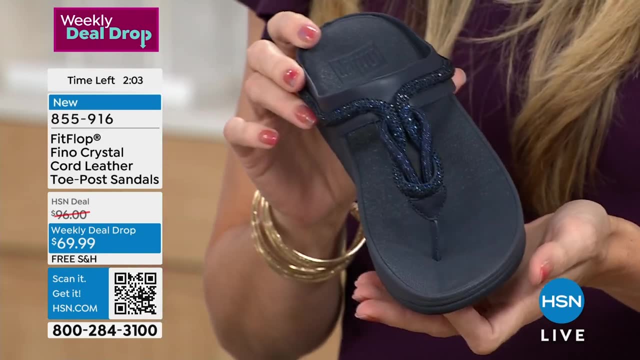 you know, a nude sandal try. this is one of the most underrated neutrals, is what my girlfriend megan says. the stylist she says i like it. navies are very. people forget about the navies. so grab a pair of sandals if you are a ten year old, and you're a ten year old and you need something. 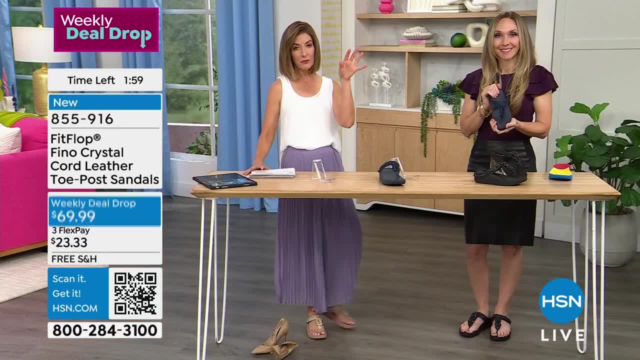 for your feet and you need something to wear on the day you're in the store or if you're in your closet, especially when they're on super. uh, we are getting busy now and i know a lot of you just wait for a fit flop today's special. i don't want you to wait for a fit flop today's. 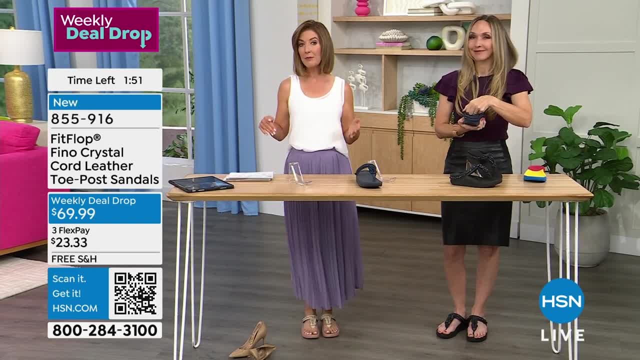 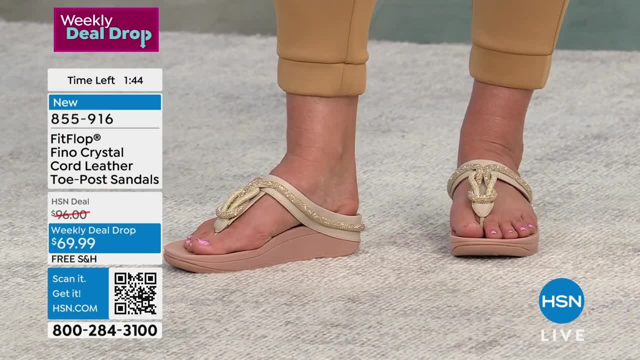 special because there won't be one until later in the summer. so this is this is your spring going into summer shoe, and this is the best time to buy fit flop when they're either today's special or a weekly deal drop, we don't get to do a lot of them. also, what you're getting is the newest style look. 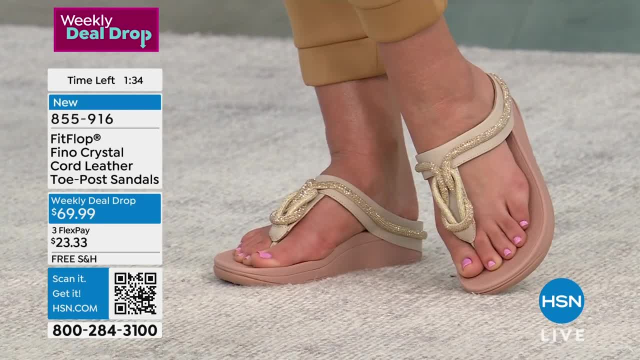 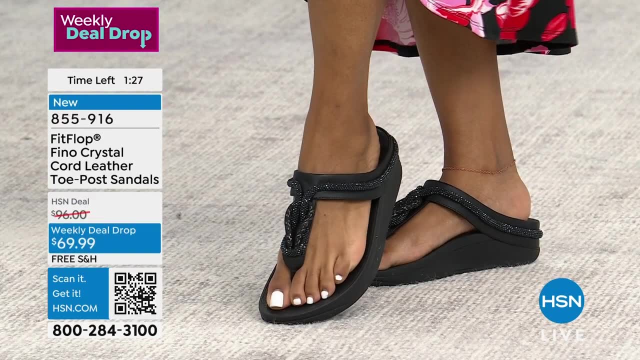 I know you described it as sort of having like a little nautical knot or a loop. It could be, yes, it could be extra glam, But also this is a genuine leather upper, just to kind of add to the luxury and the value that you're getting here today. 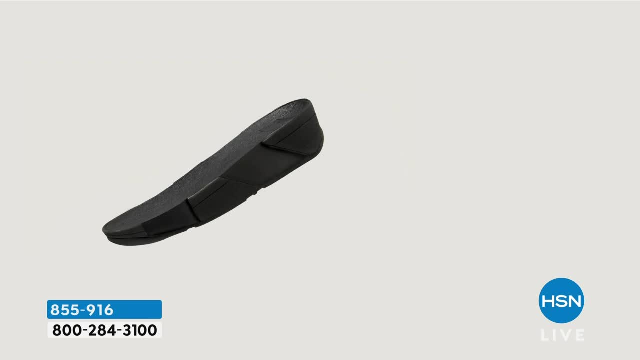 Not to mention what is a micro wobble board. So that's what really sets us apart. We were the original high fashion shoe that was approved by podiatrists. Not like kind of these are okay, they're comfortable, They promote foot health. 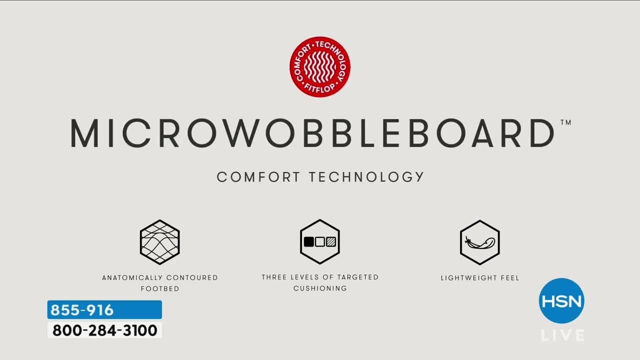 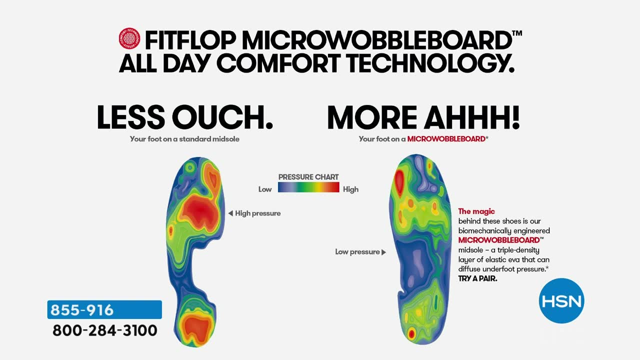 That micro wobble board technology is a triple density foam that it really supports your foot on every level. So look at I love this graphic. On the right hand side is what your foot looks like standing in a micro wobble board sole. On the left is what your foot looks like in a basic flip flop. 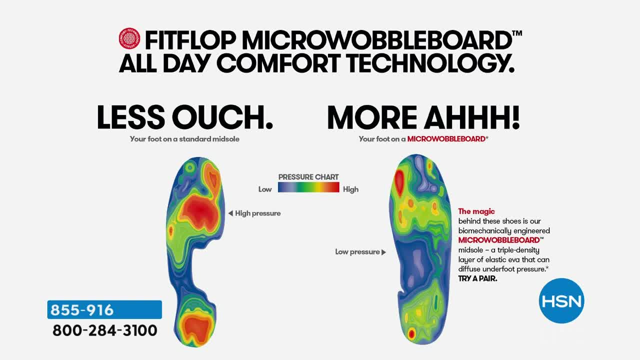 And notice all those red spots. That's all of your body weight just balancing on the ball of your foot. That's why we get foot problems. is wearing bad shoes? or you and I dancing- for all the years we danced Right, Yes, Just all the, all the. you know what we do to our feet in our 20s. 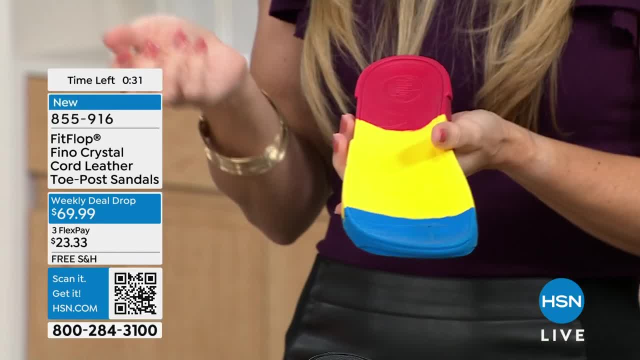 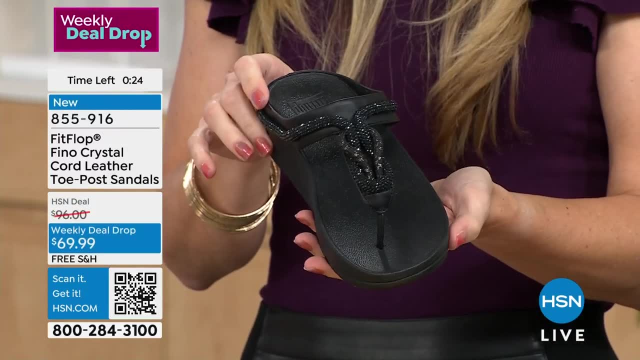 Now we have to wear shoes that really promote foot health because of what we have done. But I'm going to show you the glam though Here. look at that Like we don't have to wear those orthotic shoes anymore. These are shoes that are designed to promote good foot health. 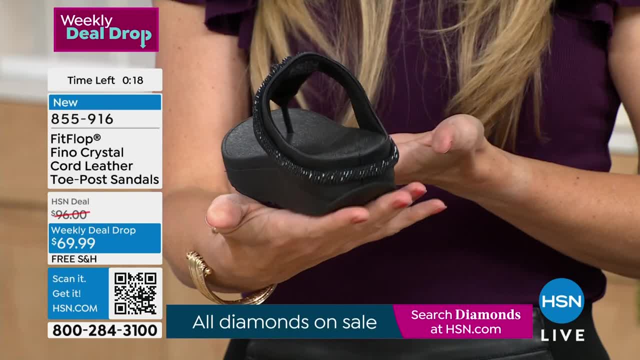 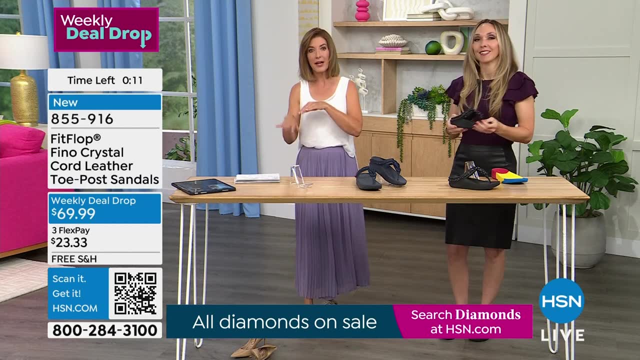 We don't have to wear- for lack of a better term- old lady shoes. You know, all of a sudden you're wearing really cute, really high fashion shoes. Then all of a sudden there was like nothing in between And you realized I have to wear the shoes that the doctor told me to wear. 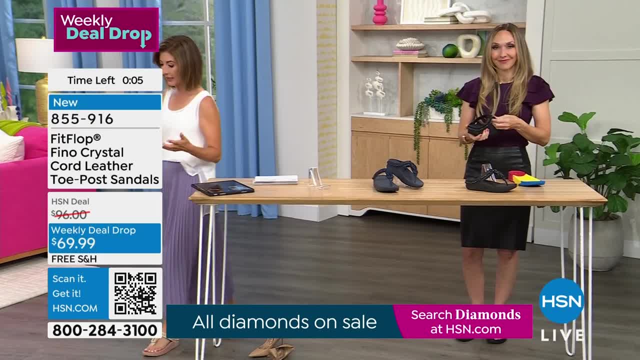 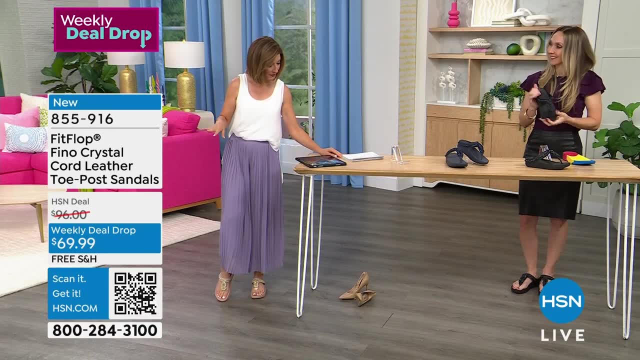 Right, I have to wear shoes that are more steady. give me more stability on my feet. This is very, very popular. I'm going to go ahead and wear the color. just to kind of go through the colors again. This is stone beige. 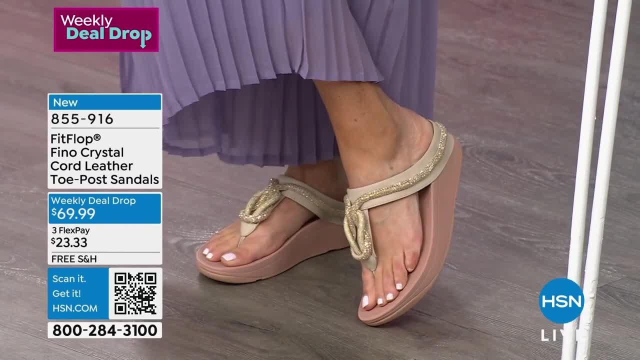 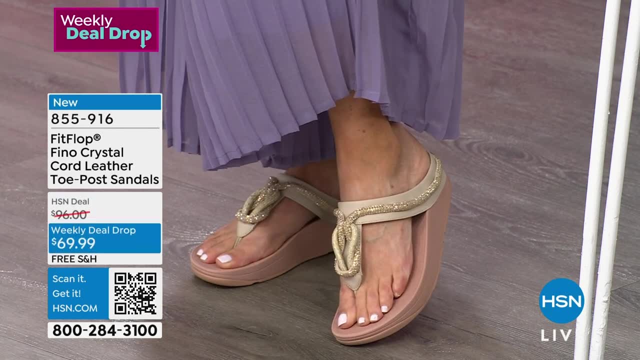 And then we have navy and we have midnight. Now, if you are a true aficionado of Fit Flop, you're getting more than one, because it's not every day we give you. I mean, usually the shoe is over $100 at retail. 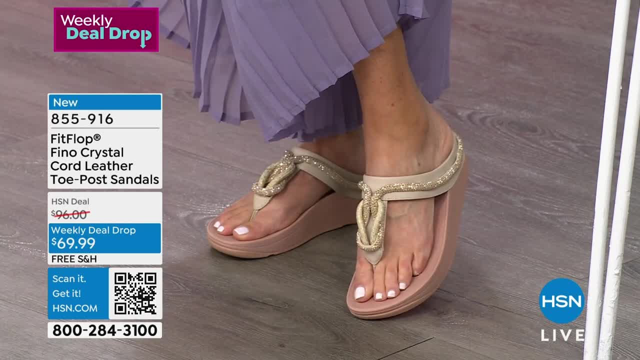 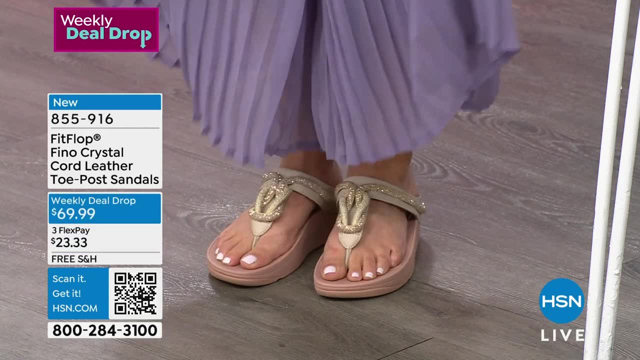 I can tell you this: This is the best price in the market. No one else has this shoe at this price. Also, no one, No one else has this shoe with all the sizing. I'm a six and I wear a six. 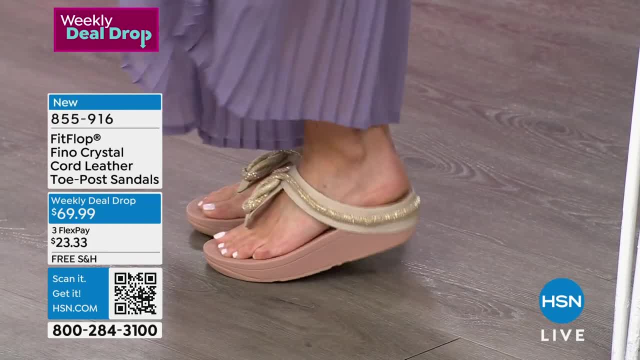 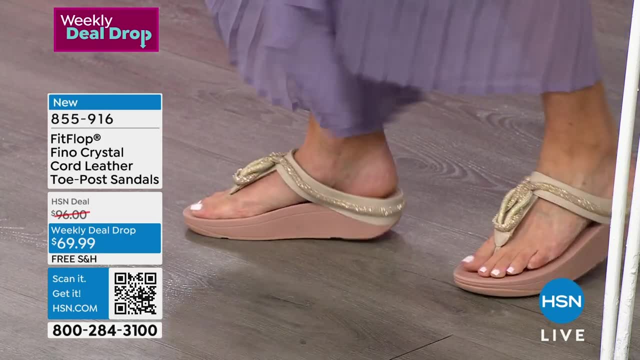 Look at how perfectly it fits. It's very true to size. You've got a lot of wiggle room. Notice how it kind of comes up. See where it meets the inside of my foot. It follows the natural motion that you walk from the heel. 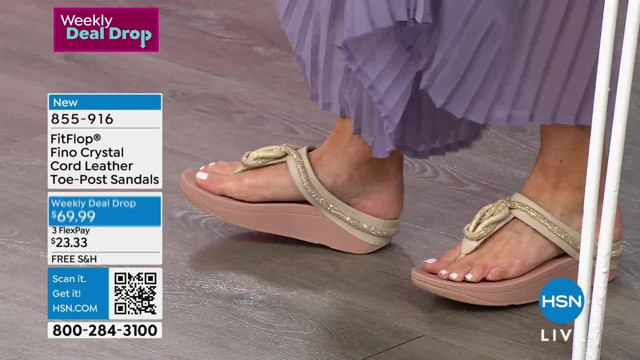 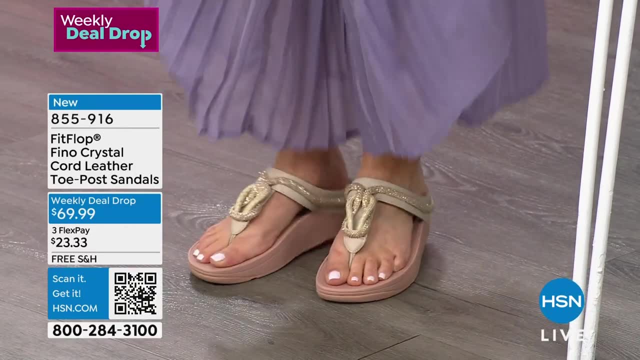 Pressure relieving, You don't hit the ground with that extra force And goodness knows, we put a lot of pressure on our feet. We take, you know, thousands of steps every single day. Okay, If you're just standing a lot, whether you're at work, or whether you're on the go, or whether 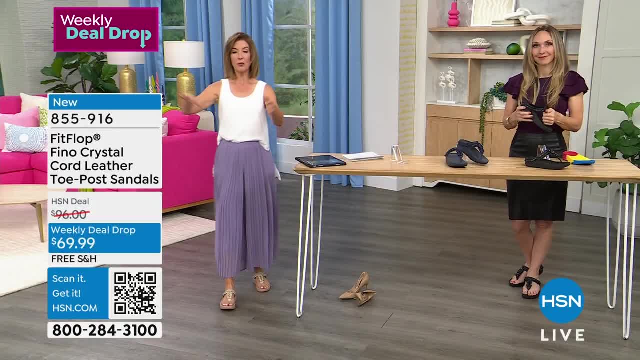 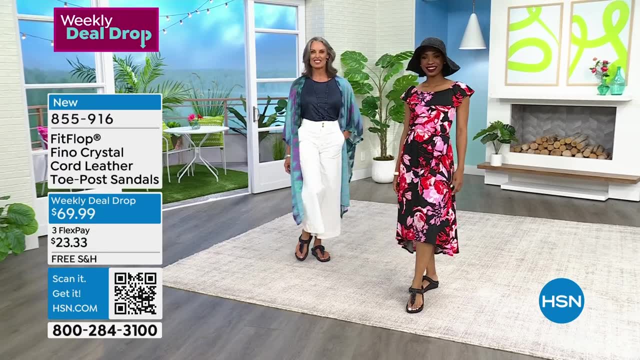 you're on vacation, or whether you're strolling the boardwalk and you're just enjoying all the sightseeing that you're going to do this spring and summer, you know. find a shoe that you can walk in. find a shoe that you can stand in. find a shoe that's approved. 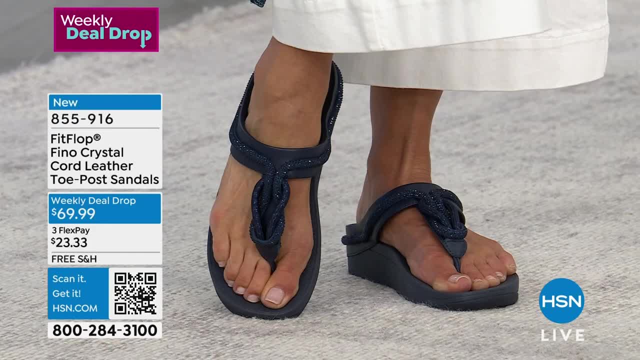 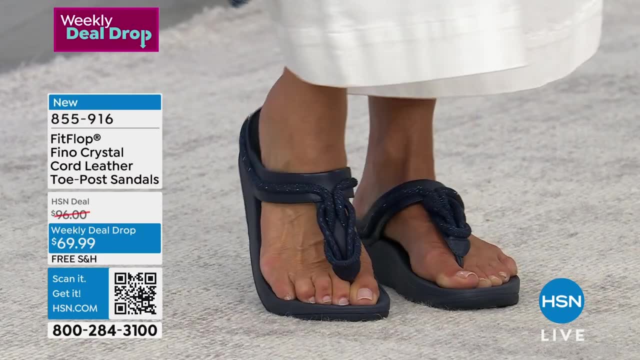 And especially when, when a podiatrist approves a shoe That looks like this, That's a big deal. Well, right, And that looks like this. A lot of people say. we heard about the brand through our podiatrist And normally when you think of shoes that podiatrists want you to wear, they're horrible. 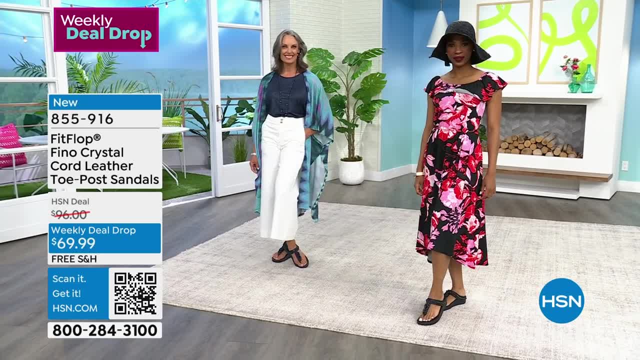 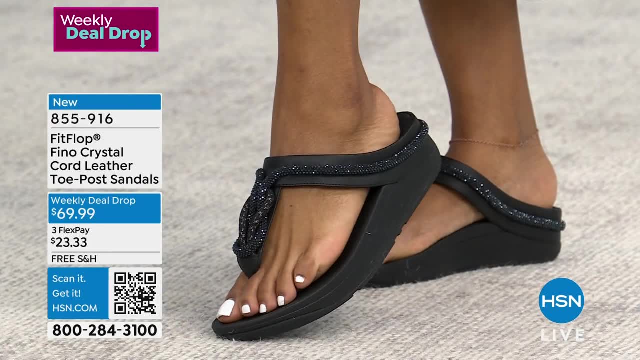 Not attractive, Like they're horribly unattractive. So fit flop really filled that niche. So you can wear this with just jeans. You can wear it with jean shorts, but this is also if you can't wear heels anymore. this would go perfectly with any sort of dress that you're wearing. 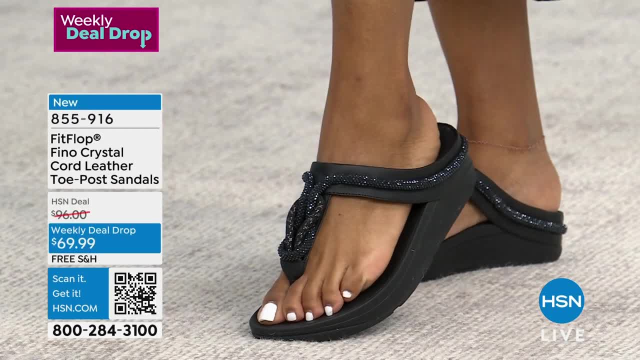 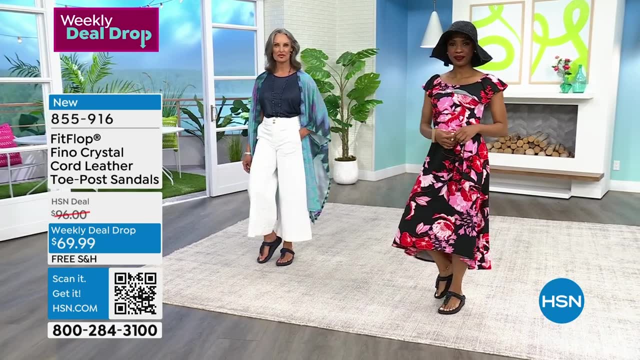 I'm upset. Oh, also slip resistant too, which is very. stability is very important for foot health. And Mary's here, She says hello. Teddy says yay, half sizes, And a lot of you are loving fit flops. 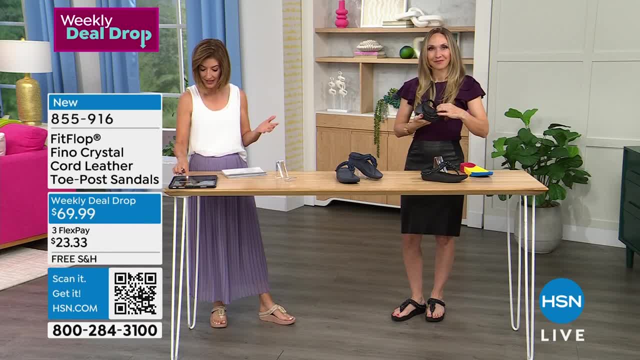 Tracy says I love fit flops, I own a pair of sandals, And then she also has the tennies. Jill says she's wearing her fit Flops right now. It was like it was like meant to be Jill. 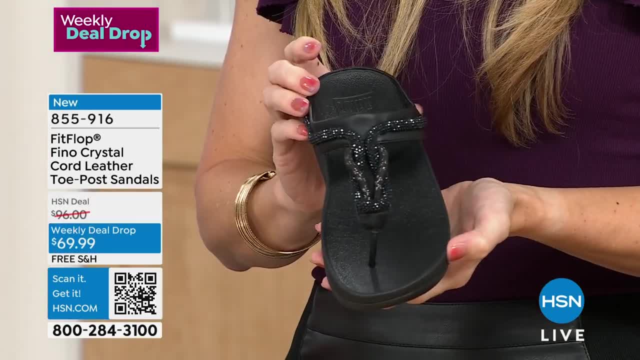 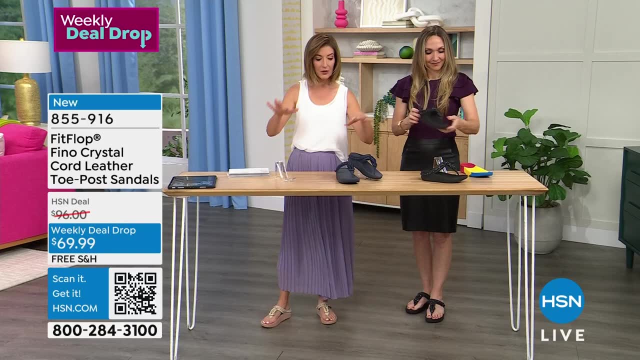 And so thank you so much. I love that we have all these great colors. This is our first presentation of the weekly deal drop. There will never be a better option for you to get your first color choice and your size. So, the first time ever, we do have some of those half sizes. 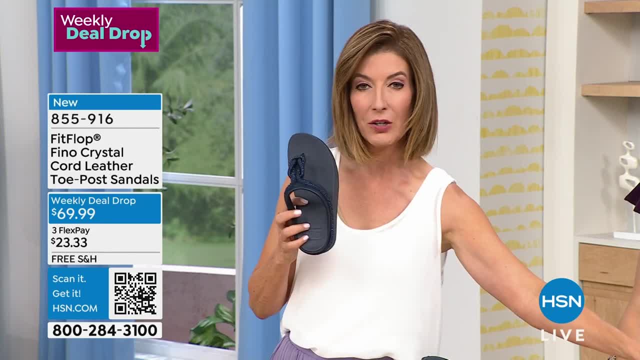 Let us get this out to you: You're going to love them, No matter what color you get. you can't go wrong. But I'm not giving that stone beige color back. I'm going to. I'm going to wear those for the rest of the show. 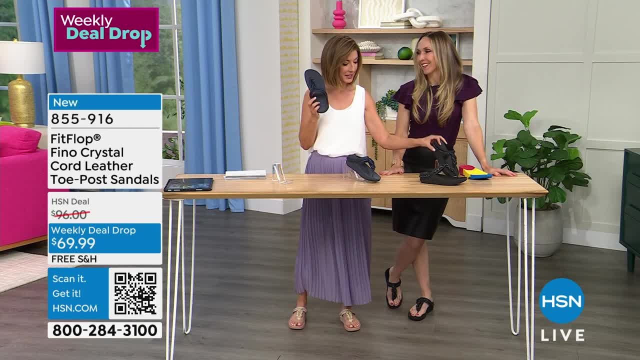 Cause I've got. I've got another Hour of Rhonda coming up and she's going to keep me on my toes. Yeah, Why are we? why are we wearing uncomfortable shoes that are not good for our feet, Or uncomfortable bras, right? 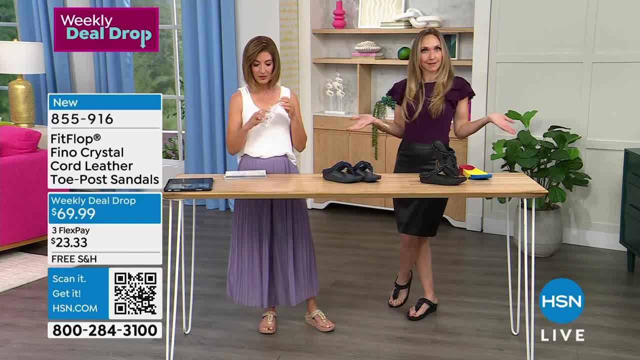 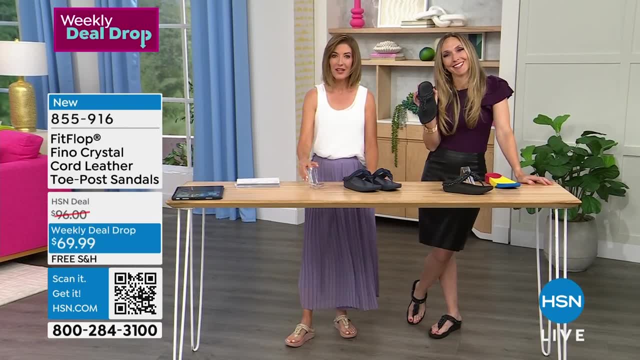 So you're comfortable. you're comfortable in your feet. And then up here, Did I mention I hate these plastic things? I just I destroy every presentation. We love the shoes. We love the shoes. No plastic parts included, Brandy, thank you so much. 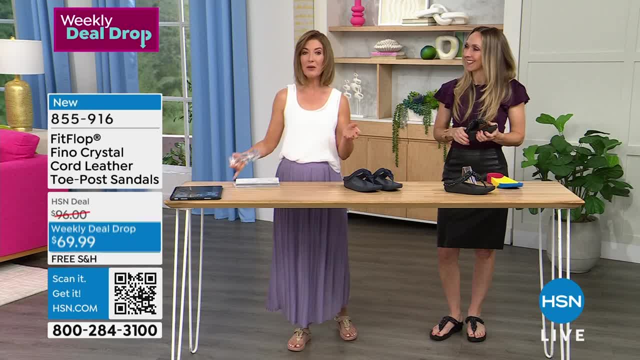 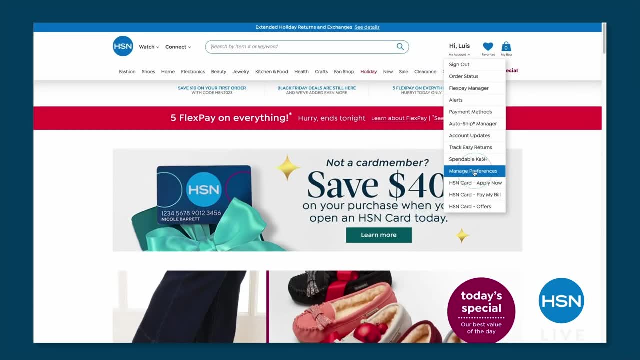 Great to see you Always, always a pleasure. Fit Flops going fast. When would you like to watch your favorite show? Do you have a favorite host? Well, is it a favorite show Like what a girl wants? You can customize your emails. 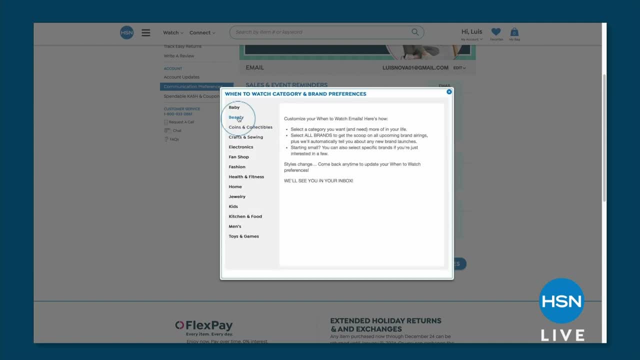 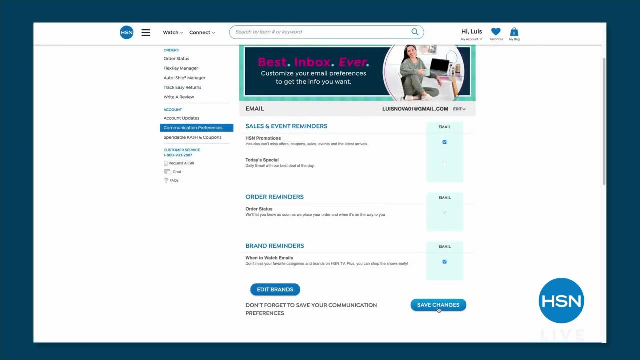 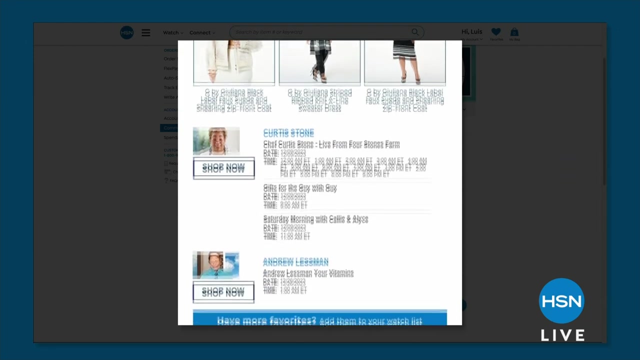 Just go right to your account on hsncom and we can get this out to you. So that would be the perfect time to kind of sign up and place your order And we're going to, we're going to. we're going to pause because what I have coming up are some really cool ways to say I love you. 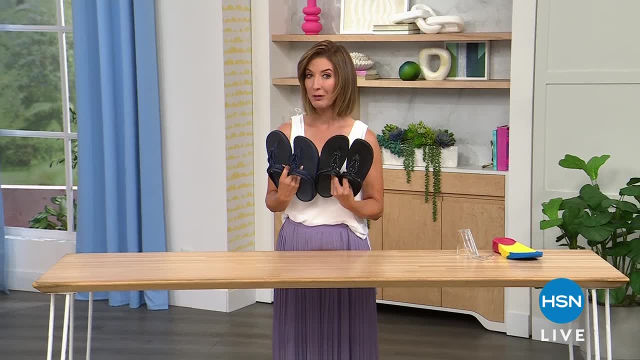 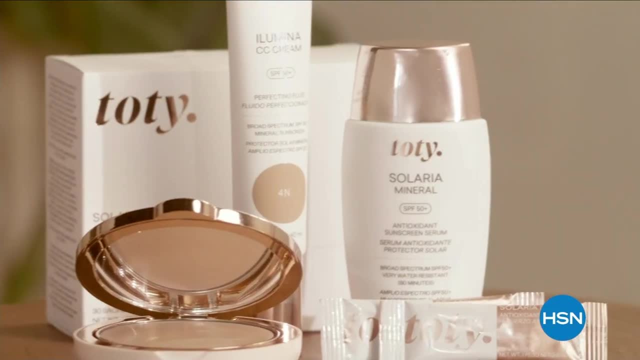 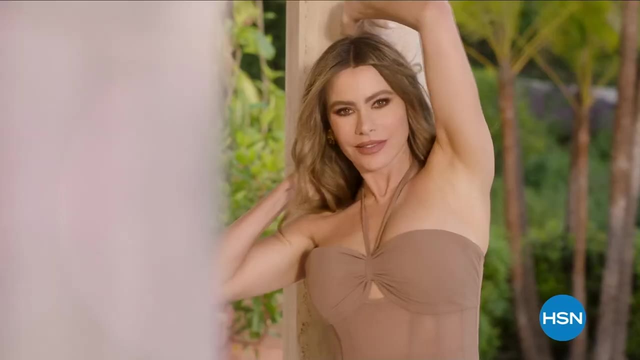 We're going to help You. send flowers for an incredible price. Don't go away. I am Sophia Vergara and I am so excited to introduce you to Toti, my new range of advanced sun care. Made to protect your skin from photo aging and visible signs of sun damage, Toti is designed to enhance your belleza. 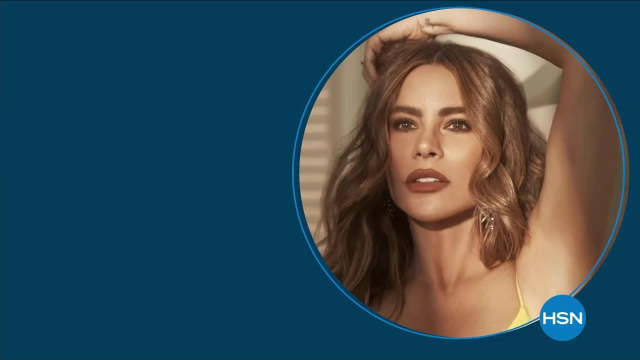 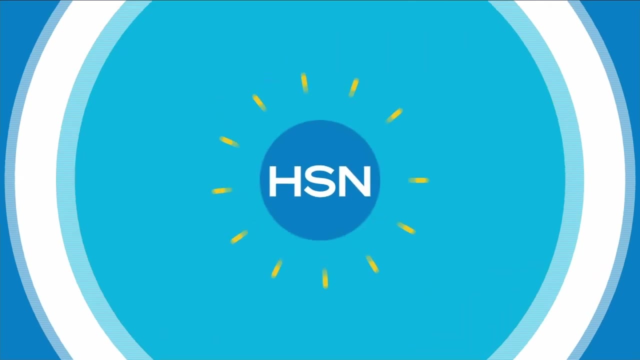 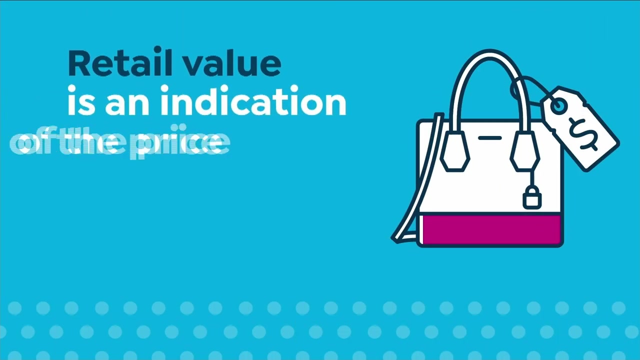 Become your most beautiful you with Toti Watch. Toti Toti by Sophia Vergara. Only on HSN. Here at HSN, we base our retail values on nationwide information. Retail value is an indication of the price you would expect to pay for the same or similar item elsewhere. 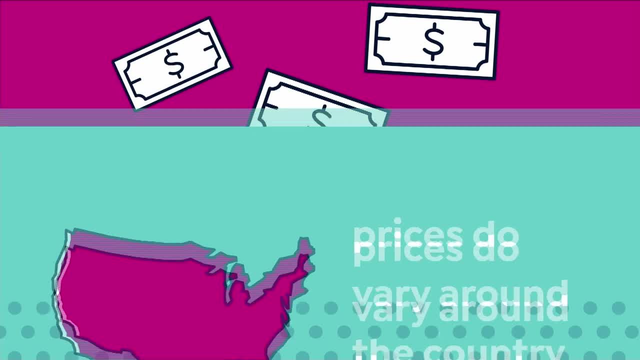 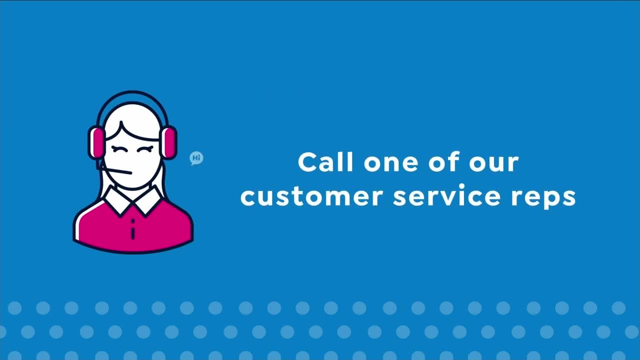 Not the price at which you would be able to sell the item. Prices do vary around the country, so ours might be different from prices in your area. For more information, call one of our customer service reps at 1-800-788-7888.. 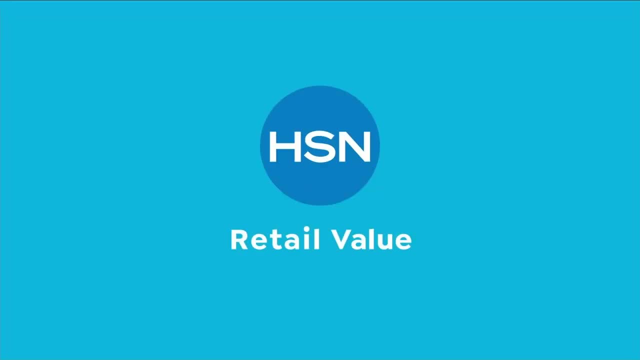 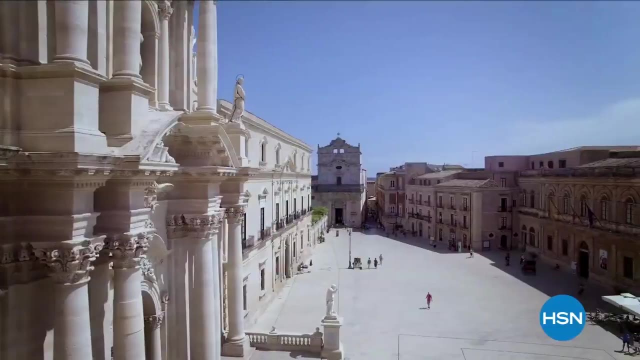 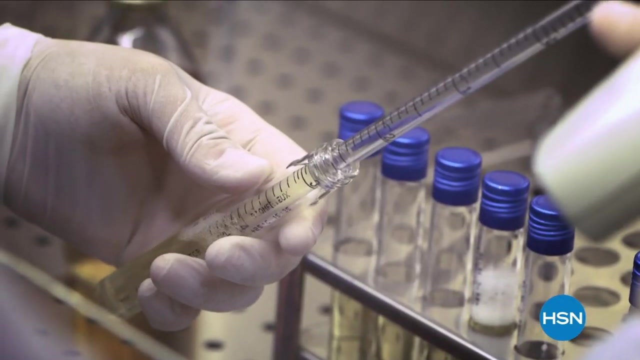 Or call 1-800-384-3900.. Perlier is an Italian bath and body company rich in history and tradition, Never far from where it started. Perlier is old world skills mixed with modern day science, Driven by a focus to treat skin with the best ingredients. 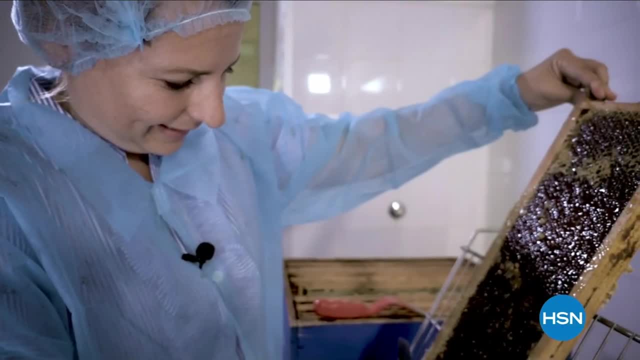 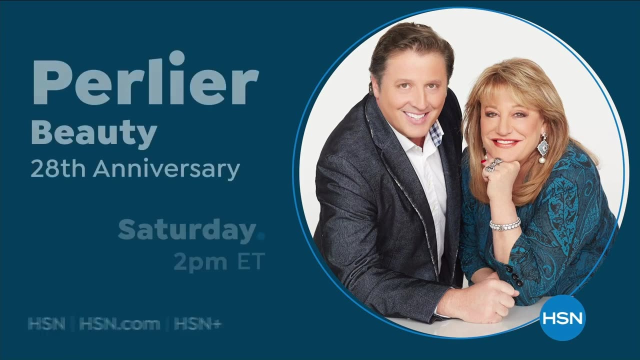 Perlier continues to develop innovative new lines while staying true to its culture. Discover luxurious bath and body products. Perlier is a product of Perlier. Perlier is a product of Perlier. body rituals from Italian Botanical Gardens with Perlier. 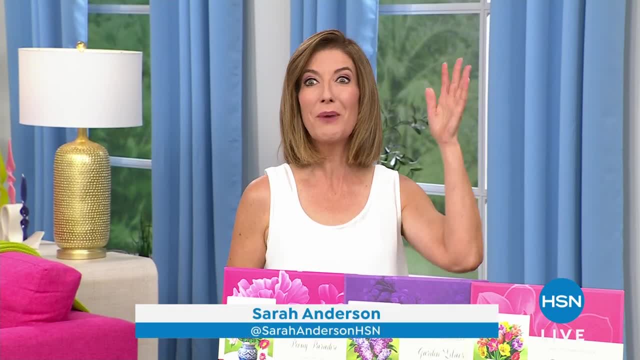 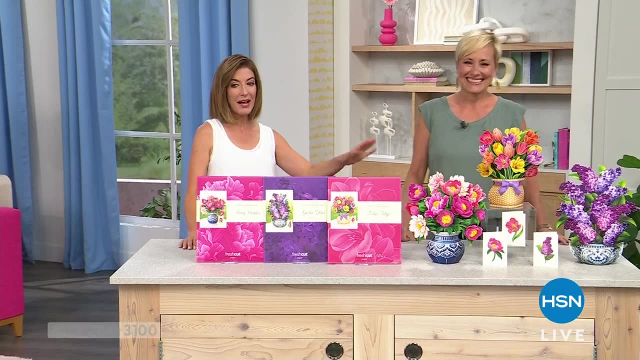 Oh, so nice to be back with you. Would you like another weekly deal drop? This is why you watch Tuesdays. We're here every Tuesday night. You're watching What a Girl Wants. Leslie Bracken is here and we're going to jump right in, because you have to see this to believe it. These are the very 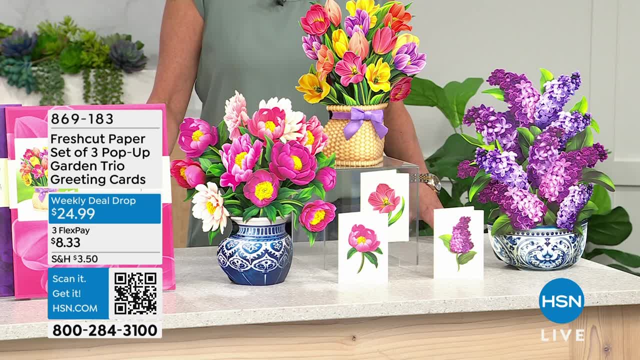 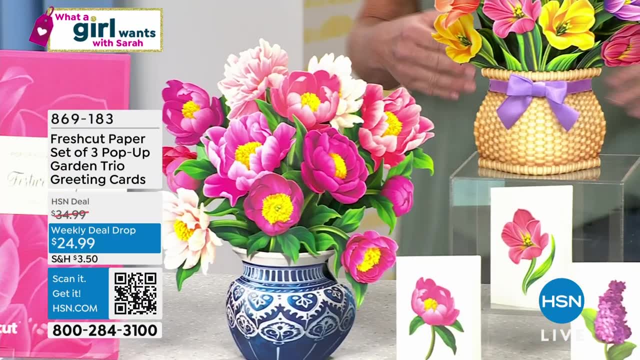 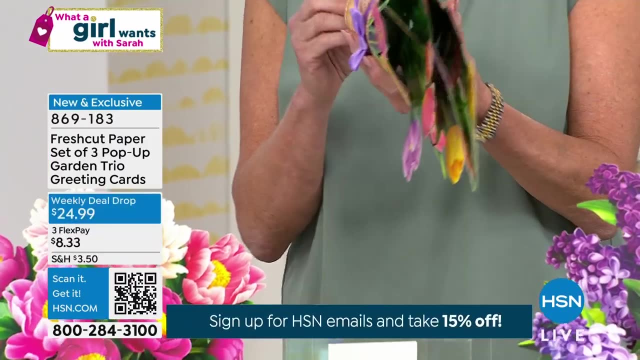 popular fresh cut paper pop-up cards. Every time they're here they sell out and we have a new trio tonight. We do. We have a new trio, Absolutely, And this is kind of our essence of spring. I love it. We call these pop-up cards because they do pop up. These are all popped up here. 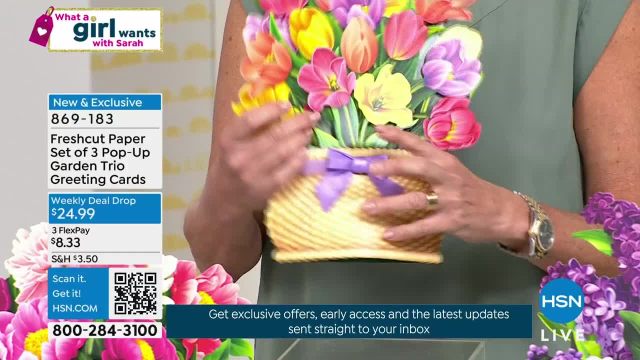 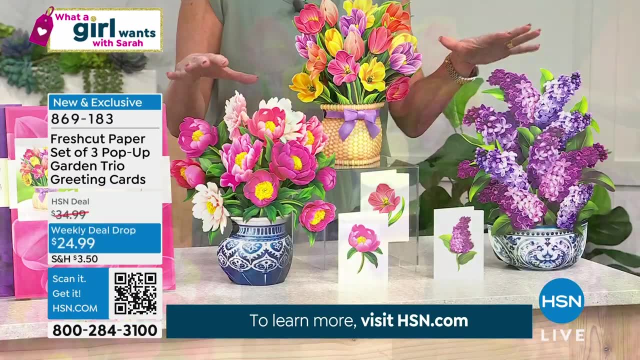 for you and they just kind of fold flat. So if your recipient wants to store these and put them away, they can. Or if you're giving them to yourself, that's possible too. But you're getting all three of these bouquets. They're really. 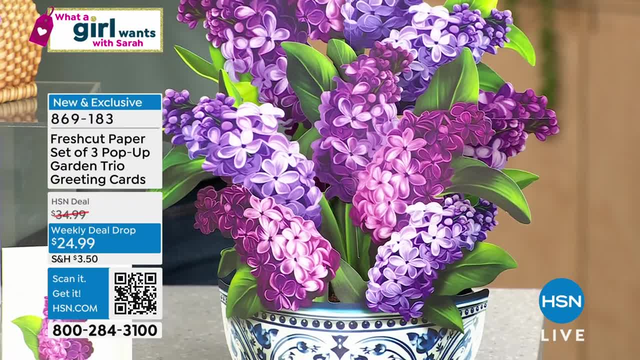 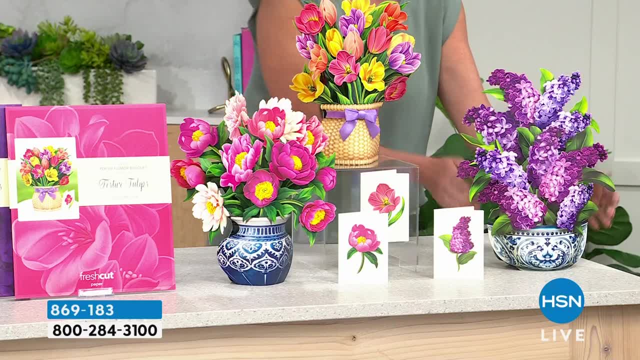 a pop-up bouquet, You're getting these wonderful tulips. Oh, we're going to go right there to the lilacs, which are just lush. They're standing about 14 inches high and 10 and a half inches wide, So they have real like dimension and depth. They have a wonderful luminous purple quality to 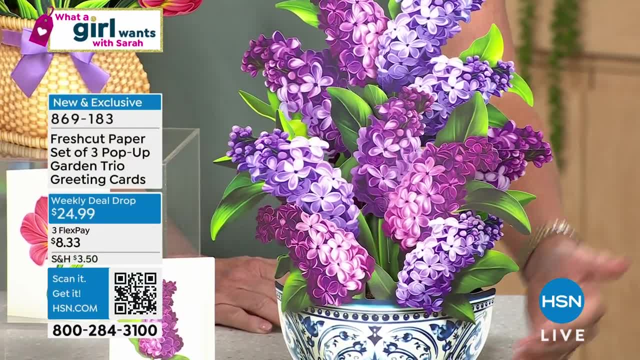 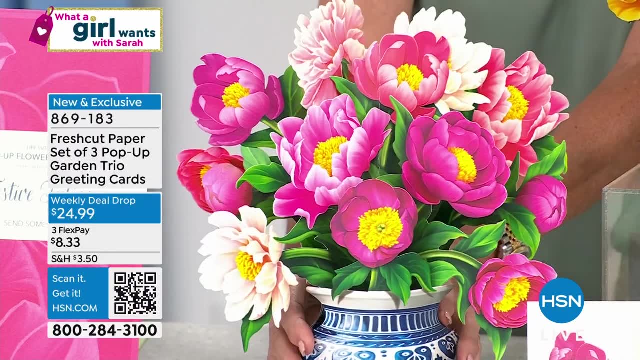 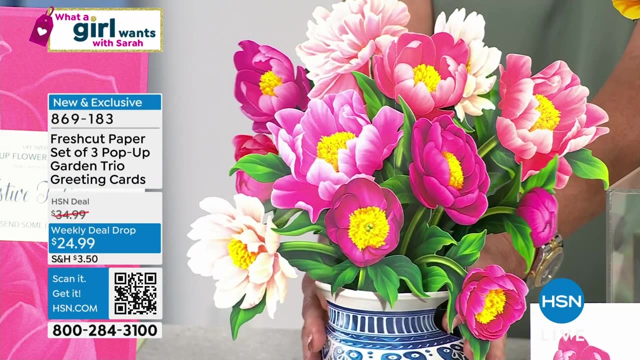 them and this great indigo and white porcelain bowl. Then you also have over here these really bright and bountiful peonies. I love how these can just add color to anywhere you want to put them. They also are in an indigo and white, but more of a vase or a pot. that's kind of French. 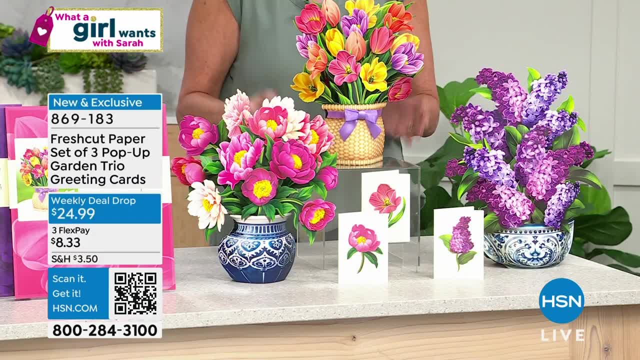 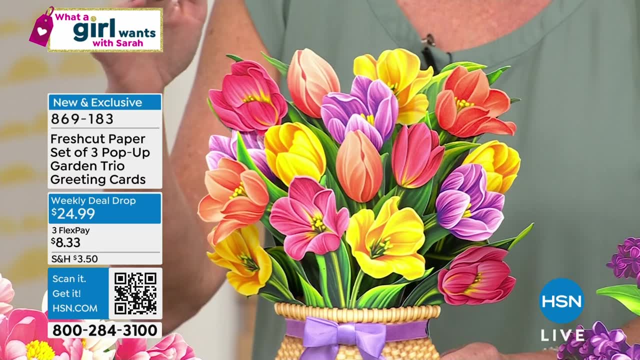 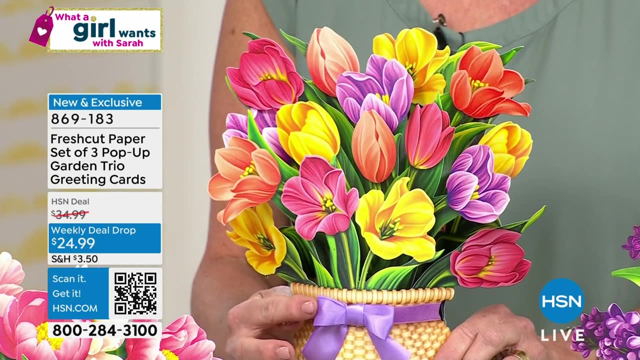 countryside. And then these tulips- which, by the way, are my favorite flower- truly are the essence of spring. You're getting this great spring color palette of lavenders and yellows and corals And they're in this really sweet basket with this wonderful little satin lavender bow, And this one's 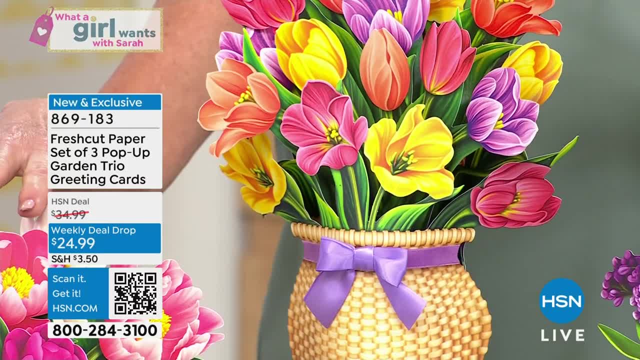 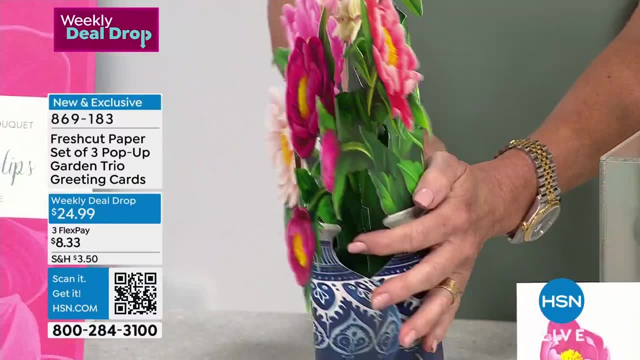 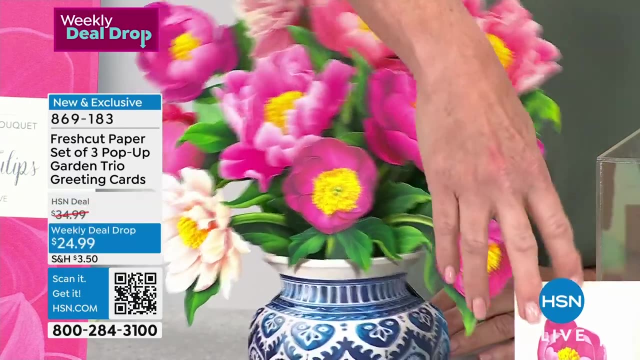 about 12 inches by nine inches, And then the peonies are 13 by 12.. So you're getting a real substantial gift here that pops up. It's all three dimensional. The colors are just spectacular. Each one of these has a card, a blank note card that matches back to them. So this is any. 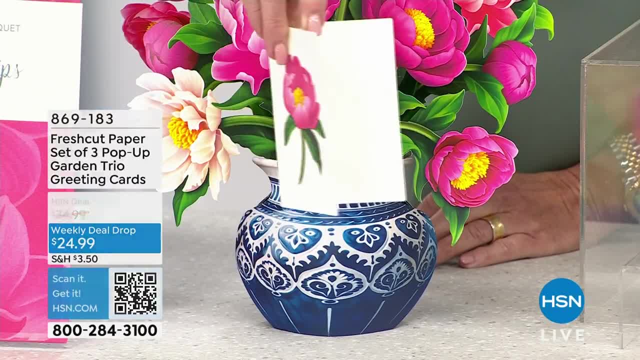 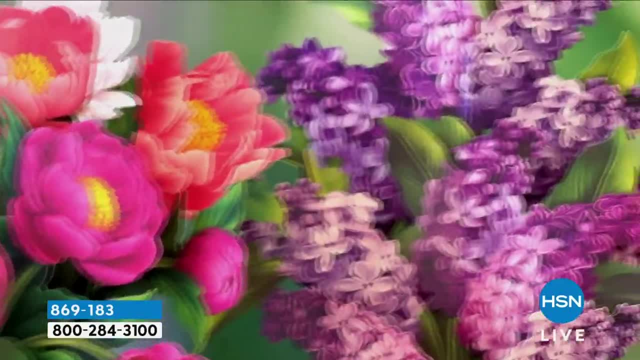 sentiment that you want. This is: thank you, thinking of you, feel better, happy birthday, happy anniversary, happy graduation. And there you see the lovely envelopes that they also match back to. So they're coming or going to your recipient, And I mean a spectacular little piece of jewelry. 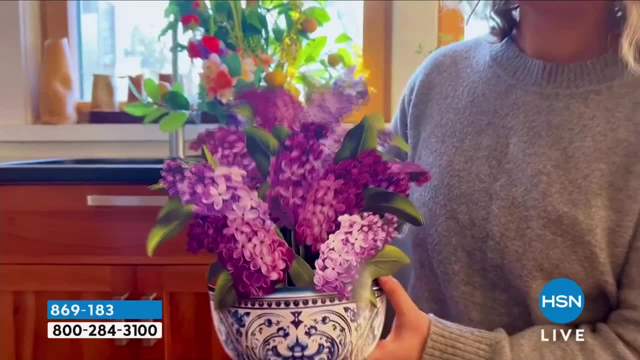 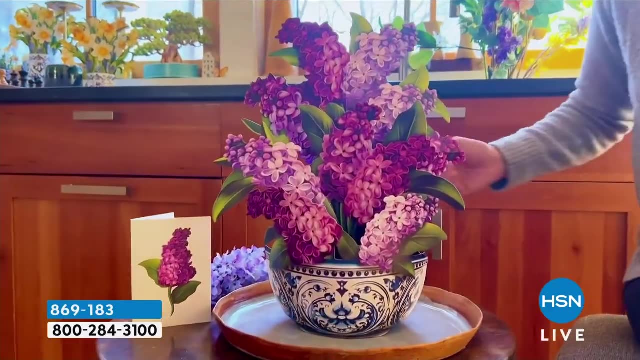 And it's only four forever stamps to send them. So it's stamps you already have in your drawer to send this incredible gift to someone And that's what you're getting. You're getting three beautiful bouquets. You're getting three of the greeting cards. 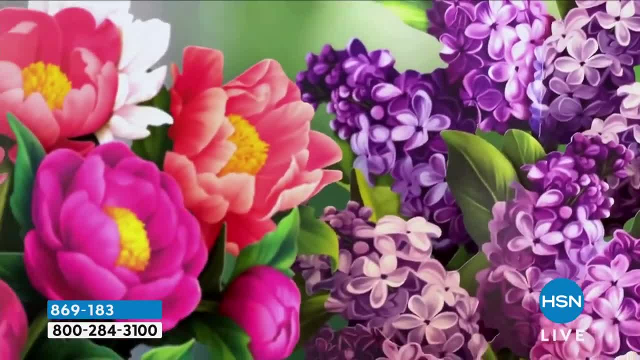 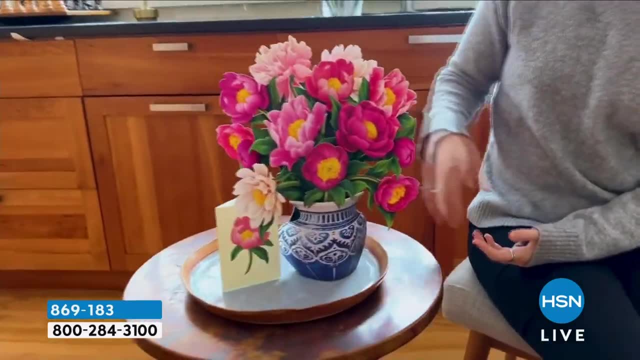 You're getting three of the envelopes. You have everything you need to send them And back by popular demand. you have been loving the peonies, So we're so glad we brought that back. This is the first time you're seeing the guarded lilacs. 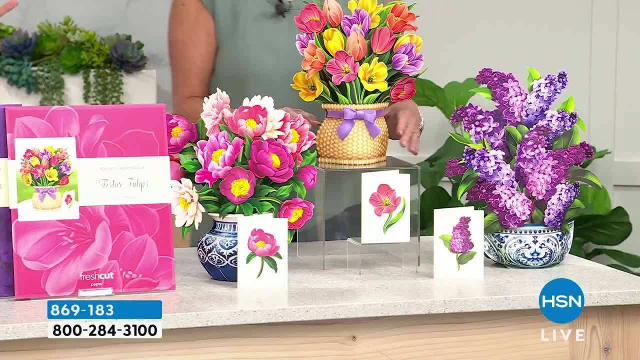 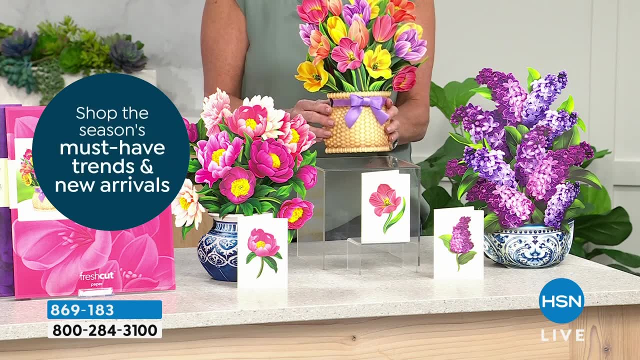 It's the first time you're seeing the tulips, And if you've ever tried to send flowers, well, let me tell you they're pretty expensive to send fresh flowers. You'll easily spend a hundred dollars just for a few dozen flowers. 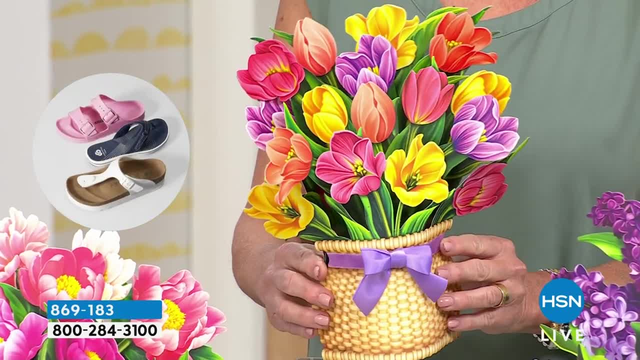 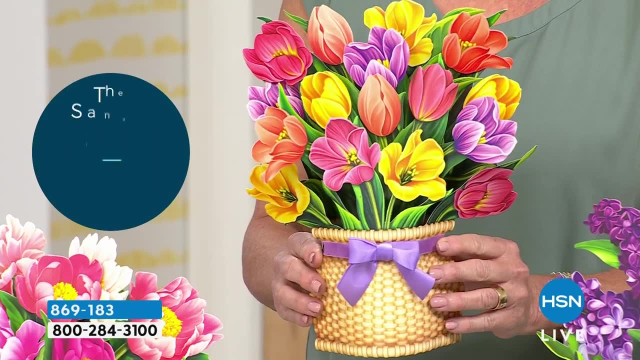 You could spend $50 a pop, and then you'll have to pay delivery fees. This is like sending a bouquet of flowers that won't wilt, that won't die. You don't have to worry about fragrance, You don't have to worry about bugs, You don't have to worry. 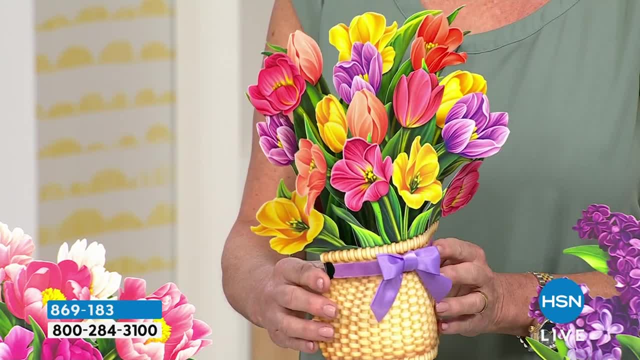 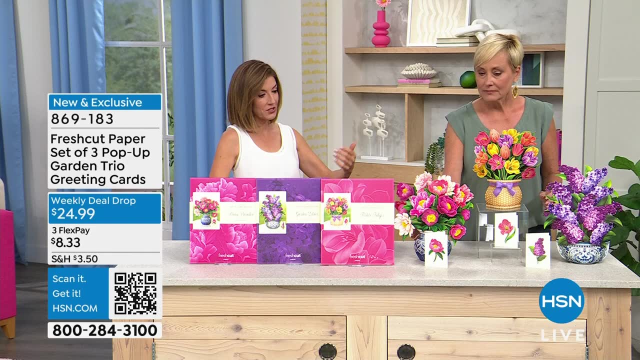 about how they're going to look when they arrive. And if somebody loves the idea of flowers but maybe they can't have flowers, fresh flowers, whether it's in their hospital room or in their assisted living, This is like sending someone a bouquet of flowers. This is their Mother's Day trio. You're the first to. 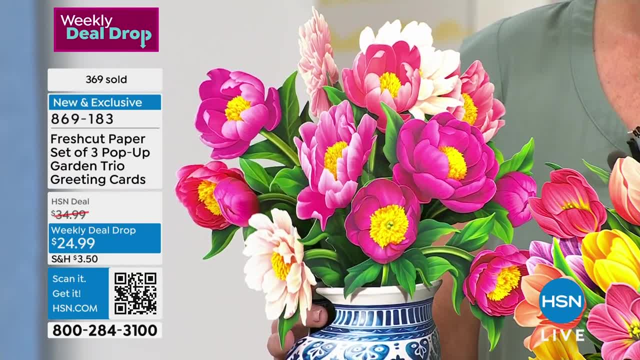 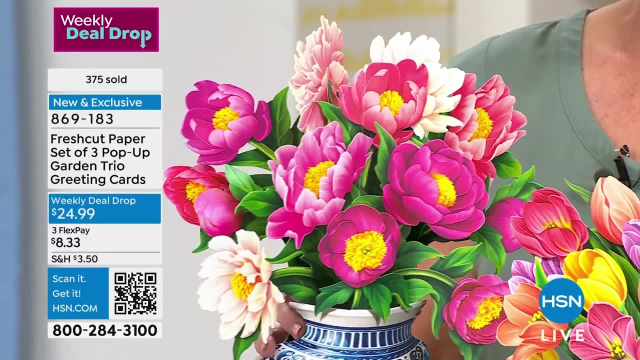 see our weekly deal drop. They sell out every single time they're on air here at HSN, So jump right in. We'd love to get these out to you 869-183.. But I'm sure people just rave about them. They're always customer picks. I can't remember if we've ever done a weekly deal drop. 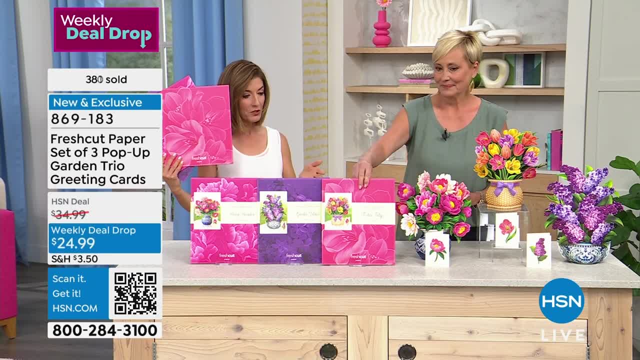 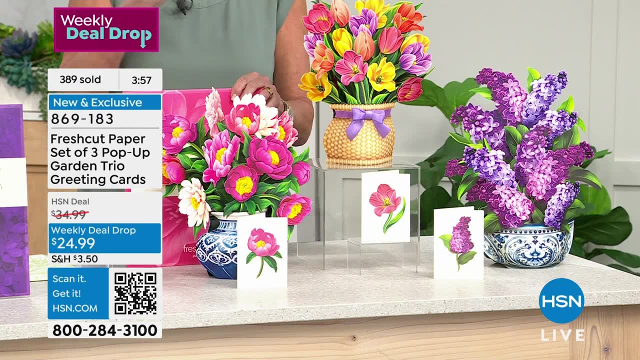 where you get such a great value and all you do is place them in the mail yourself. So you mail them to who you want, when you want. Or you can just hand them right to yourself, Or you can hand them. In fact, I actually was at a baby shower. Give yourself a bouquet of flowers, So tulips. 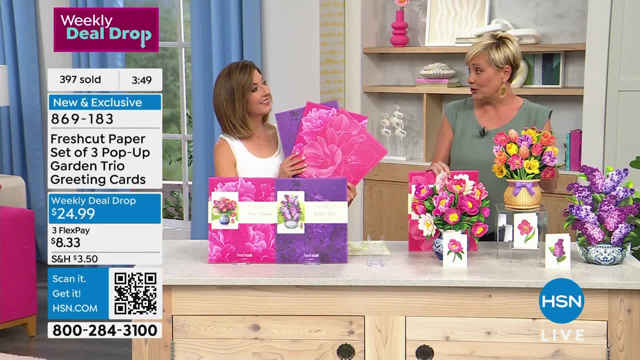 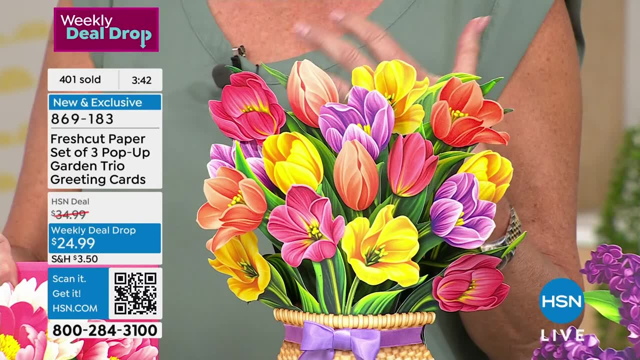 by the way, represent. they symbolize unconditional love and new beginnings. I actually just gave these at a baby shower the other day And let me tell you, the entire room went: oh, that is so cool. In fact, 15 years I've been here and I have brought you all kinds of home stuff. 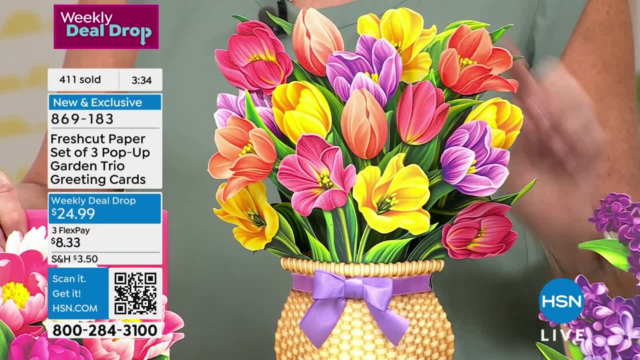 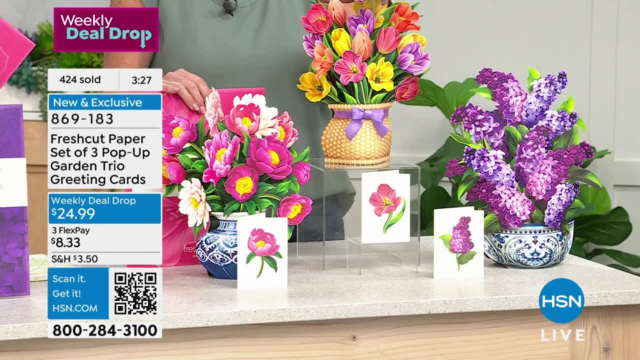 And even some crafting. This is the one table when I have fresh cut paper that everybody wants to come and touch and look at, Because you're really getting just spectacular. So these are. the tulips are symbolized, like I said, new beginnings, unconditional love. So think of. 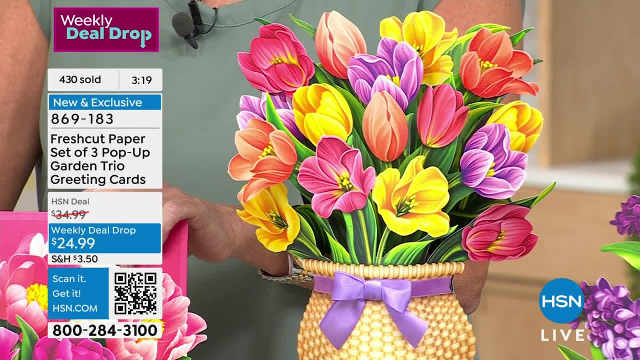 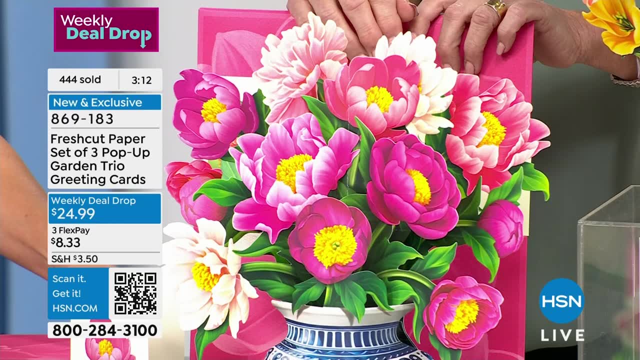 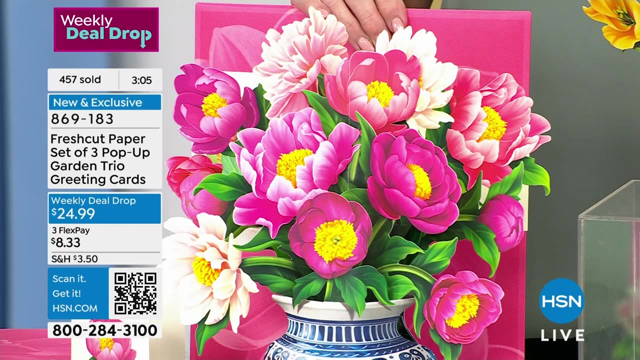 those people that you want to give unconditional love to. You want to celebrate new beginnings. The peonies- these represent beauty and bliss. So again, think about really good celebration. It's graduation season coming up, It is Mother's Day coming up, It's teacher appreciation also next month. So these are 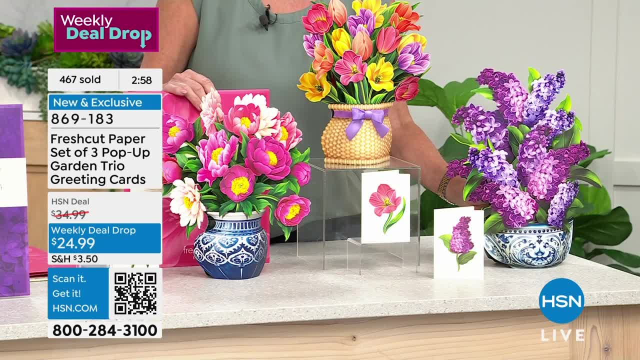 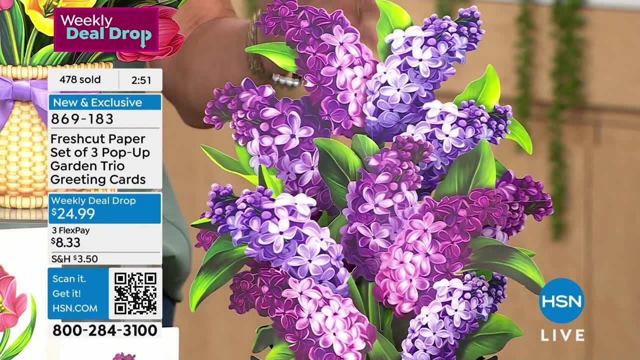 great flowers to give. And then lilacs. I like that you mentioned fragrance, Because lilacs can have fresh lilacs can have a very intense fragrance Fragrance. It can be a little bit harsh, But you're getting all three of these. I can't stress enough: All three of these you're getting. 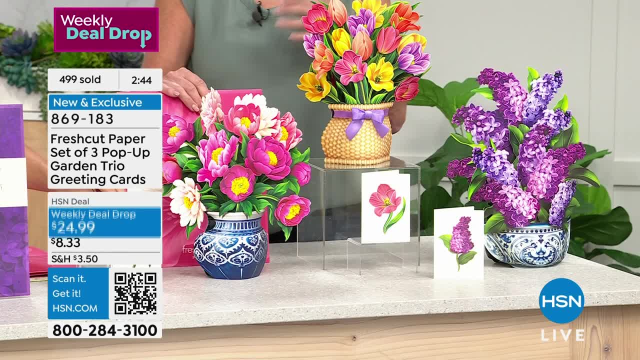 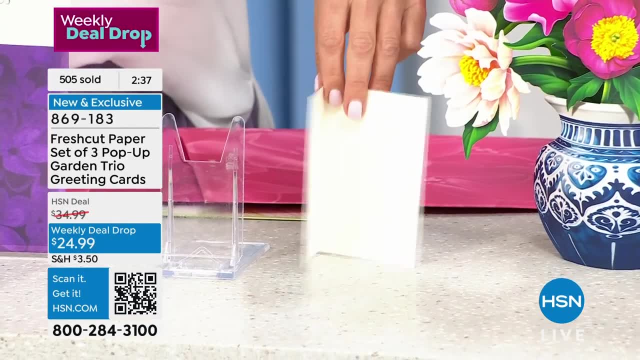 for what is it like? just over $8 a card, $8 a piece, And then you're also getting three of the cards. So you're really getting a bouquet times three. You're getting the reading cards times three, And then you're getting the giant, beautiful, I mean even the. 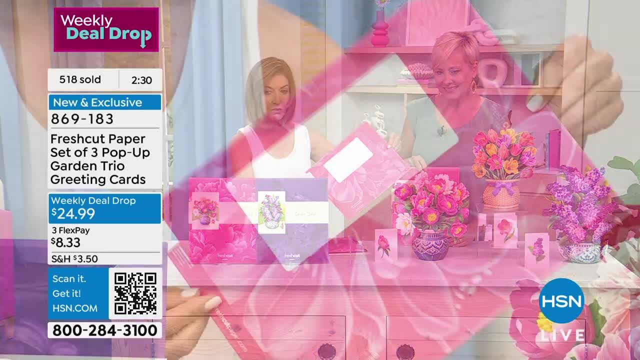 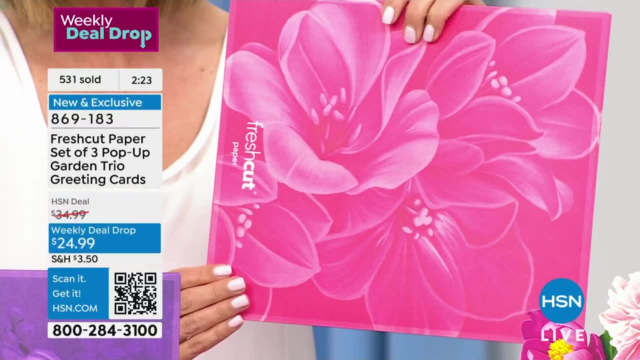 envelopes are so gorgeous, They're going to know they're getting something special. You get three of these. You put on four of the stamps that you already have at home, You pop it in the mail, and they're going to be so thrilled to receive these gifts. Here's what's going to happen, though These. 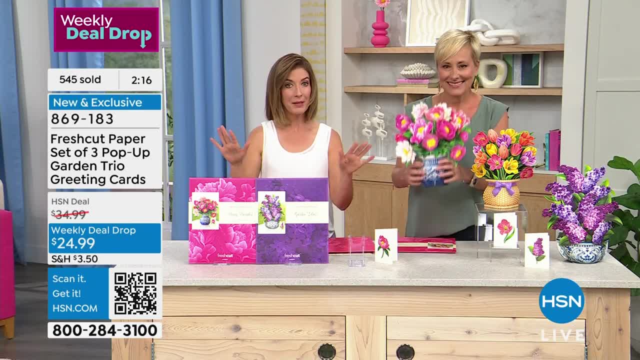 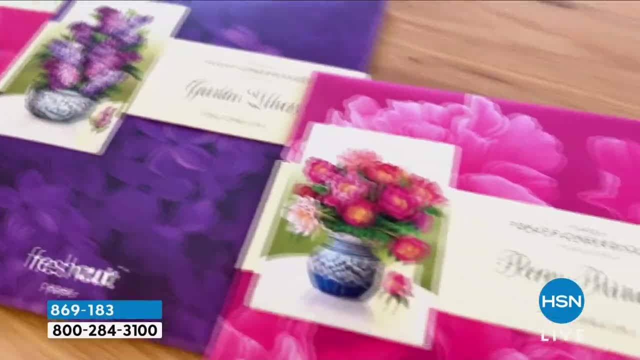 are going to go very, very quickly. Order a couple sets Might not be a bad idea. I love that you mentioned the end of the school year. You want to do something for teachers. Also, even if you have a friend who's probably having her baby right now in the hospital, I would love to send her. 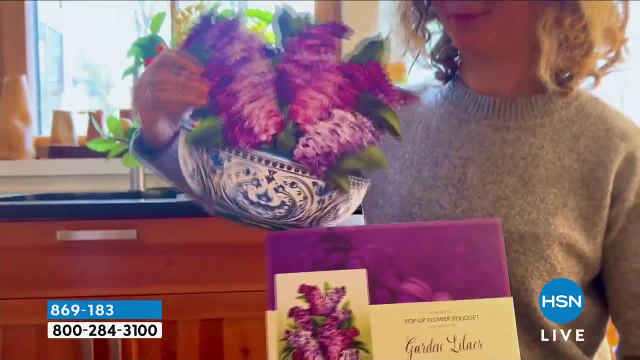 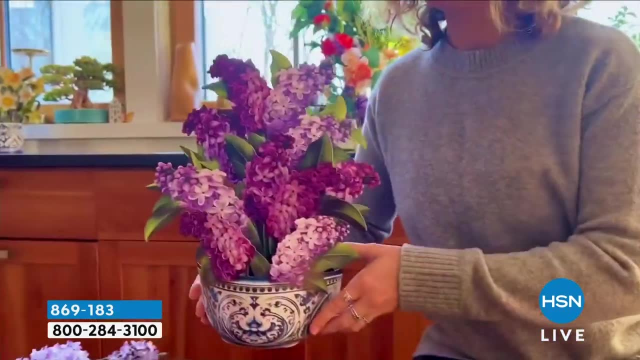 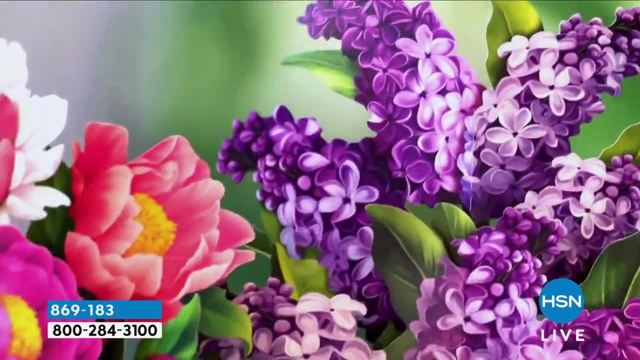 fresh flowers, But I thought, but then she's going to have to bring home a vase and water and a baby and all the stuff from the hospital, And this you could actually pack flat and then you can pop it up again when you get home to your destination. Look at how lifelike they look, three-dimensional. 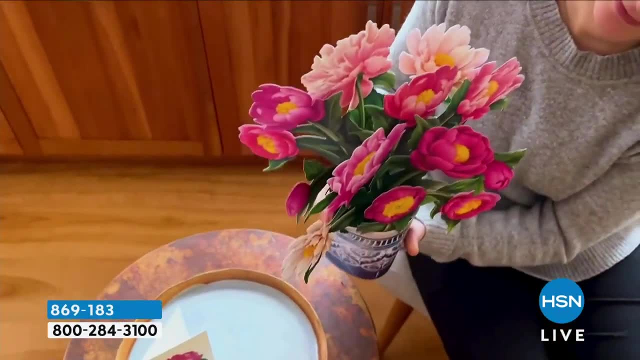 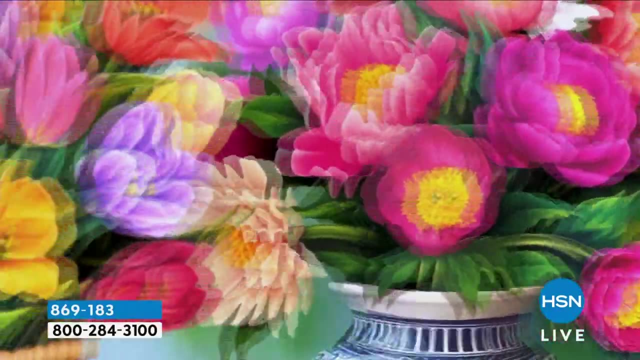 from across the room. It looks like they're in a real vase. It looks like they're in a real basket. It looks like they're in a real beautiful, gorgeous China jar. that looks like they're in porcelain. Leslie, Absolutely, They are life size and lifelike and they really are little works of. 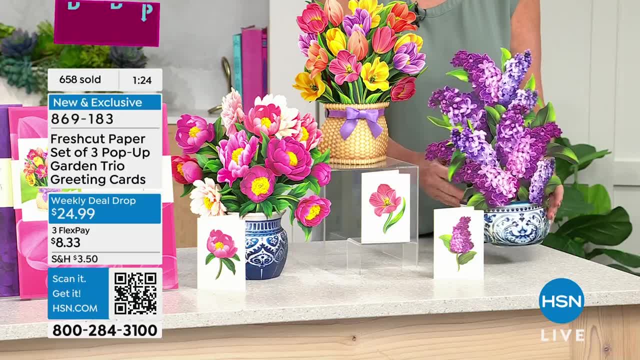 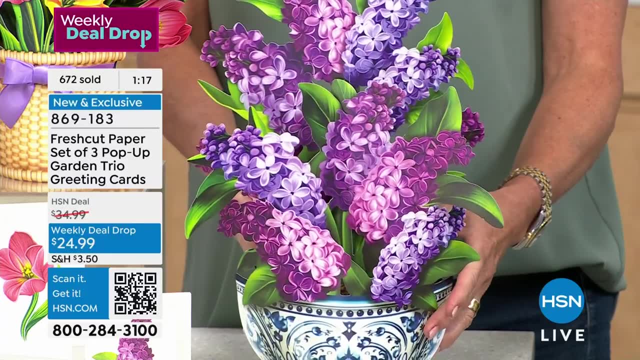 art. I mean, you can see and please do. This is our the first time that we're coming here with this bundle, with this trio, but we have brought you fresh cut paper before And please do go look at the other trio, the other bundles, and look at the reviews, because what you will see- time and 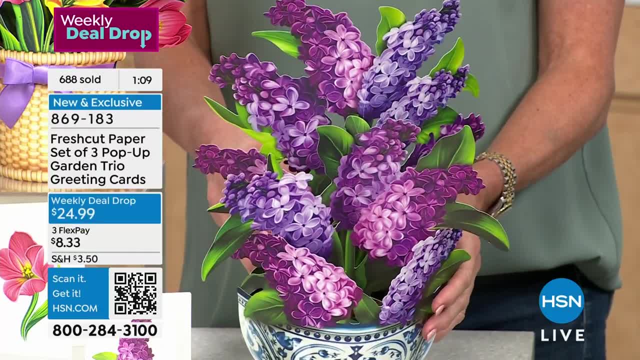 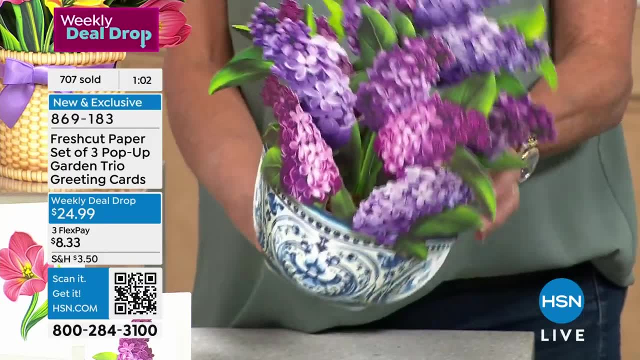 time again is: they looked great on TV. They look even better in person. The people that have purchased them have been wowed by the way that they look, and the people that they have given them to have been wowed by the way that they look. And remember: you are actually. 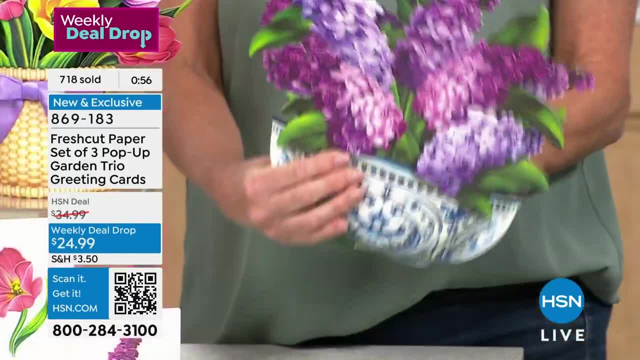 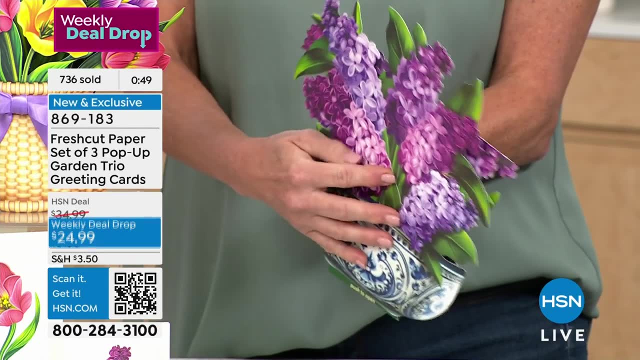 shipping this flat. It just folds down. This one actually folds two ways. right here It folds completely flat. So if you were the one that received this, or if you've given it to yourself- cause that's okay too- you can actually put this away and bring it back out for the season, Like. 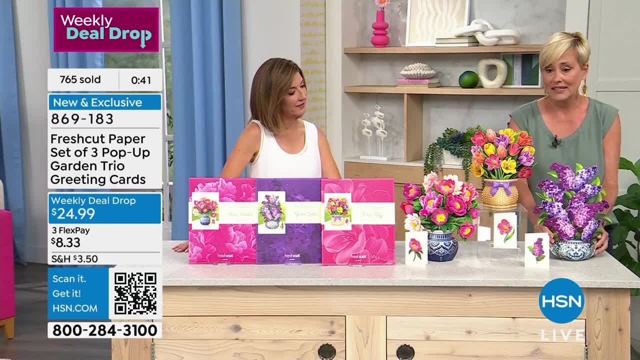 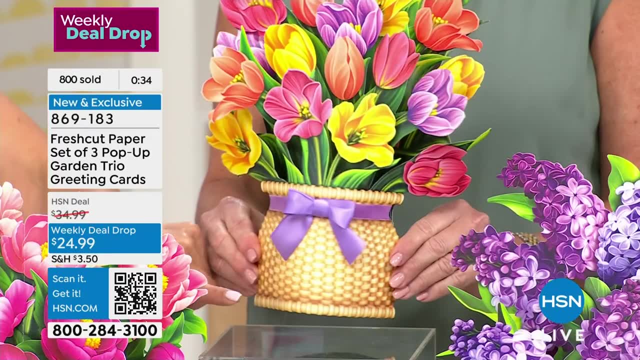 for instance, tulips- really again essence of spring. If you want these out like as Easter or spring, this looks like a basket. If you weren't here in the studio and coming over and touching it, it looks like a basket. Let's talk about the artist. 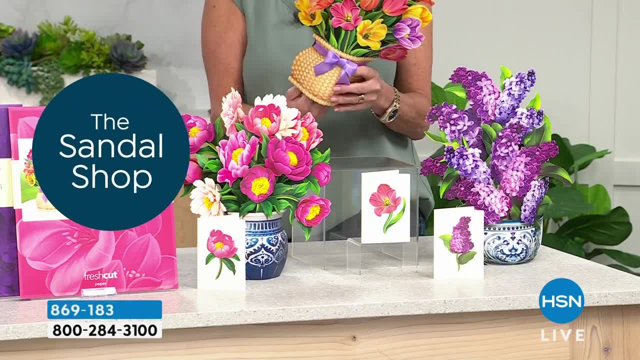 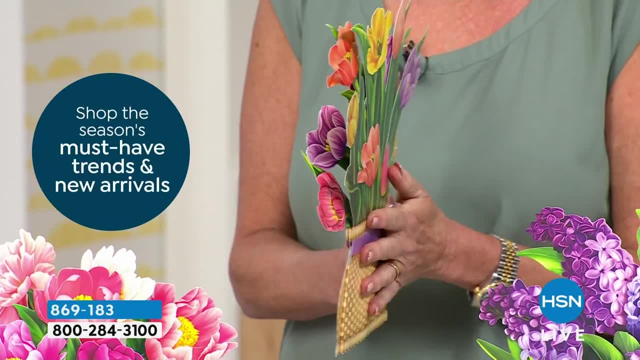 Yeah, So Peter Hewitt is the artist and designer of all of these, And he actually started this about four years ago, right in the midst of COVID, because we couldn't send fresh flowers. There was, you know, lots of people that weren't doing well, lots of people that were suffering or that they 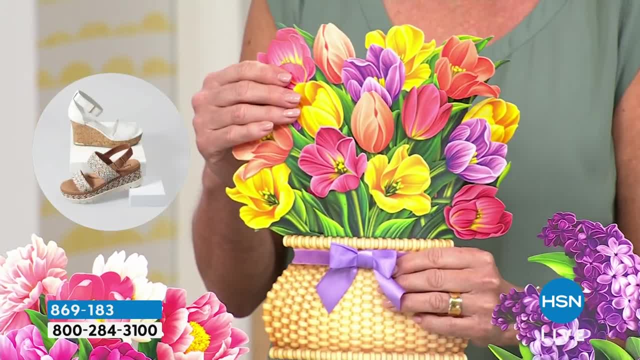 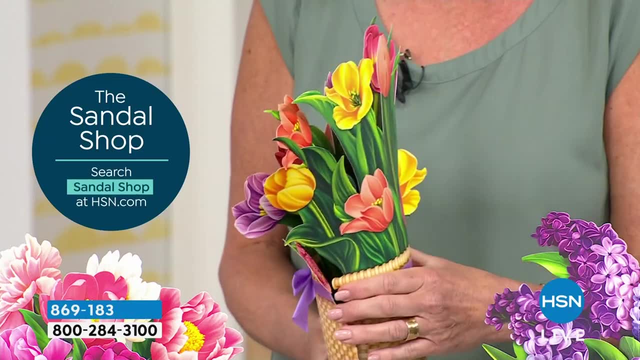 were lonely or isolated, And so you and we couldn't send flowers. And so he decided to find a way to send a basket of flowers. And so he decided to find a way to send a basket of flowers, All of the beauty and all of the drama of flowers and all of the sentiment of sending fresh flowers. 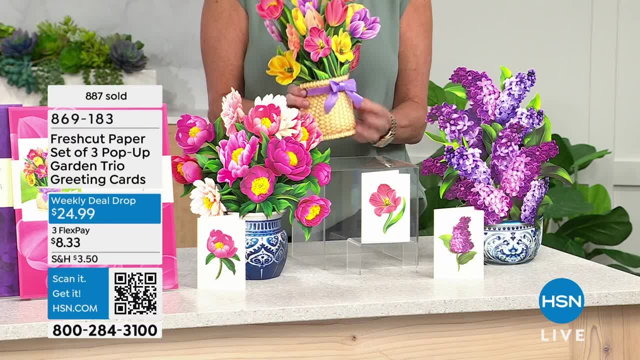 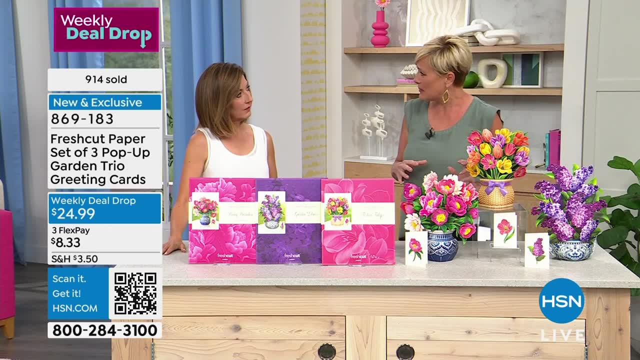 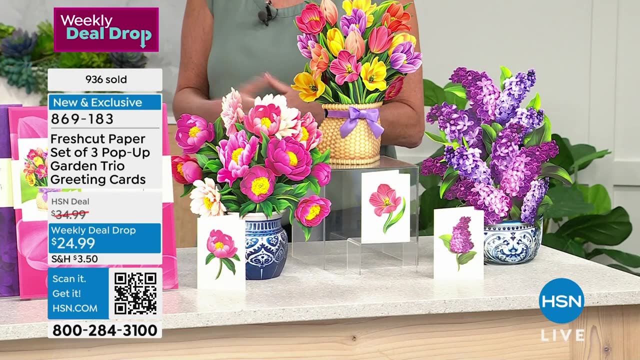 without the issues of delivery or the issues of allergies or being in critical care or the sadness of dying flowers. It's kind of sad when they die right, When they start falling apart and you're just throwing them away. These last and last forever. He's known for designs and decorations. 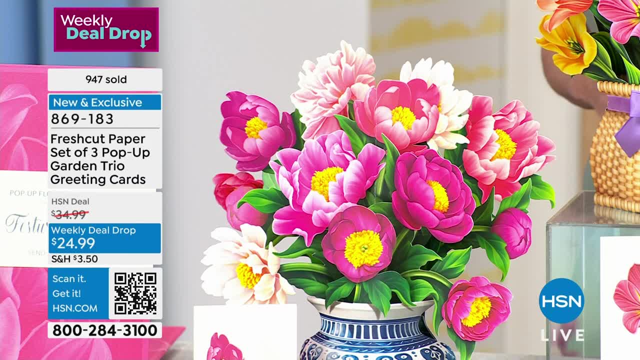 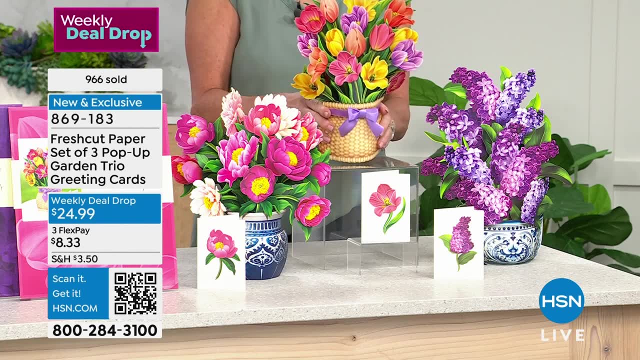 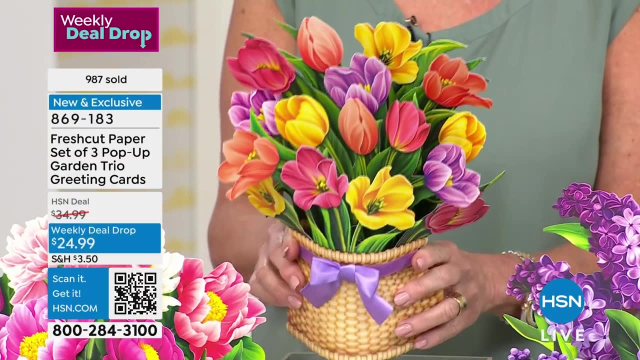 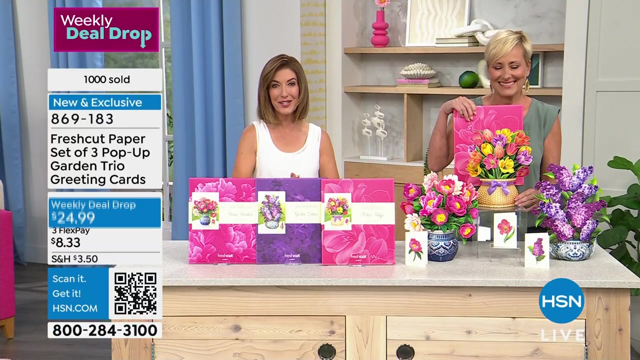 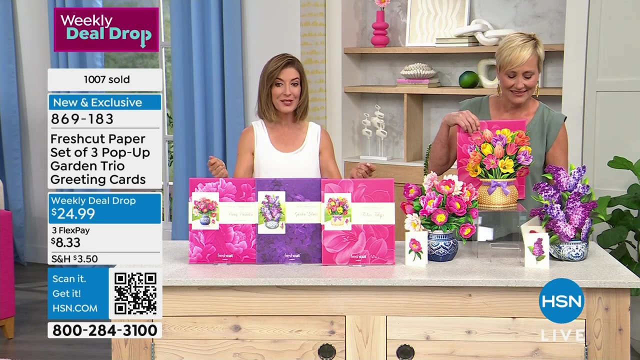 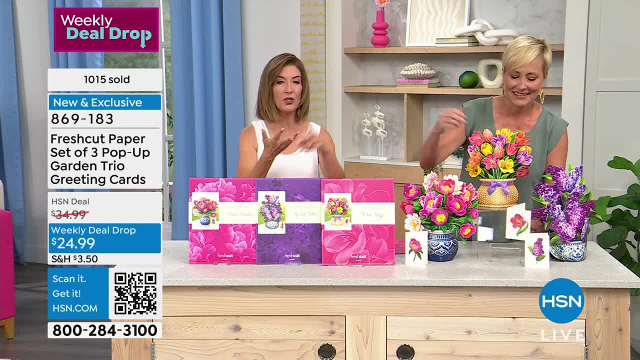 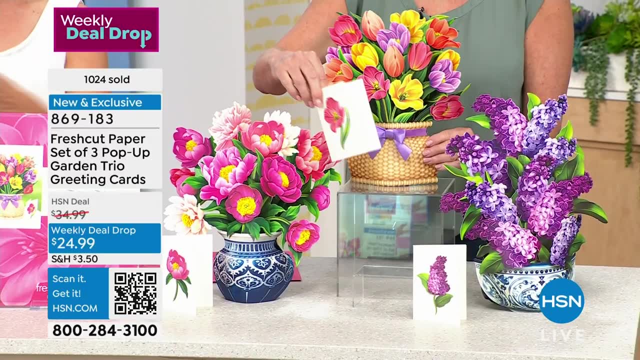 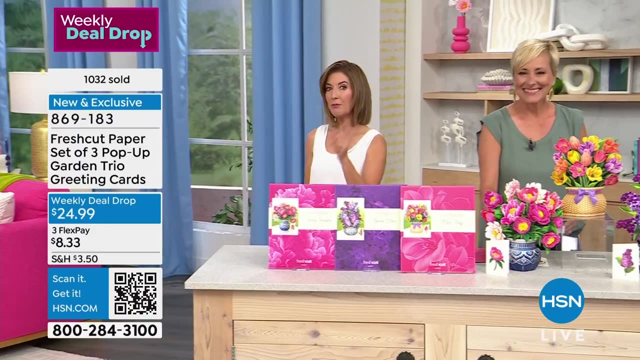 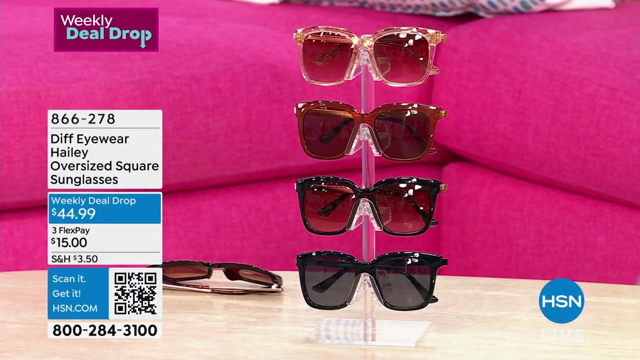 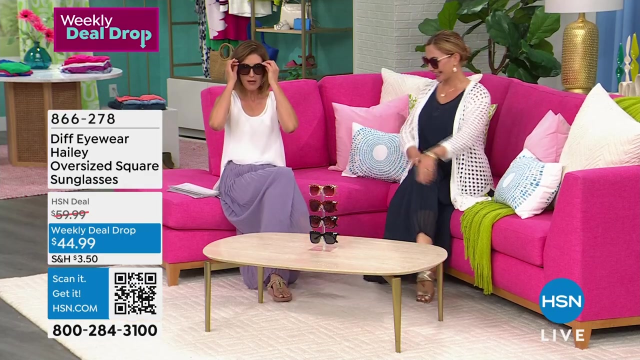 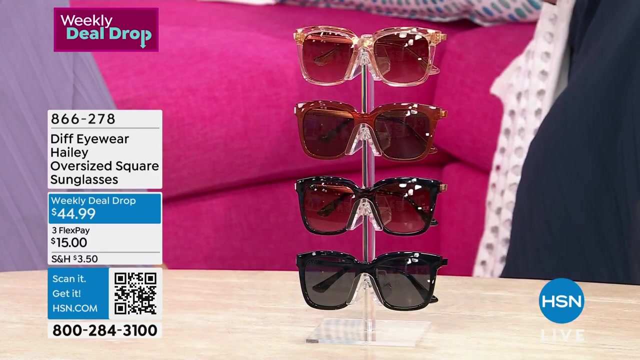 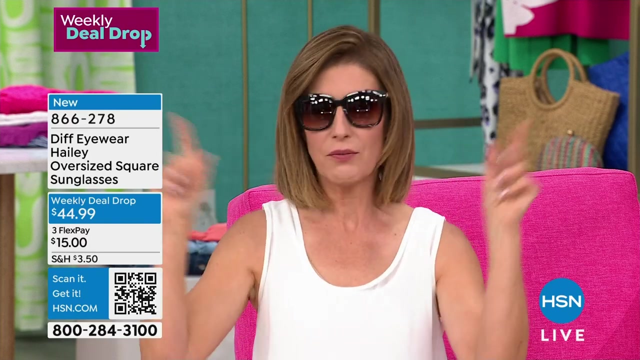 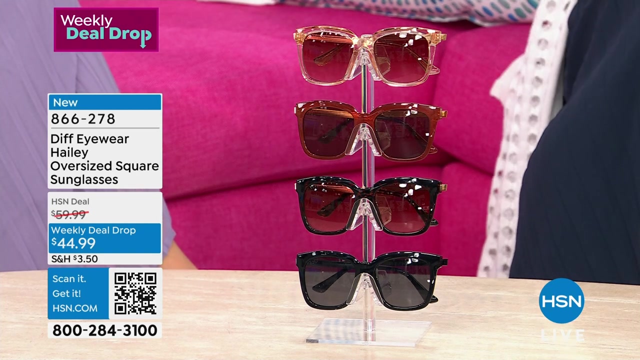 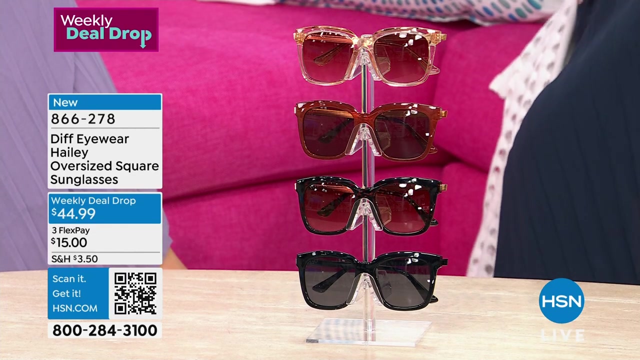 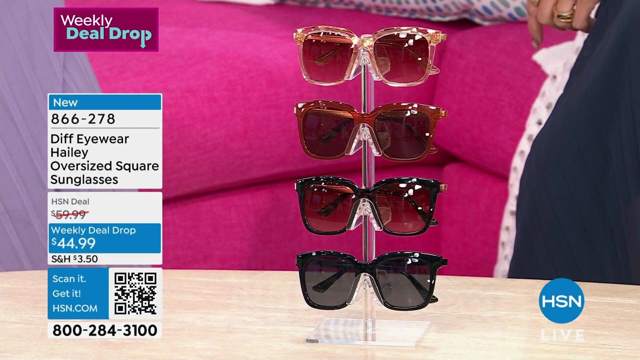 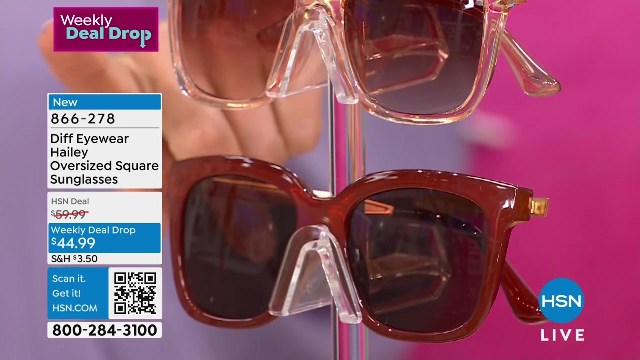 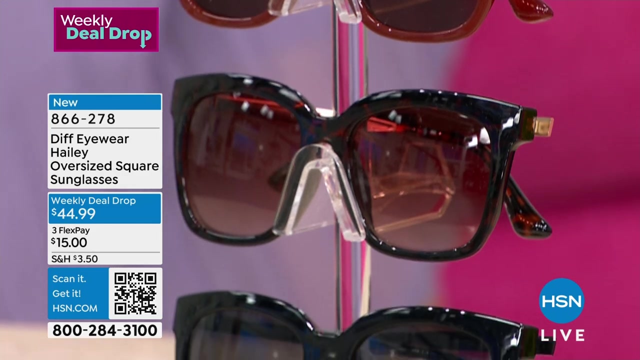 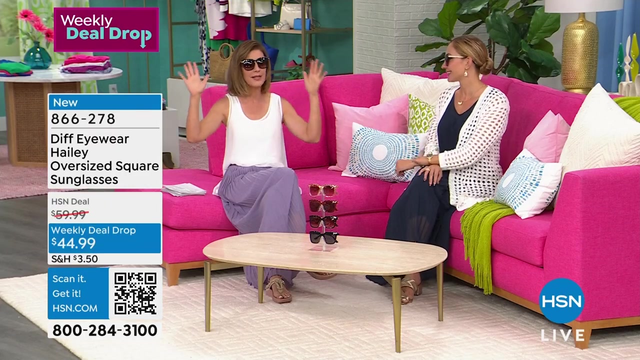 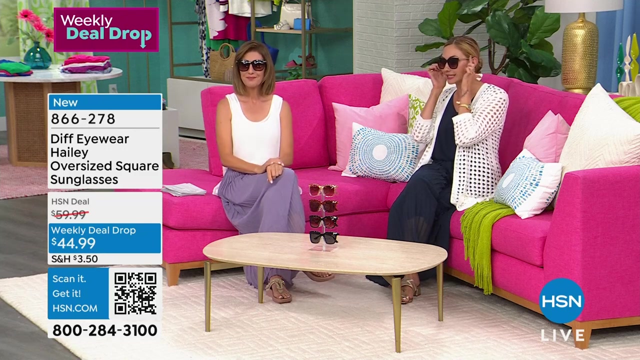 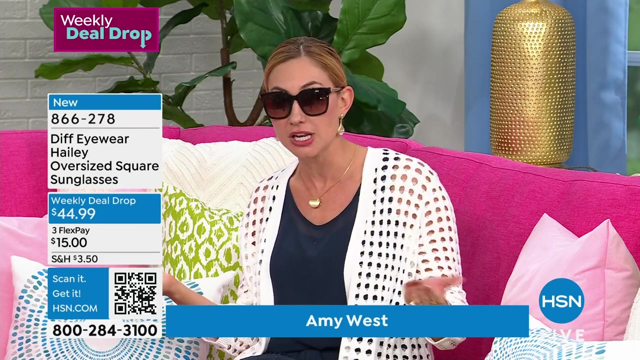 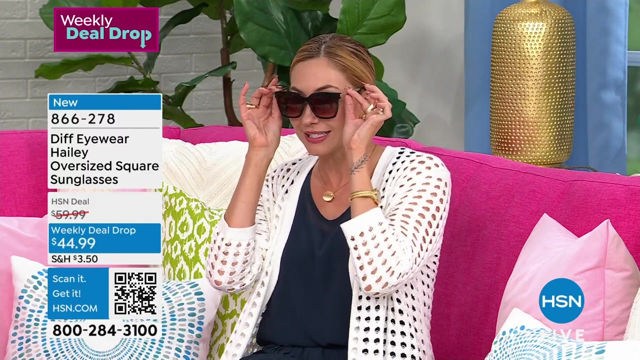 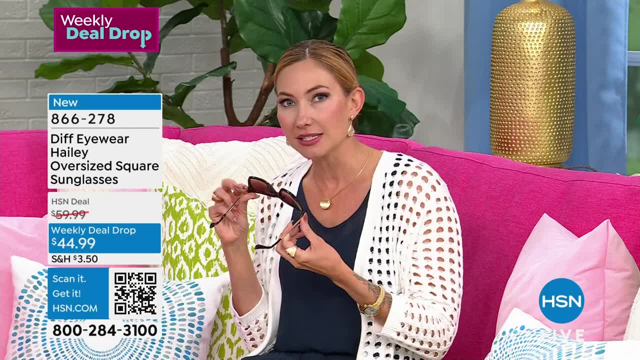 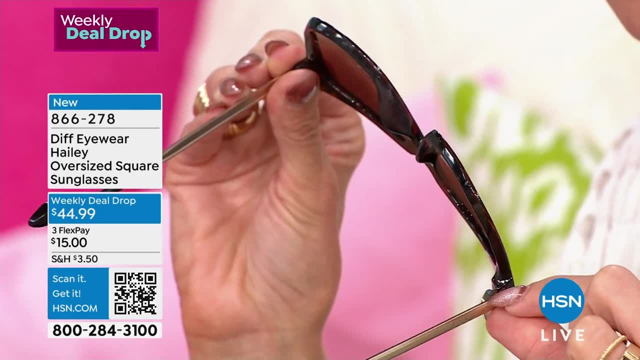 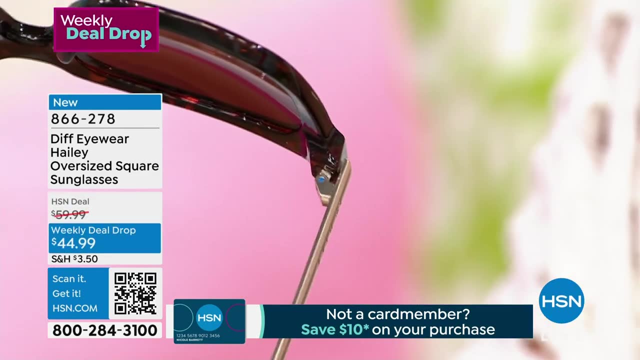 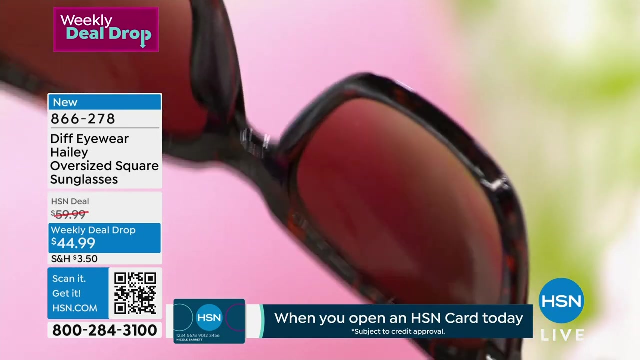 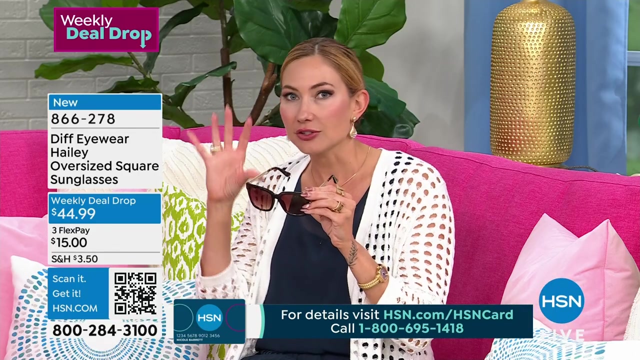 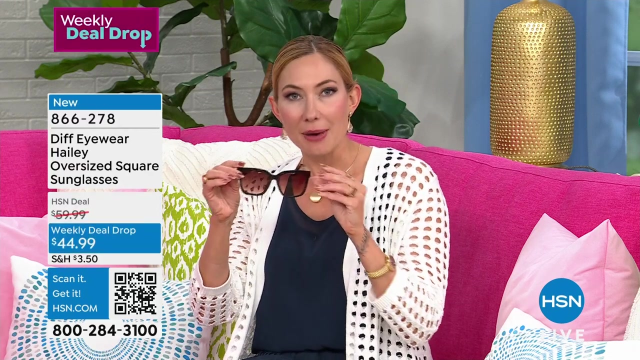 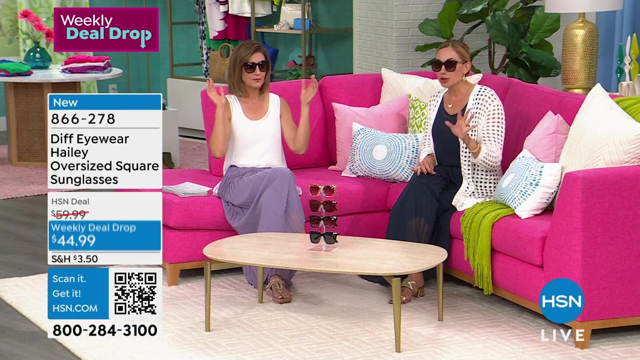 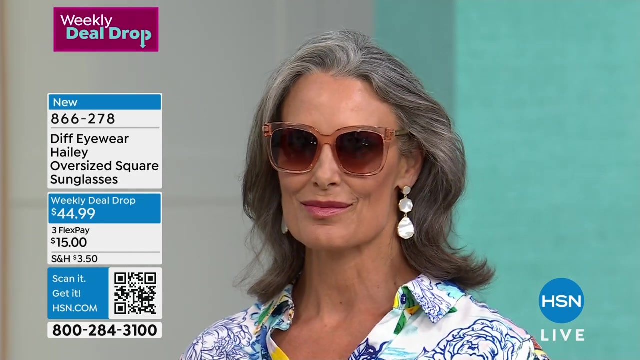 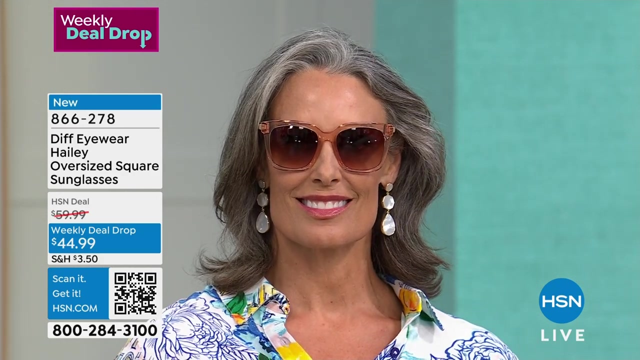 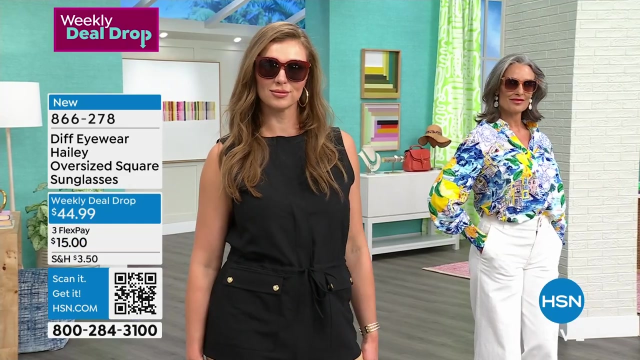 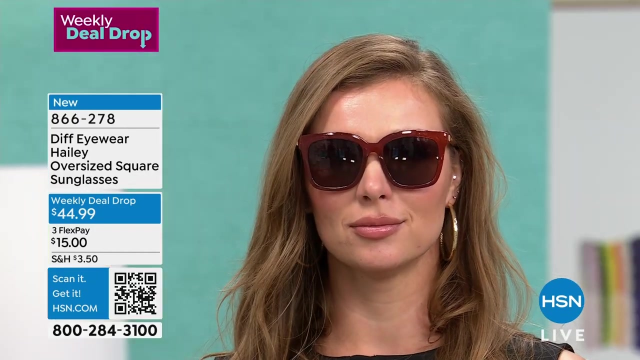 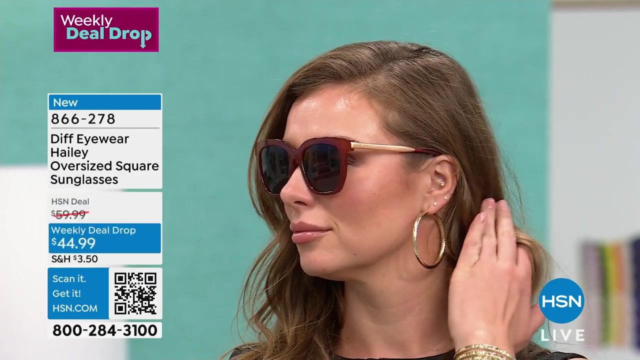 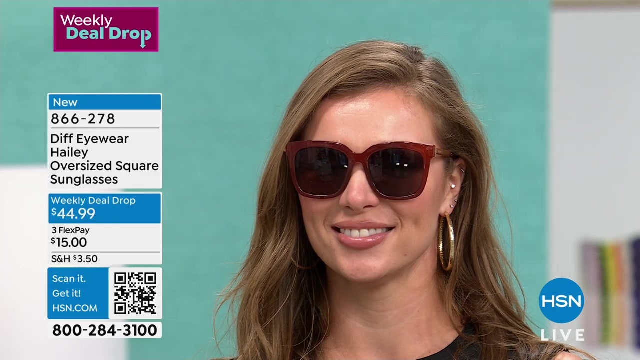 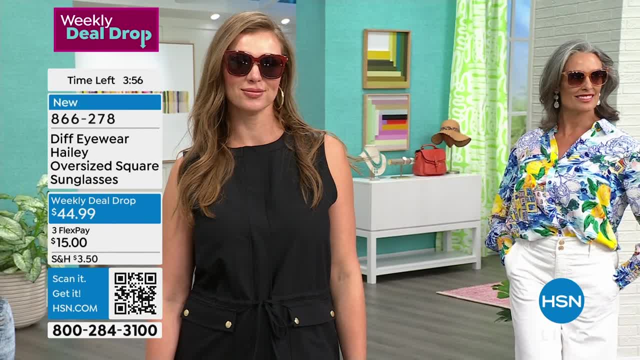 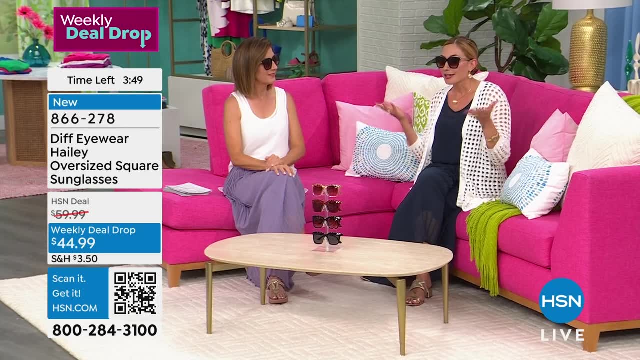 have actually benefited from the money and the efforts that DIFF has put into providing eye care and glasses to people, So over 4 million people. So I love that they have a mission and that they make a difference And at the same time you get to benefit from that affordable luxury and looking. so fashionable. Okay, let's go through the colors, because I know every time that DIFF has presented a weekly deal drop- and I don't think we've had one in a very long time- you're getting about a hundred dollar pair of glasses for over 50% off. We have the best price anywhere. These retail. 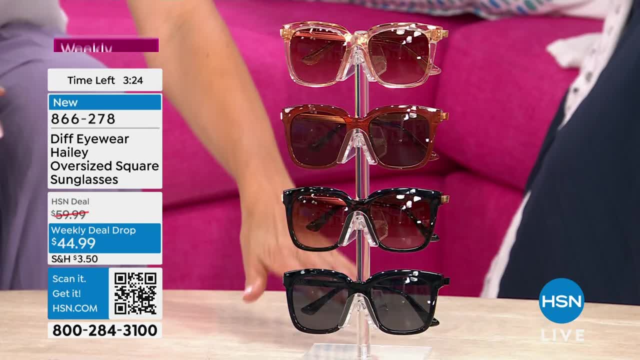 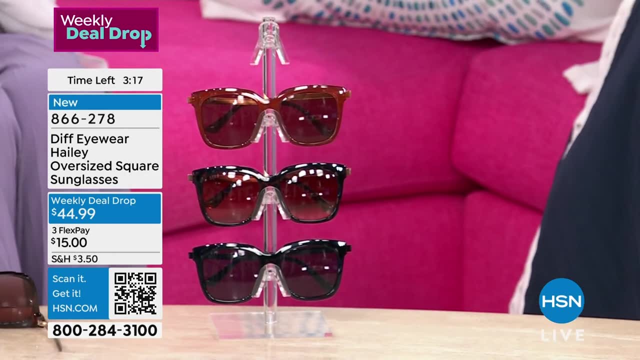 you can go to their website- about a hundred dollars a pop. Let me just pull this toward me And, if you guys don't mind, bring out the case as well. They do get a case included. Let's start with the lightest shade and I'll just put these on one by one and we can do a little closeup on me. 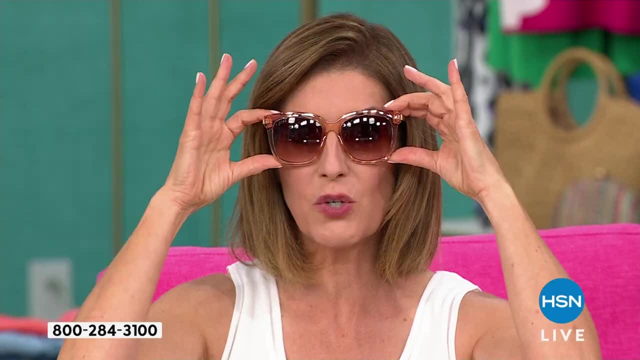 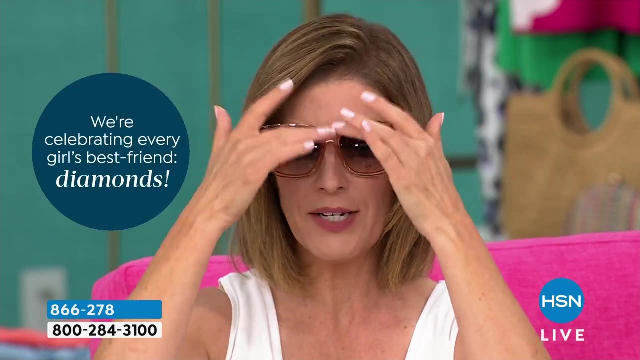 And you can see these are really flattering designs. It's a little bit of a square. I like the coverage because with the UVA and UVB protection I don't need any more wrinkles around my eyes Or my forehead, So this is the lightest shade. We're calling this one Crystal Nude. Look how. 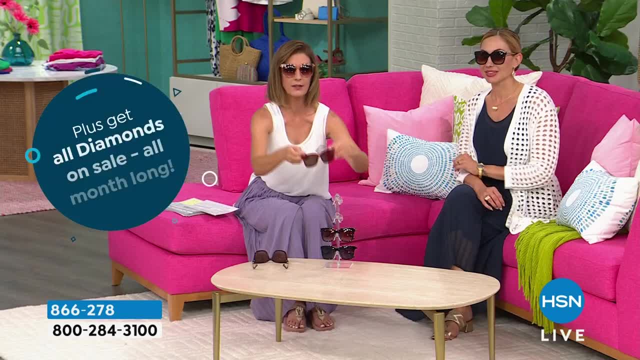 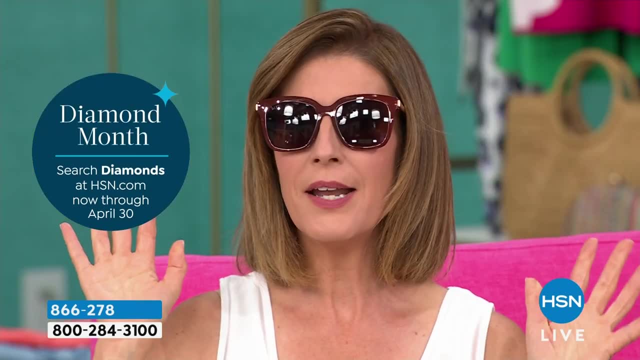 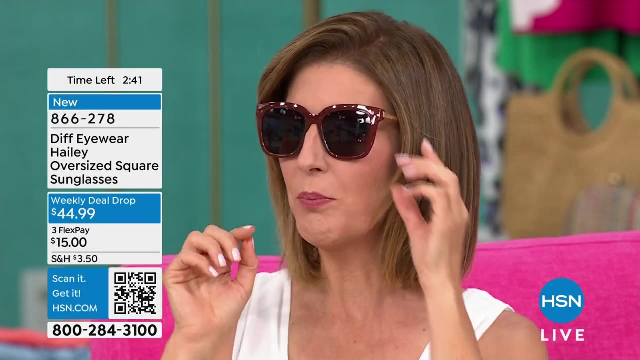 pretty that is. That's Crystal Nude. Okay, hang on. This is our next shade And if you guys don't mind helping me out with the colors while I'm, That's the Nut Nut Brown. Okay, Not hearing anyone, So I think that's a Nut Brown. Yep, Look how pretty that is. It almost has a red tint to. 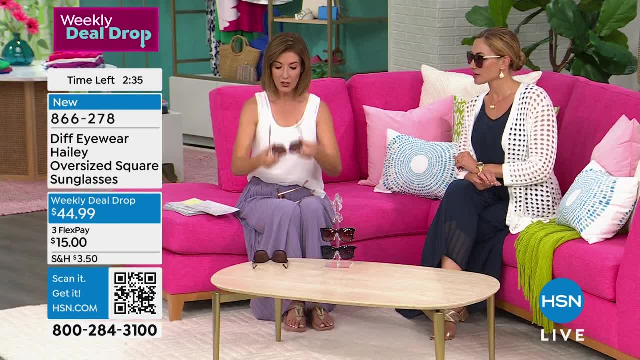 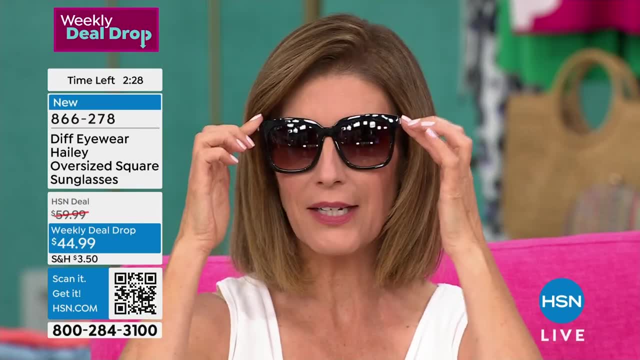 it. It's like a dark, A little bit of a darker lens. It's a little bit of a brownish-ish color. I think that's a good way to go with it. Yeah, It really is a good color And I just love that. look on that one. The color of the. 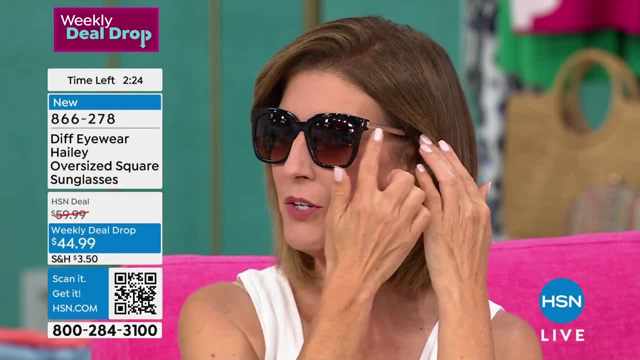 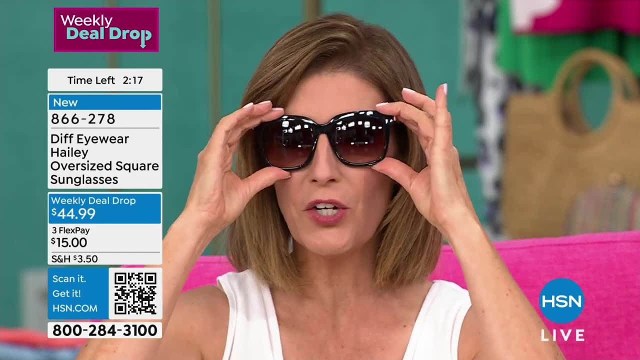 paint is really pretty as well, It really is, And it's just so beautiful. And then we get to our Tordochelle. Now this also has just again that kind of classic Tordochelle look, So Browns and Blacks, And then you get that beautiful. I mean, these are solid, stainless. 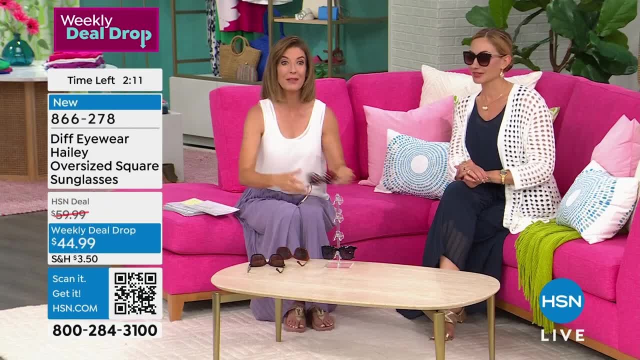 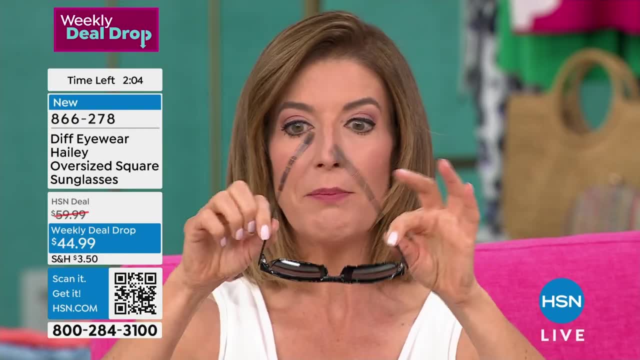 steel hardware accessories. These are beautifully made, very secure. They're not thin, They're not flimsy, They're not plastic. You get UVA, UVB protection And then there's black. So maybe are very beautifully made. You can feel that these are not flimsy. They are not sort of too easy to. 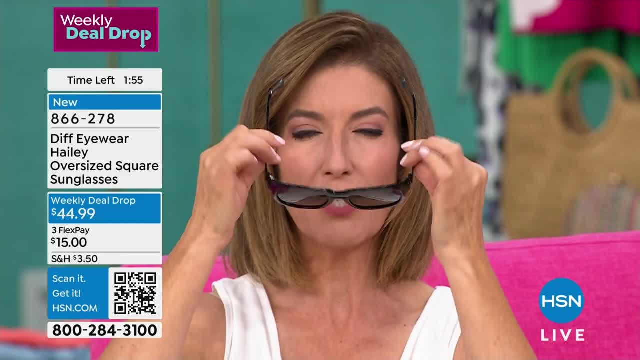 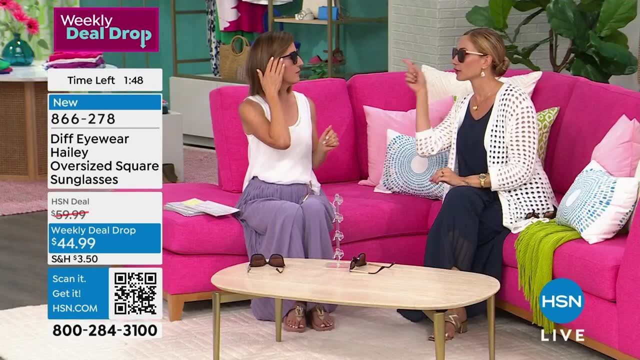 move. They have some tension there, And the fact that there's just a little bit of a spring means they're going to go on and stay on. There's the black Wow Okay, And the black earpieces are the only ones that are different. They're just a black color. The other ones are gold, but they're both. 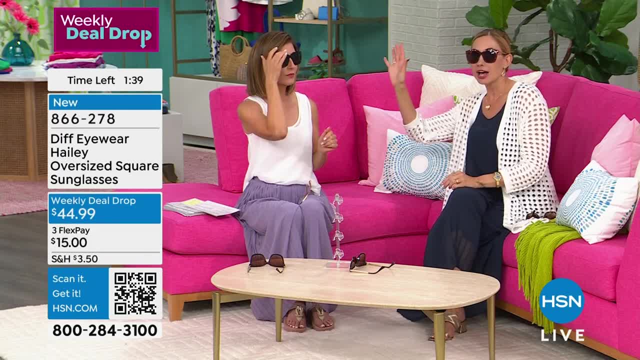 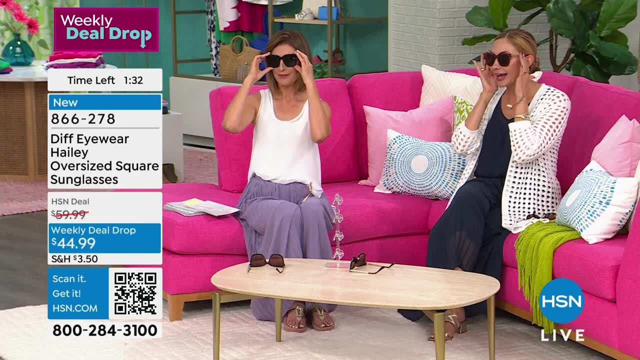 stainless steel. So you get a little bit of play there. If you want to do, I always say like all black, everything. If you're doing a whole like with your fashion, you've got the black on black. And then, if you like the gold accents- I love the gold earpiece accents, but all of them are- 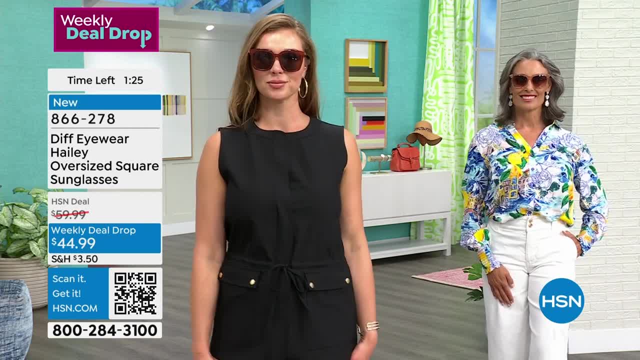 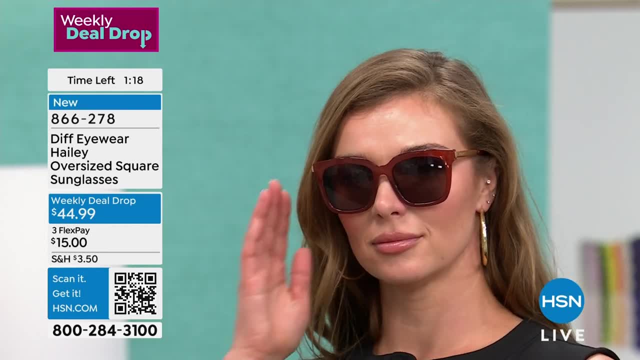 neutral, So they're really designed to go with just about anything. I love how they fit. They really sit up on your nose. They're not sliding down Right, And on these you don't have the articulated nose pieces, So it's all one solid piece. If you're that person that likes to put 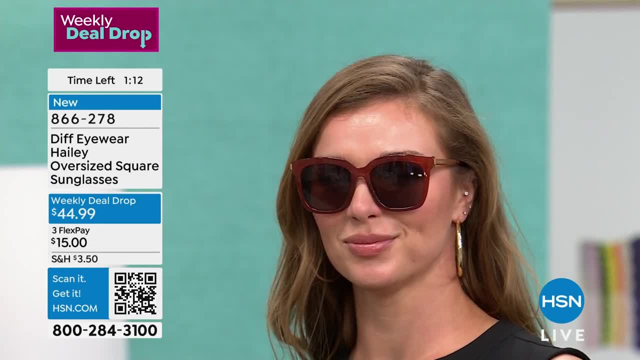 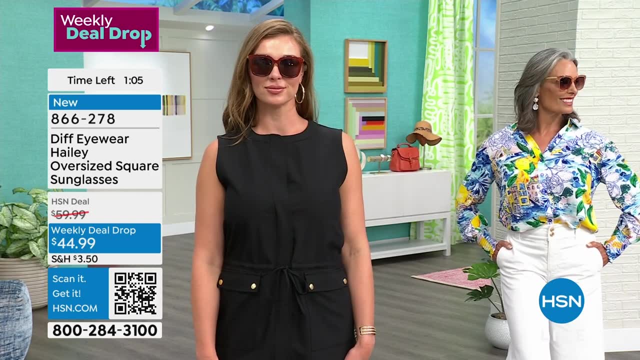 them up on your head. it's not going to get wrapped up in the articulated nose piece. We will have some other styles coming along. We have some aviators coming along and they they we'll have the traditional articulated nose piece, but know that with these it's all that. 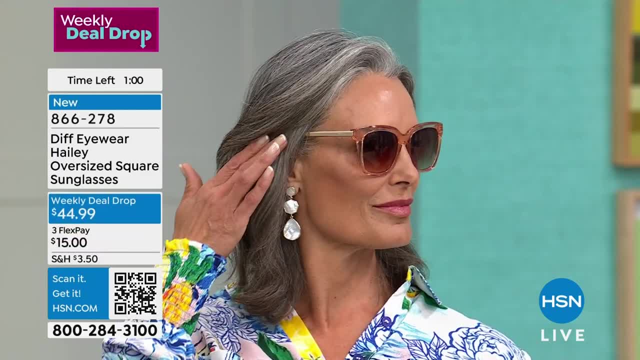 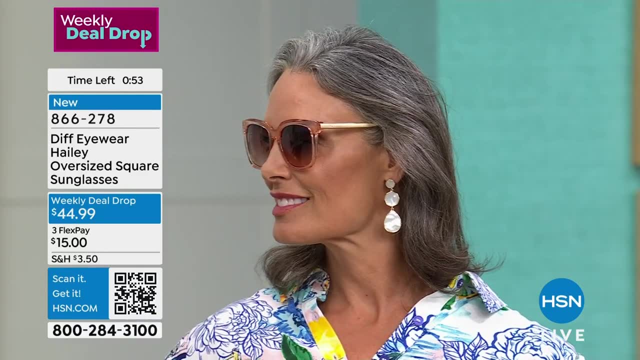 solid piece, but these look great. I'm thinking of these for gifts. You've got graduates, You've got mom, mother's day coming up. Even you know I'm always thinking ahead. I always I have a gift in closet, as I know a lot of you do. So I'm always like: Ooh gifts, One size fits all And 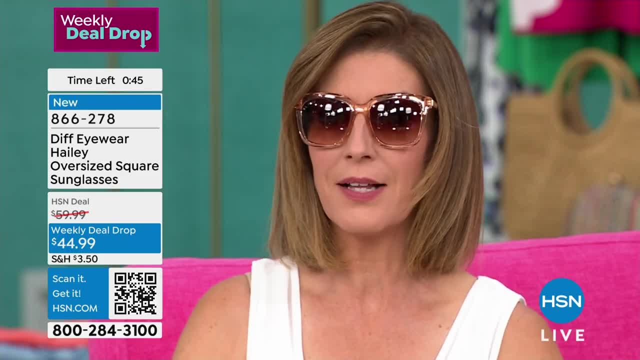 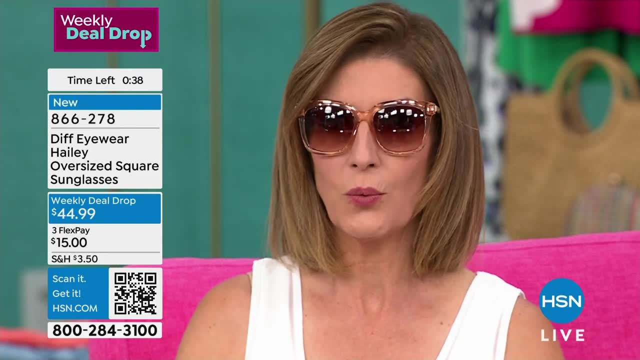 I'm telling you, a lot of us have spent a lot of money on sunglasses, Yes- And are you getting anything different than what you're getting here today? The reason and the answer is no. We can spend a whole lot more, maybe for a different brand, but what you're getting here, 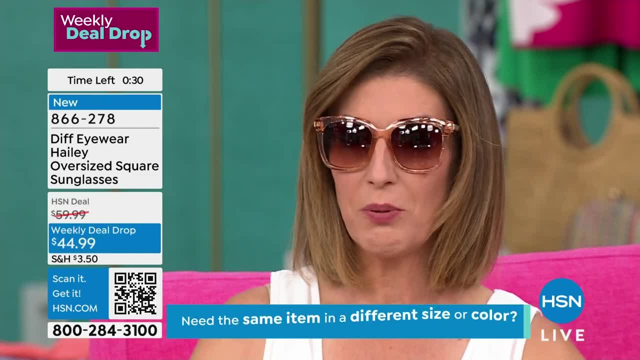 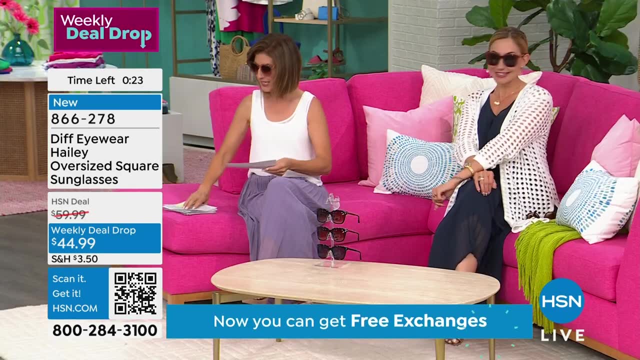 today. is that high quality, that affordable luxury for a fraction of the price? I would love for you to get these before they go quickly. It's our weekly deal drop. Thank you, Amy West, Thank you, Sarah. I feel very much in vogue and in style, but we've got a lot to talk about. 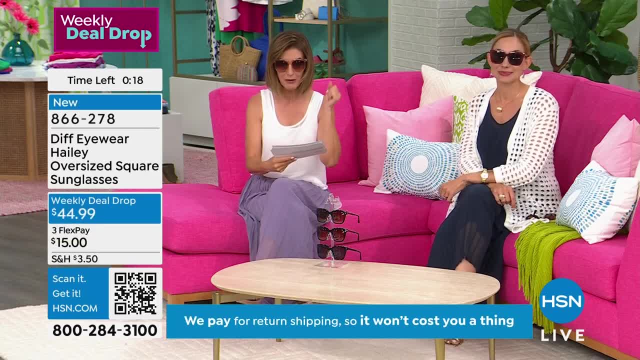 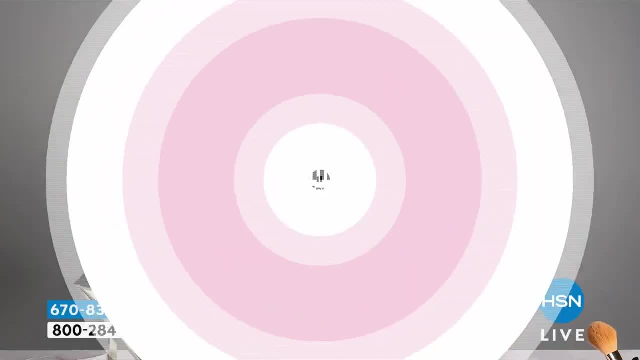 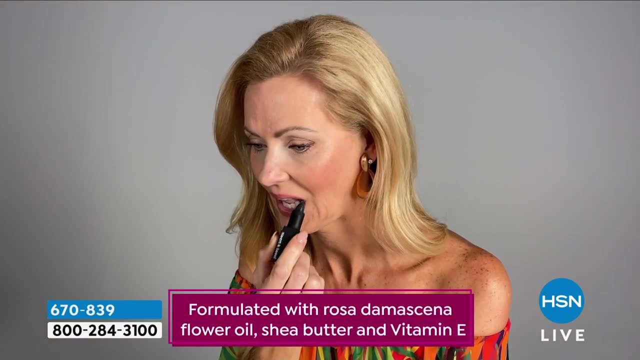 including our incredible weekly deal drop from Beauty Spy. We're getting ready to drop the two pack of the black heart and soul rose lipstick. It only happens once a year And once it's gone, it's gone. We have sold over 2 million lipsticks from the Beauty Spy. the Beauty Spy, Well, it's Chelsea Scott. She. 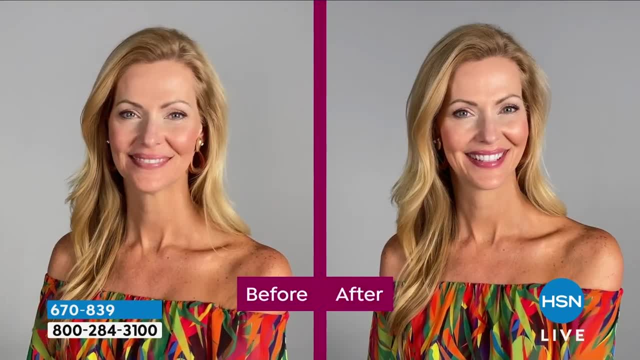 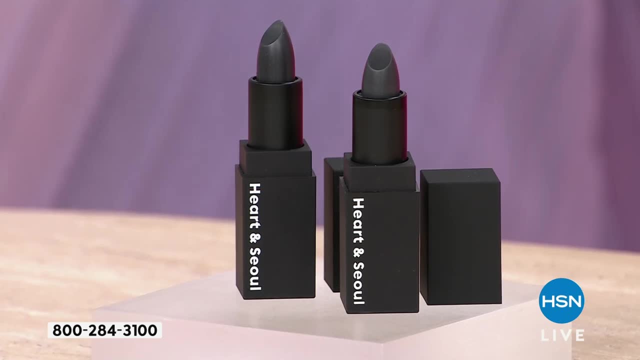 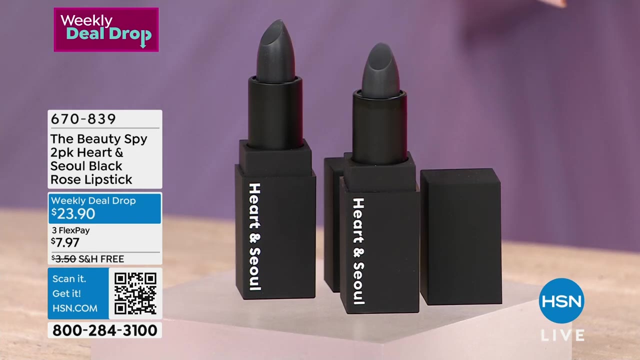 travels the world. She brings us the best of the best, And some of her travels take her to Korea. This is hashtag K beauty. This is what they're famous for. This is an exclusive offer here at HSN. Here's what we're offering. One is $24.. You're getting two for less than the price of one. 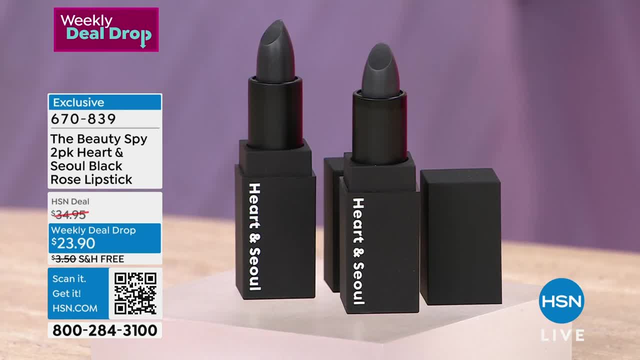 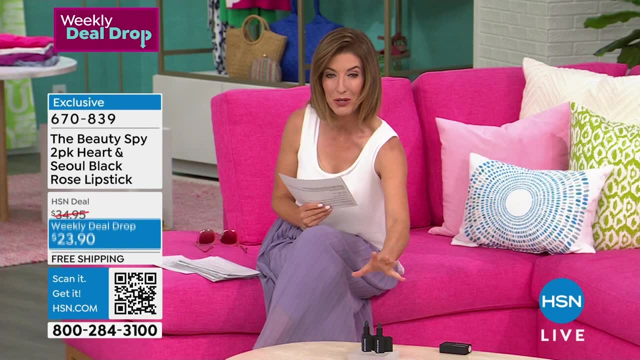 You're getting two for less And the price of one. She only brings this in once a year. This is your once a year offer. We have free shipping. It's not just a beautiful black, It's actually a deep purple rose oil. 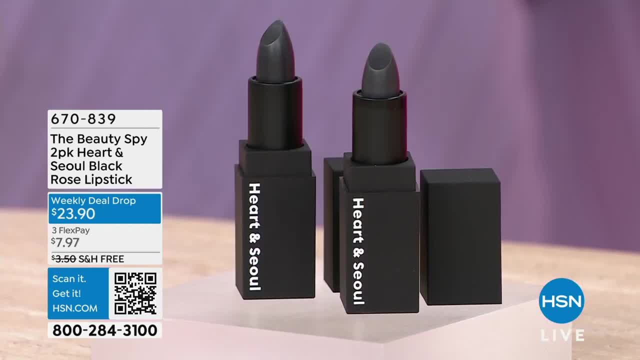 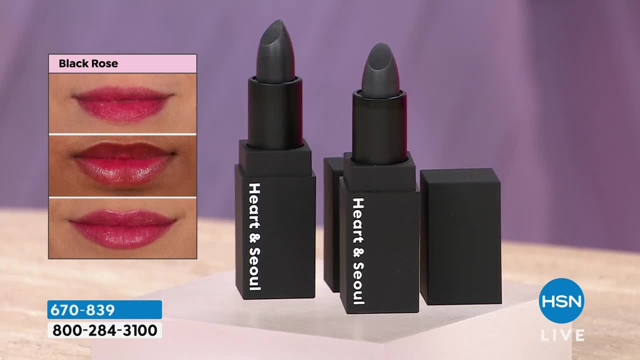 that actually interacts with the pH balance of your skin. So everyone's going to get a different color. Everyone's going to get ultra moisture, ultra hydrating, a smoother looking lip, a plumper looking lip. There she is, Chelsea beauty spy. She's got her purple shirt for the 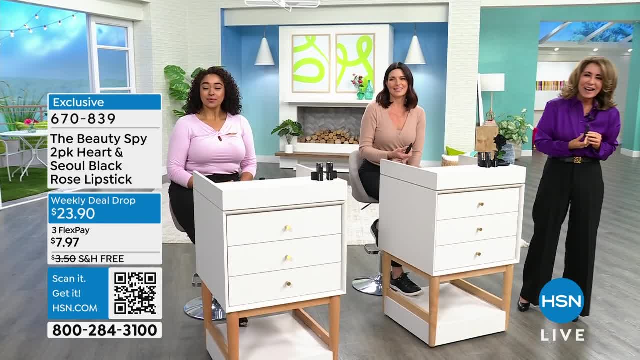 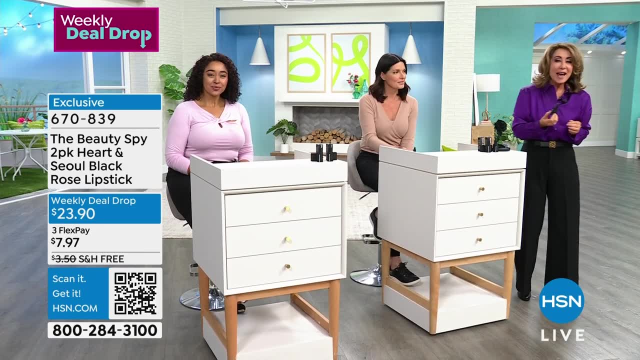 purple rose oil And talk to us about this, Thank you. Thank you so much for coming. We're this lipstick. this is. this- has been one of the biggest, most iconic cult favorites in the history of hsn and beauty spy. oh yeah, it really is exciting, hi, sarah, i'm so excited to be back. 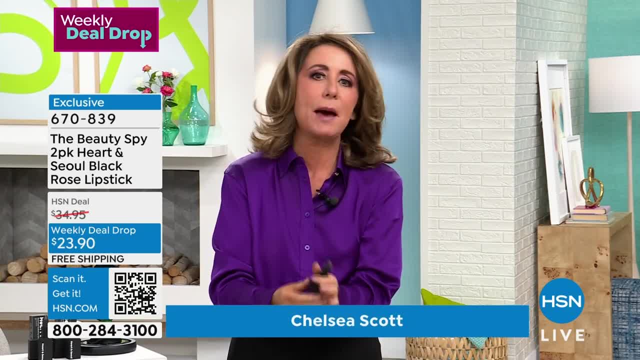 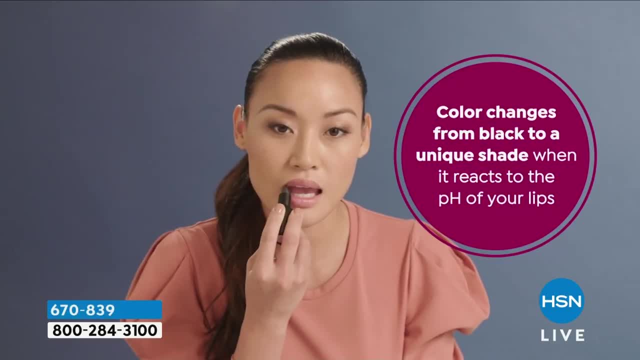 finally, with the heart and soul. it's the lipstick that everyone talks about and the reason why there's so many things. first, we can start with the color. obviously it's jet black in color, but it doesn't apply to your lips- jet black. the black is actually coming from the incredible deep, deep, 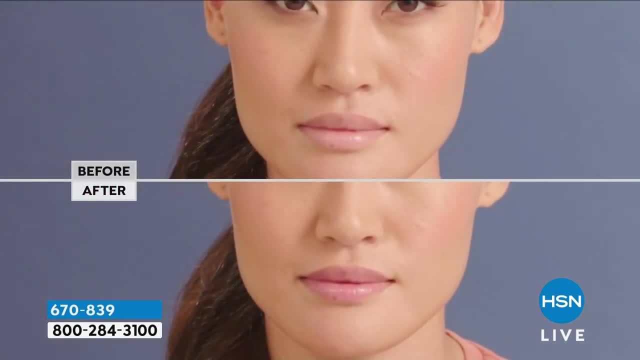 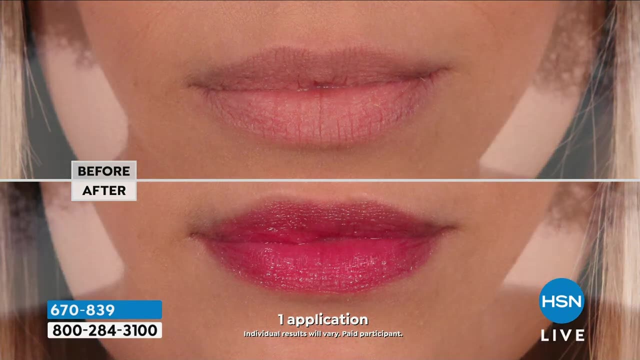 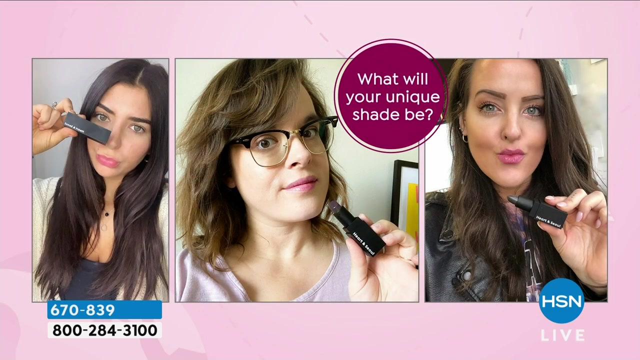 beautiful roses that are harvested in south korea. now, to be totally transparent, they are not jet black roses, they are a deep, deep, deep purple. we extract this gorgeous oil and it is so ultra hydrating for the lips. that's why everyone is so obsessed. if you have fine lines, crinkles in the 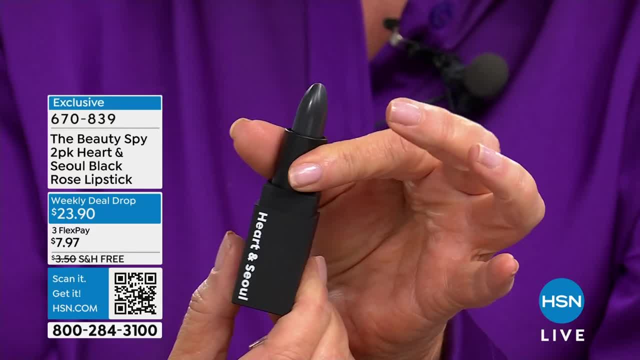 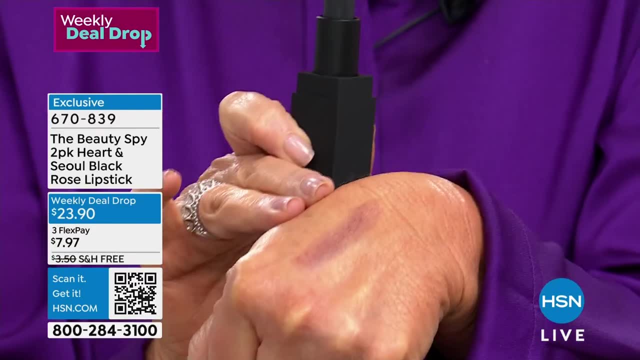 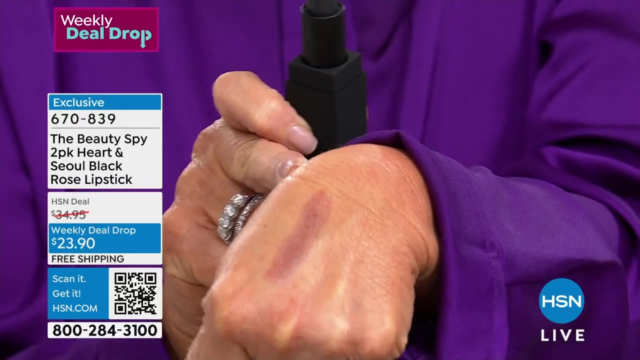 lips. if you have dry patches on your lips, this heart and soul goes to work to immediately hydrate, smooth. but here's the coolest thing, here's the technology. it actually works with your own skin tone and it starts to react to create your. you're watching it change, right there. live, that's. 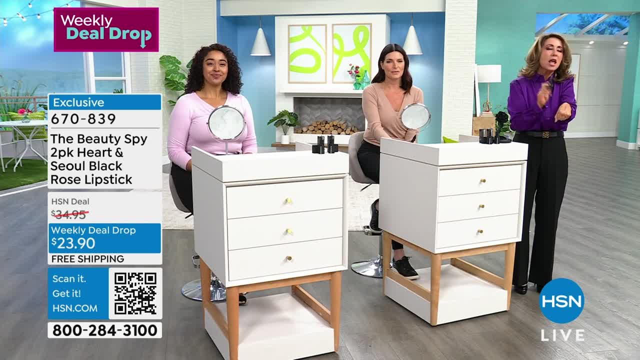 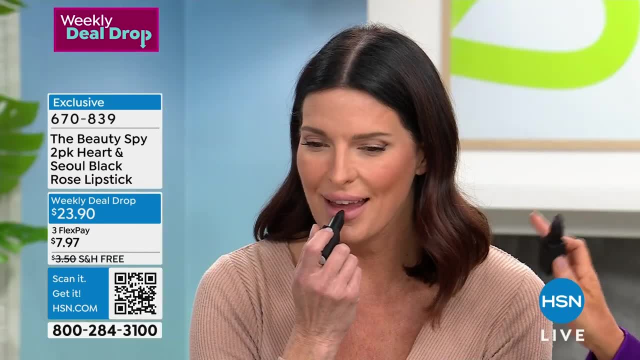 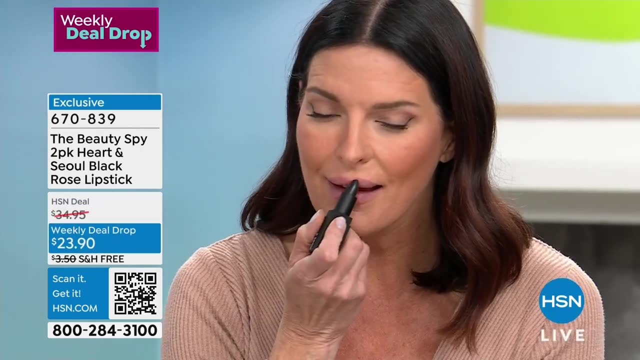 pretty amazing and it works with your own ph level, so it is the most hydrating. hydrating, is that a word? yeah, okay, it's the most hydrating lipstick you guys have ever tried. so we're going to show you how. on all of the girls it looks different on all of us, so you don't have to worry about. 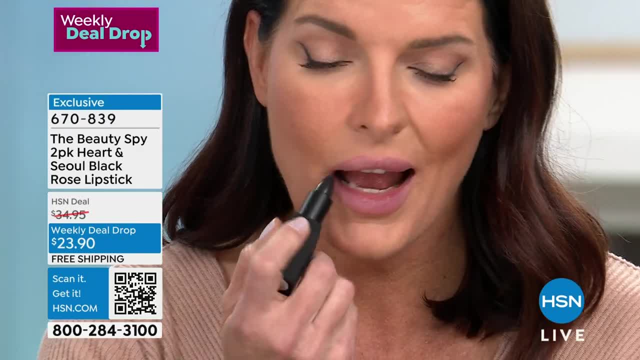 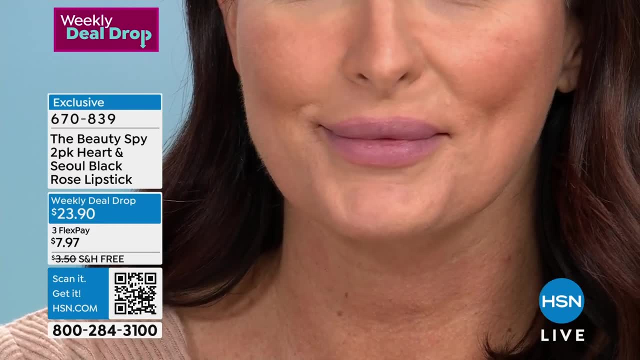 choosing the color. this lipstick is just giving you the perfect color that your lips were meant to be, and i don't know. i always talk about berries. i don't want to go down a road that i can't recover from, but in new york, when i was, 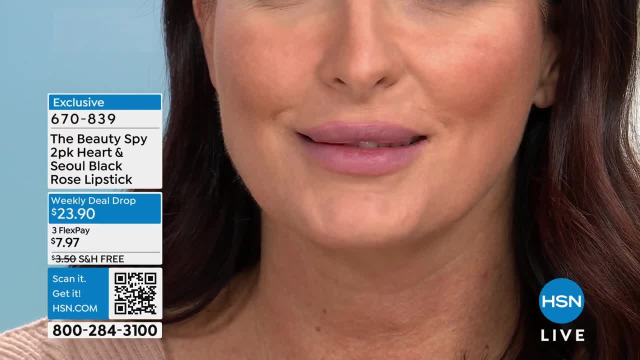 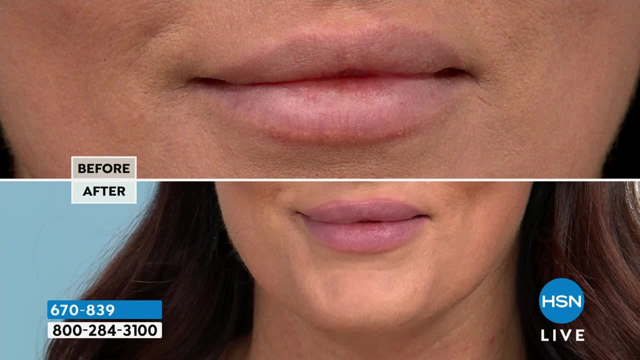 growing up we had these blackberries that would grow in the backyard and it was really funny because it would stain your lips. if you ever experienced that growing up, that's the kind of color that it's going to transform on your lips. it's that very kind of berry, youthful, juicy look. 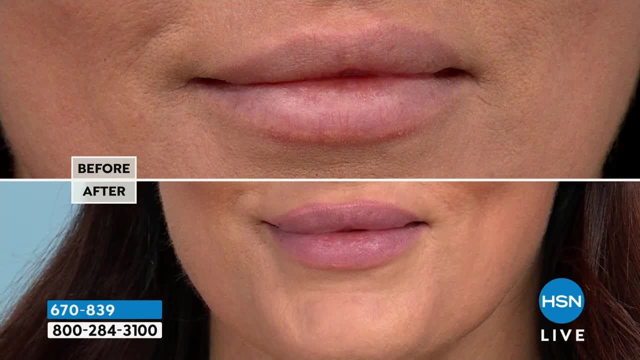 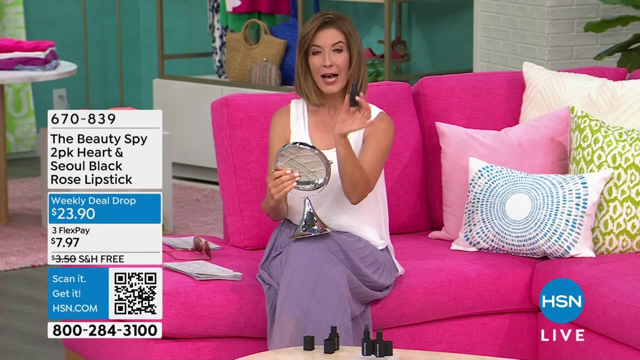 okay, we're already getting so busy. i know you wait all year for this. it only happens once a year. the sooner you place the order, the sooner we can get this out to you. is this not the best thing ever? how many of you are going to be able to get this out to you in the next couple of years? i'm going to. 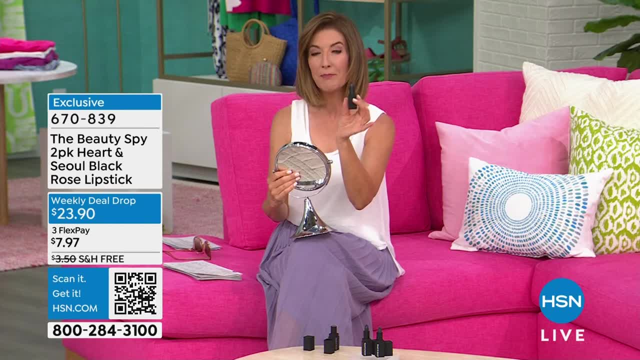 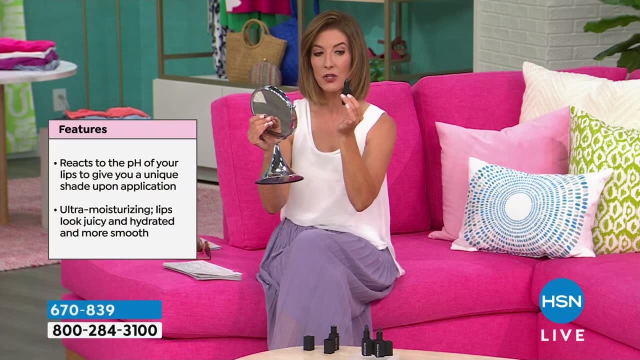 freeze when you buy lipstick because you're so afraid of buying the wrong color right and you don't want to get stuck with anything. this lipstick is going to be designed just for you. it's customized to your lips. it looks like it's black in the tube. this is so much fun. and then 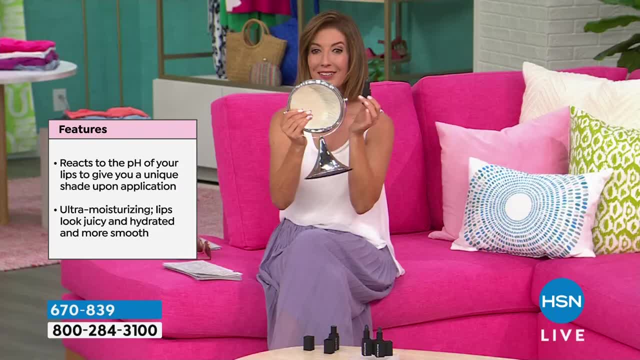 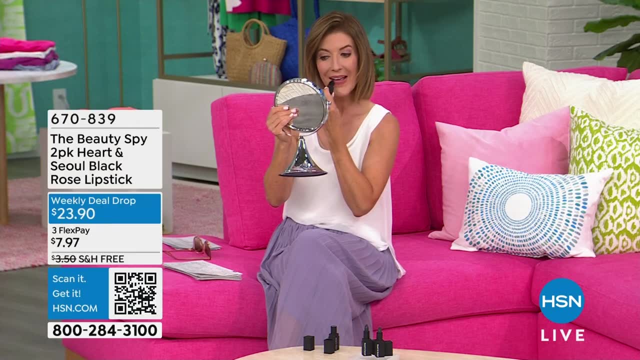 you're going to get it home and the first thing you're going to do is go. i wonder what it's going to look like on me. so i'm going to pull up my mirror and i'm going to go ahead and apply it. it's very concentrated, it's very rich, it's very luxurious, it's very juicy, hydrating. 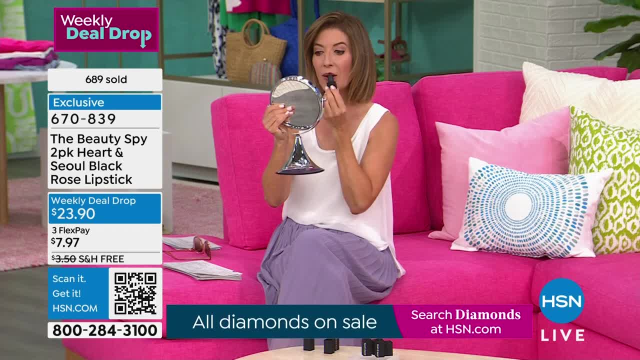 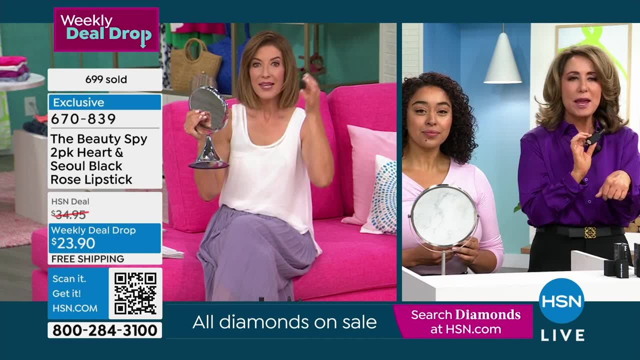 mm-hmm, it's like a lipstick, a lip gloss and a lip stain all in one. yeah, and already you'll start to see the change in your lips, right? you don't have to wait very long. you don't have to wait. it's the heat of your skin. yeah, and no one is going to have exactly the same color, right, exactly, and 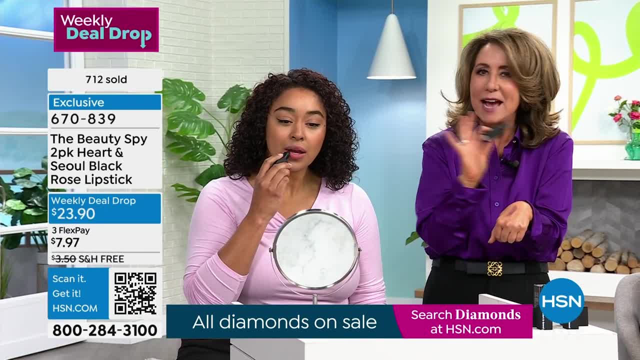 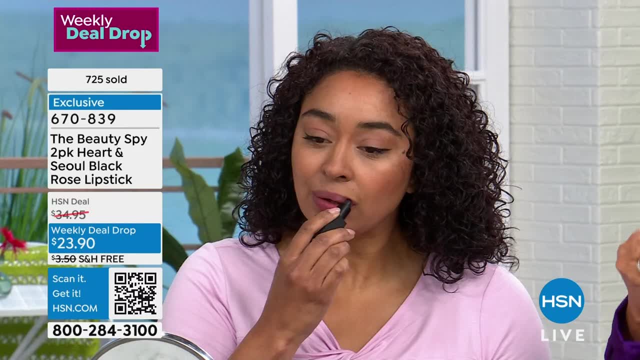 that's really cool technology. but even more important, yes, it's fun and that's great. you're getting to see your own color, just um, appear right before your eyes. you're looking at kenya now. hers is going to be different than sarah's, is going to be different than mine, but it really 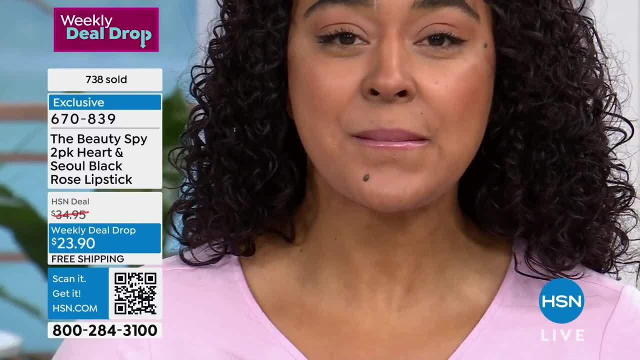 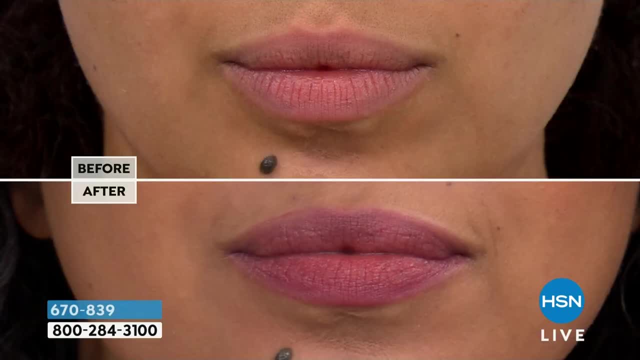 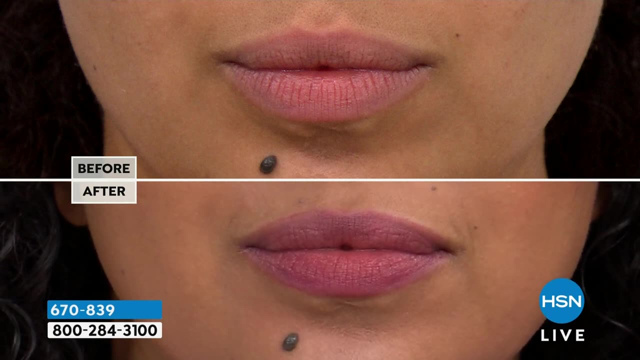 is the heart and soul- no pun intended- of this lipstick is the transformation to aging lips. so if you look at kenya in the before, if you've got like patchy lips or dry lips or your lipstick is constantly migrating or you feel like your lips aren't plump, and then you buy all of these. 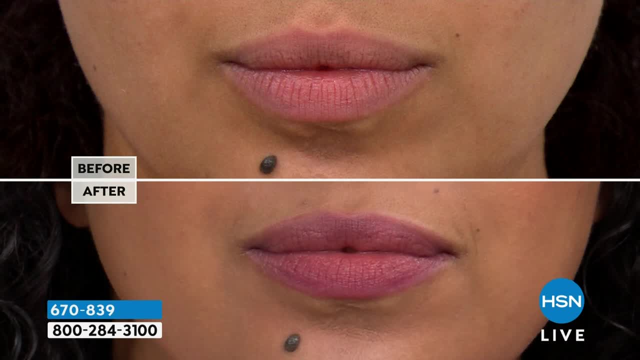 lip plumpers that are stinging and they really cause uncomfortable feelings on the lips. the heart and soul has been known around the world. literally it's that famous. at this point, we've been doing this. this is our third year for the hydration, for the plumpness that it gives your lips, but without ever being uncomfortable. so 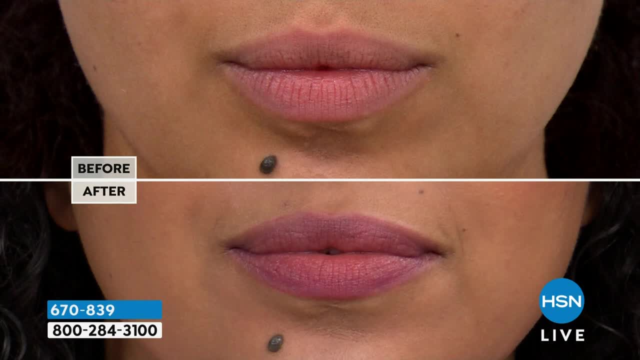 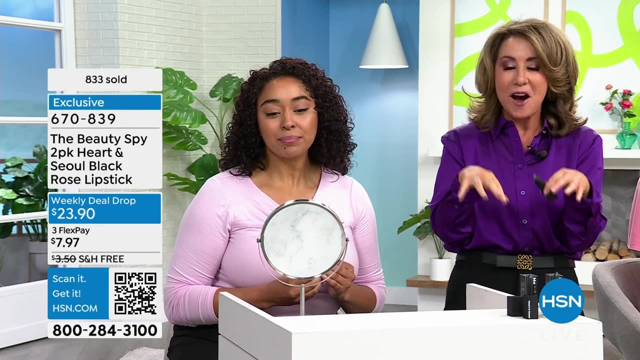 what happens was is we actually- you guys all know this by now. i talk about i spend half of my time in south korea. in fact, um, join us on may 1st, mark it down, we're going to be live here on hsn from south korea. it's a first. it's never happened before. i didn't know about that. yeah, yeah, we're. 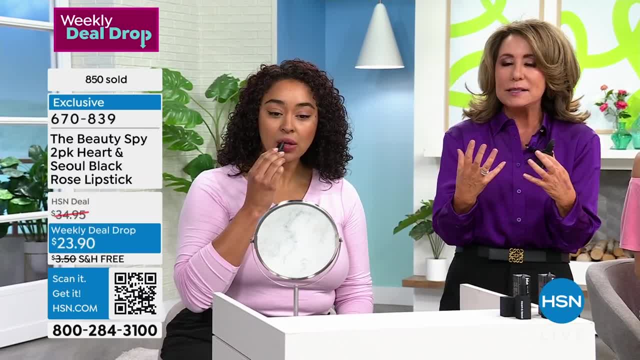 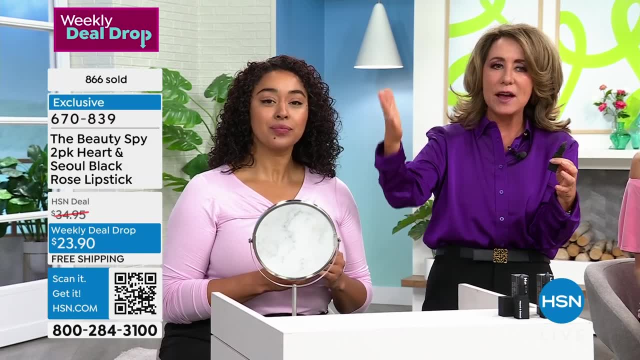 doing a whole day live from south korea. um, and what's so great about south korea is if you read about it- just type in korean beauty- it is literally the hottest thing in the world because their technology is 5 to 15 years ahead of everywhere else. we are on the ground in south. 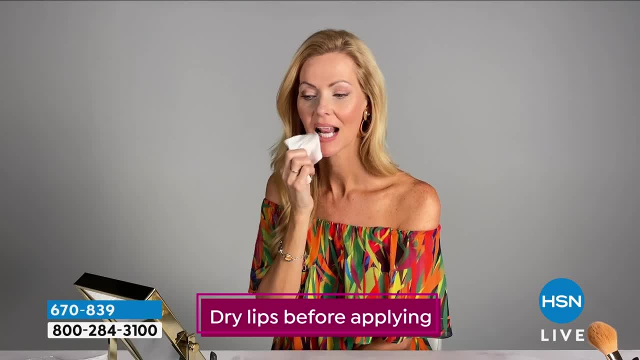 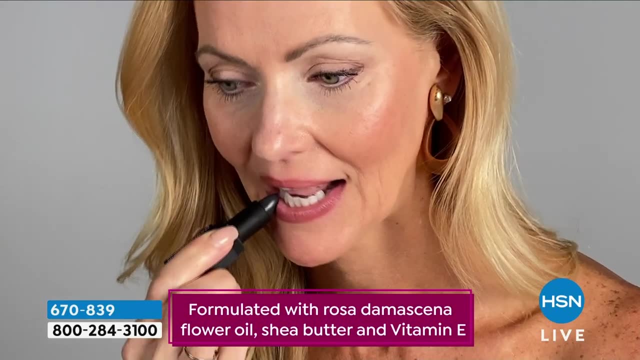 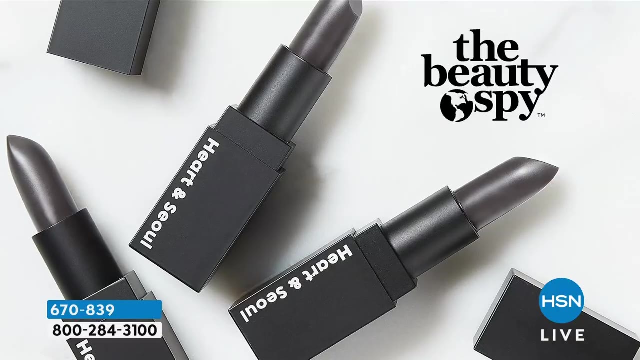 korea with our teams, and we actually have a team that harvests these roses for you. they bloom before 6 am, they are pulled out of the ground and they use every part of these deep, deep, deep, deep purple roses, from the stem cells to the actual petals. um, and it's an incredible technology, because this? 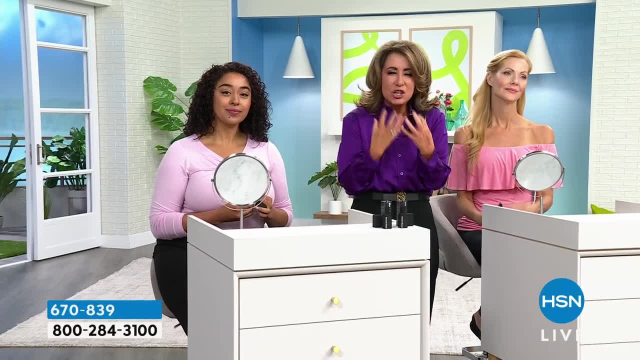 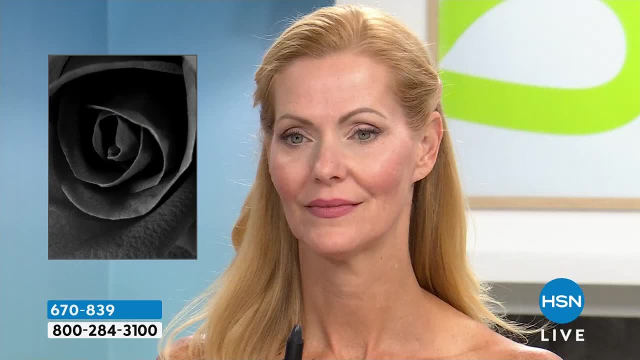 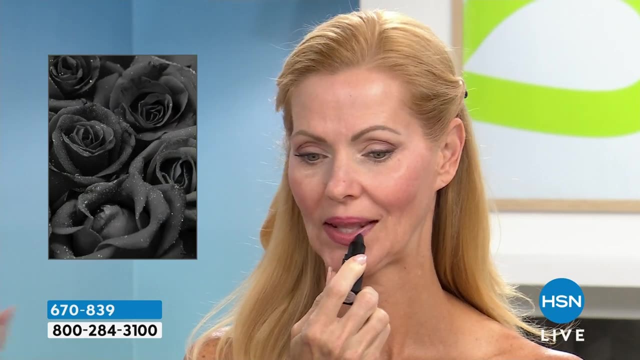 rose. damascena oil that's coming from this black oil is so juicy and rich and hydrating. you can actually see the rose there on the screen. so it's just a beautiful story. this lipstick is made with love for you guys and it is completely exclusive to hsn. you can't get it anywhere else. 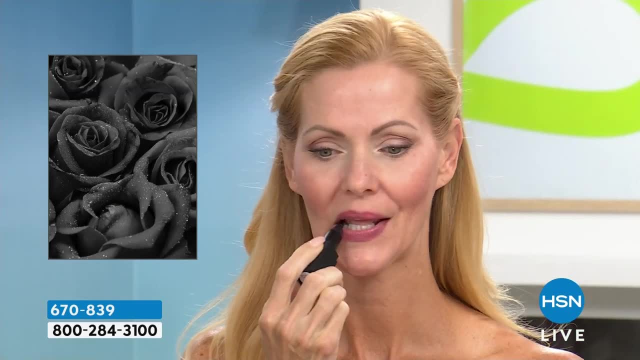 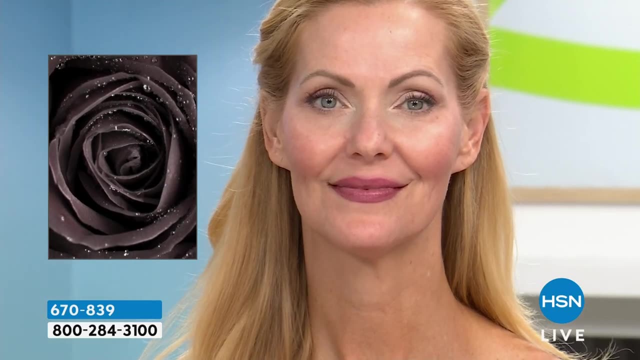 in the world and we only do it once a year. it's a huge customer pick. the rave reviews are in and it only happens once a year. it's a. it's like better than a: buy one, get one. one of these is 24. we will not be able to repeat this offer in the rest of 2024. if you do this now, lock it in. 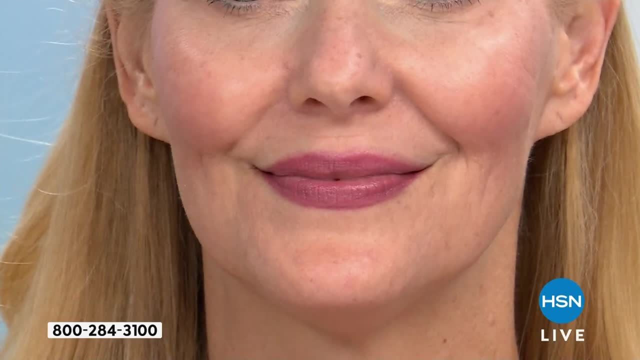 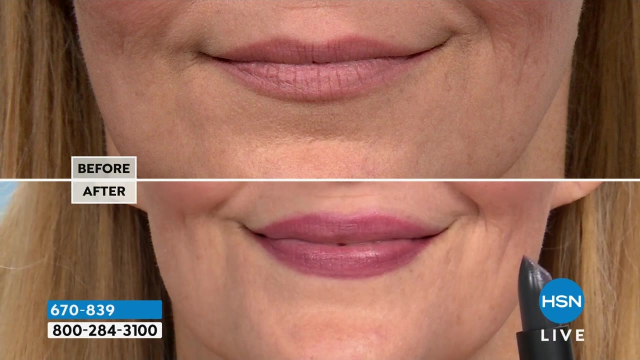 on your calendar to try our best to make it happen. and, as of today, we have given away 24 очкіński pink rose next month, so stay tuned. we are going to give away one of these mommy skin care product. you can put this on and you don't need to worry about any extra set. 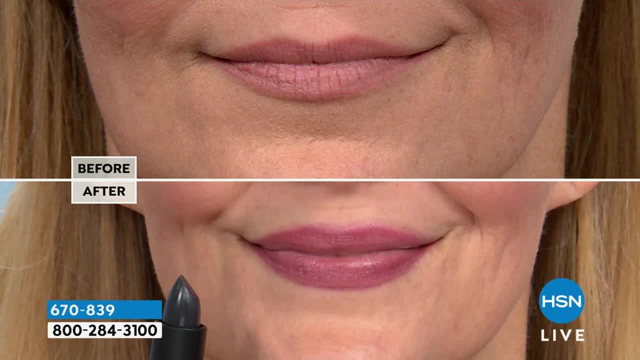 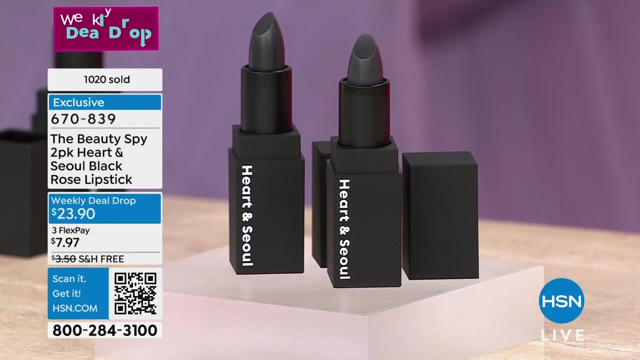 because these are the coolest things to share with girl, friends, a sister, a mother, a daughter, any family member. they'll be so thrilled the fact that you can give it to anyone. you don't have to worry about their skin tone, you don't worry about their skin type, just say, put this on, i can't wait. to see what the color is going to look like on you with the incredible black rose oil, shea butter, vitamin e, all these amazing extracts, oils, key ingredients. they're super nourishing. one is 24. you get 2 for less than the price of one. i'm going to see where it goes in the next few minutes. 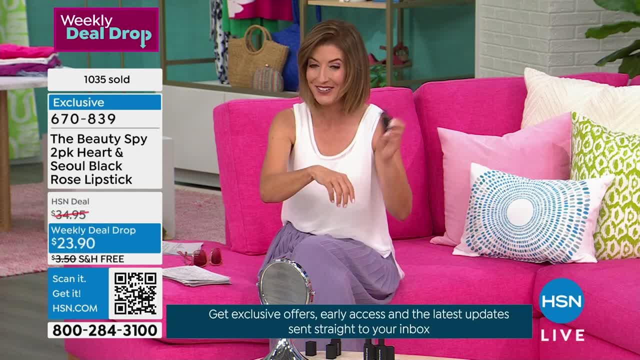 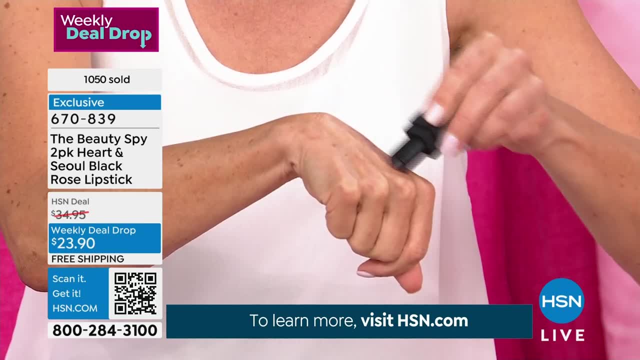 gonna put this on my hand because you're gonna- you're gonna- be so excited to get this home. i know you are. yeah, we're already very busy. uh, go ahead and just put it on your hand if you want to, sort of you know, tell a friend about it, and then within moments, my lipstick already does not look. 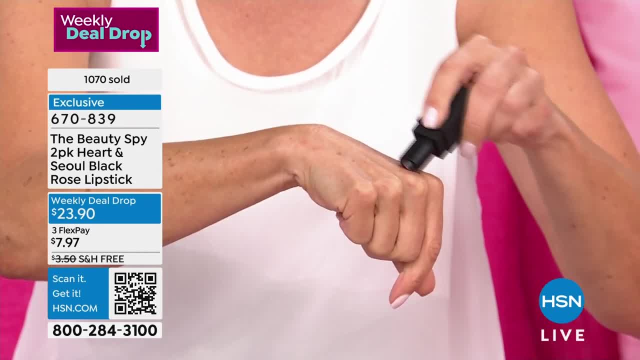 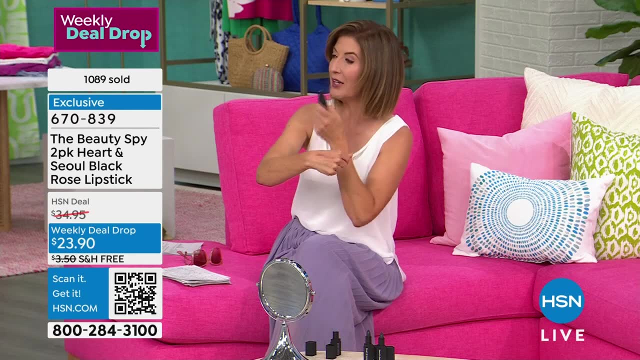 black. it doesn't come out black, right, right. no, that's the magic. it's already turning like a beautiful kind of berry color, yeah, and the more i apply, the darker it gets. and then does the color stay? yeah, so it's really cool technology. it's a hybrid between a stain, a gloss and a long wearing. 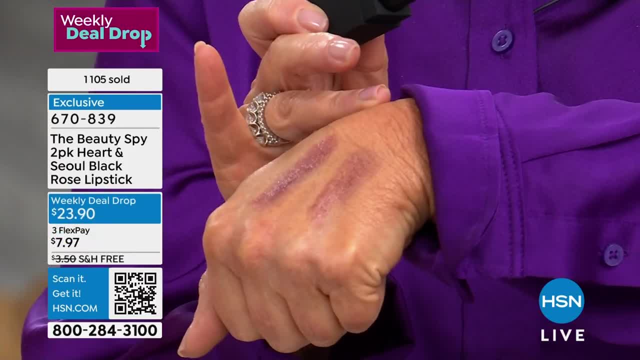 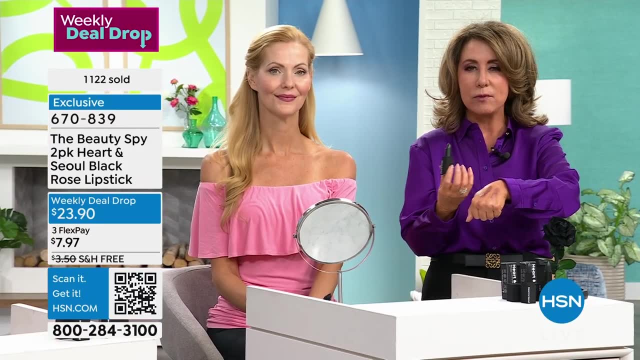 lipstick. that's what makes it so unique and why you guys keep coming back, and i do want to say that there is only one other company i that i'm familiar with globally that actually has access to the rare black oil. um, and that one i don't even know. it's ridiculous. it's like fifty dollars for. 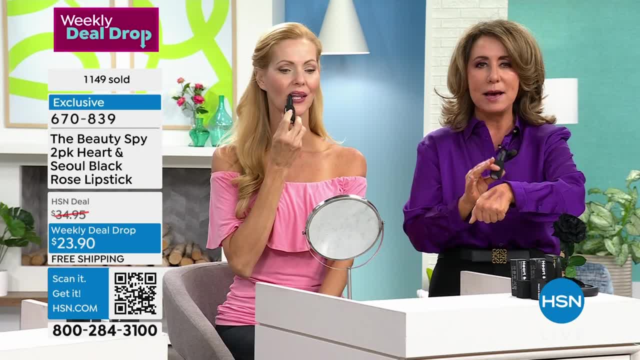 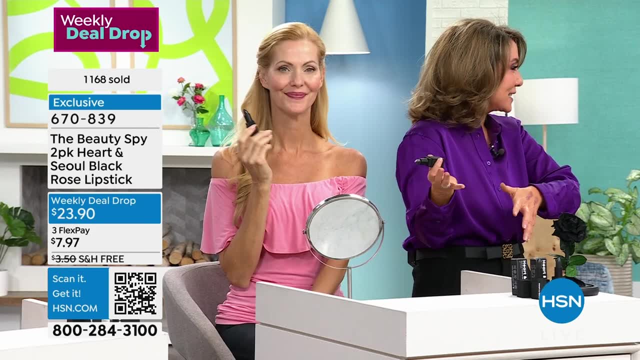 one lipstick. so we really went out of our way to bring you the best of the best today, and i- i mean the value, obviously- is crazy, sarah, because this is the same price as when we launched it, or even less, i think. i know, um, but if you are just joining us, i know we. 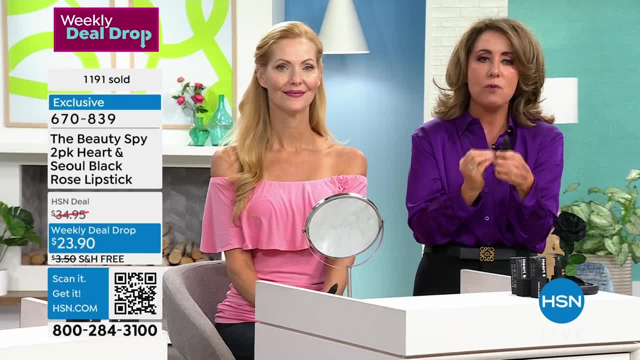 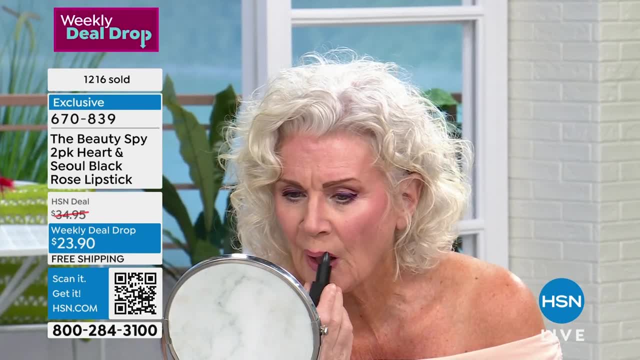 don't have a lot of time so i want to show you on everyone. this is that very rare heart and soul black lipstick. it is completely exclusive to us at the beauty spy. what makes it different, it's the ingredients. so when you apply this to the lips, it is packed with essential oils. that beautiful black. 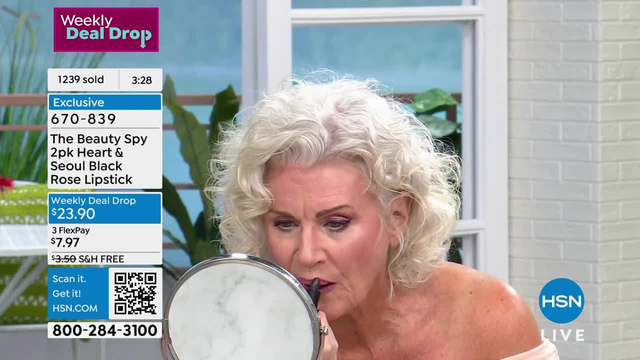 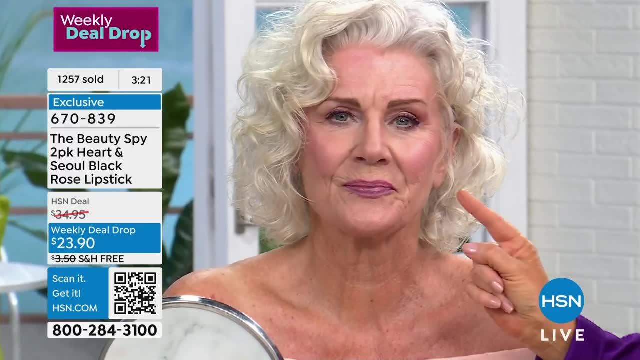 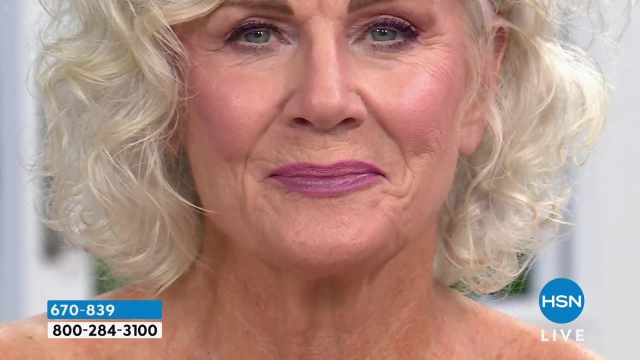 rose oil, which gets into the lips and drenches your lips, and hydration. it is literally going to transform your lips. if you have any dryness, if you have lipstick that normally drags on your lips right and pills up, if you have lipstick that's uncomfortable, if you guys use those lip plumpers- oh my gosh that have all those ingredients. look. 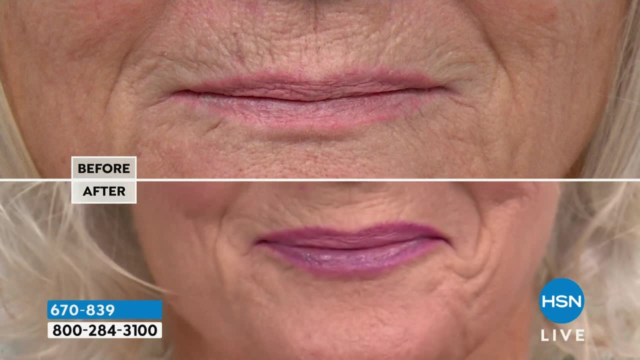 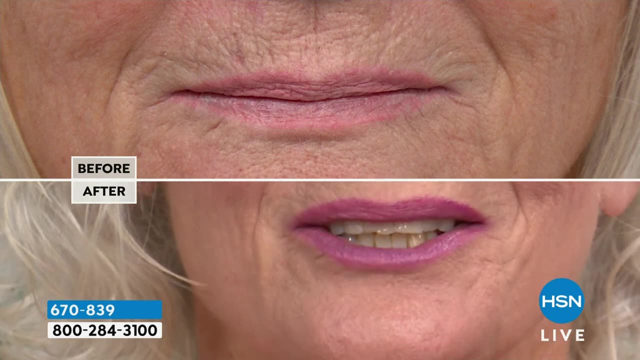 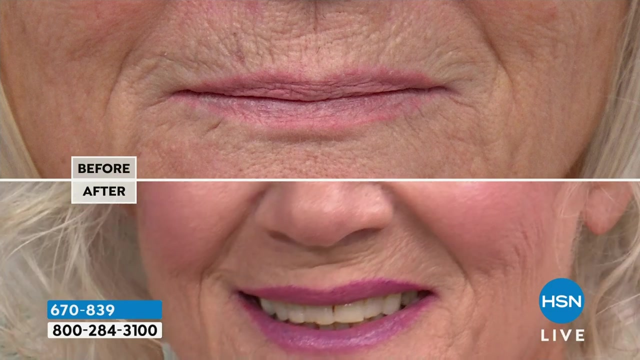 at the difference here in this before. come on, look at the before. that's me right. i always have the lines in the lips. look at how gorgeous um her lips look. they just look juicy and hydrated and it's the perfect color that just gives you that pop. no more guesswork. no, it's going to. 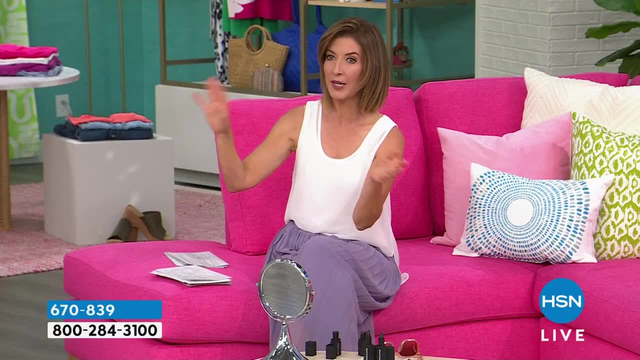 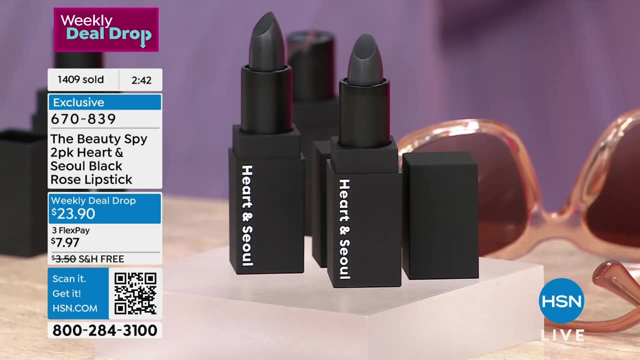 be a lot of fun. perfect for you. here's what's happening. we have 400 people ordering. uh, it's a weekly deal. drop is supposed to last an entire week. i can tell you right now it probably won't even make it through wednesday. so you need to order yours right now and that way we can get this out to you. you can. 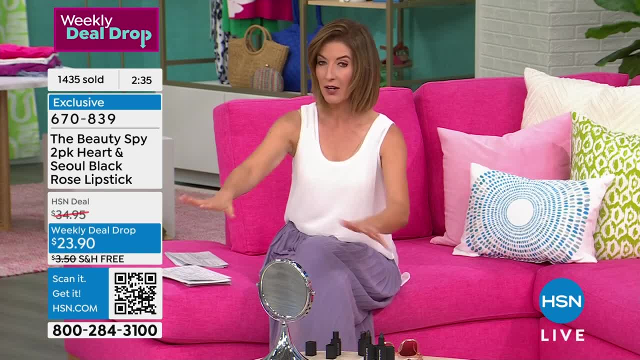 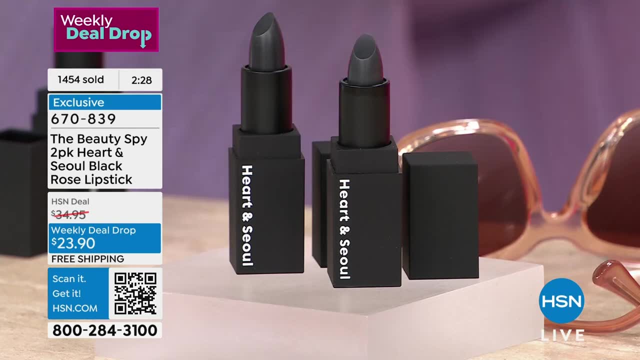 order by scanning that little qr code. these have a cult following, these are iconic, these are famous. we've sold two million of these, and only once a year do we do a buy one get one free. that's basically what you're getting here: a buy one, get one free. you don't have to worry about the color. 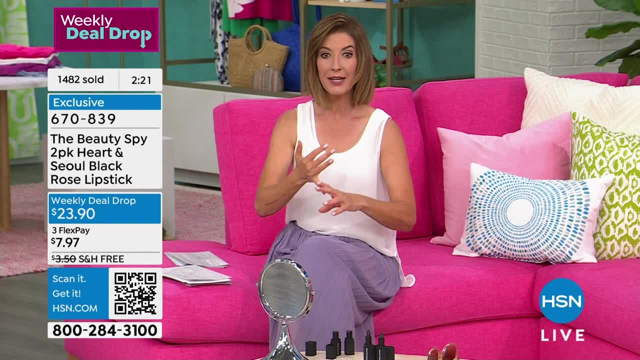 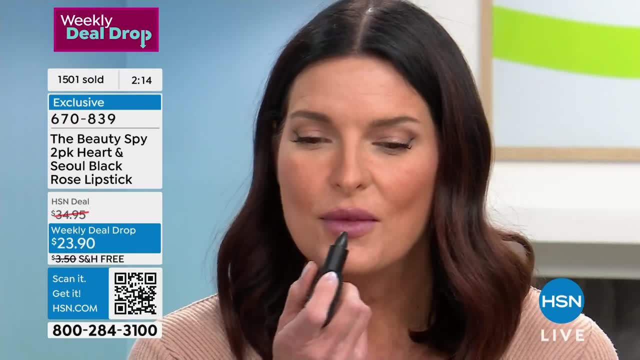 or the shade, or the tone or the type of lipstick. you're going to get one free and you're going to have lipstick. just make sure that you're getting it and get more than one while they're in stock. you can also order online. you can give us a call. uh, go to automated ordering because we are so busy. 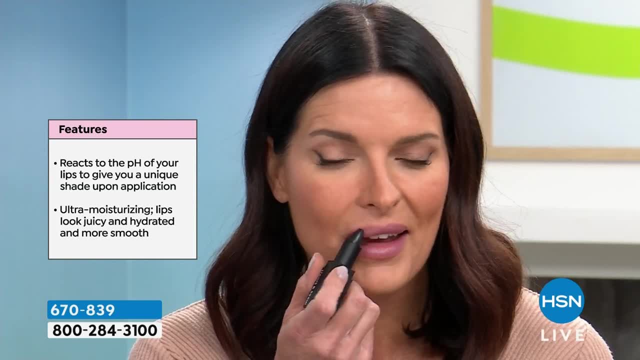 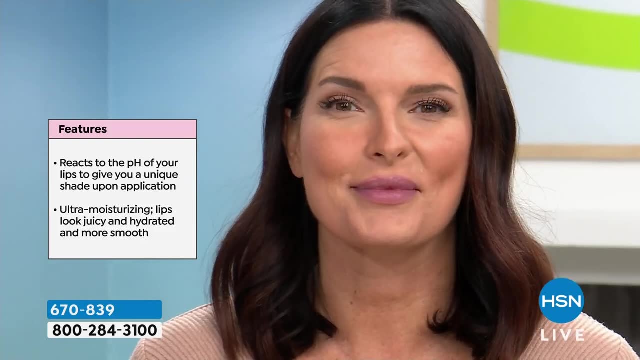 we're three minutes away from ronda shears today's special, so the sooner you order, the sooner we can process your order and make sure that you're going to be a part of the family, and i think that's what makes this so special- that there's really no other lipsticks in the world that do. 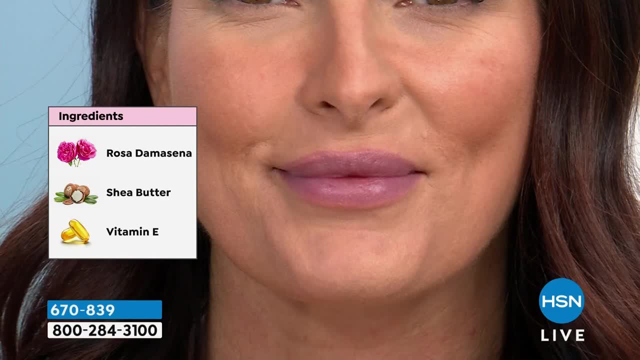 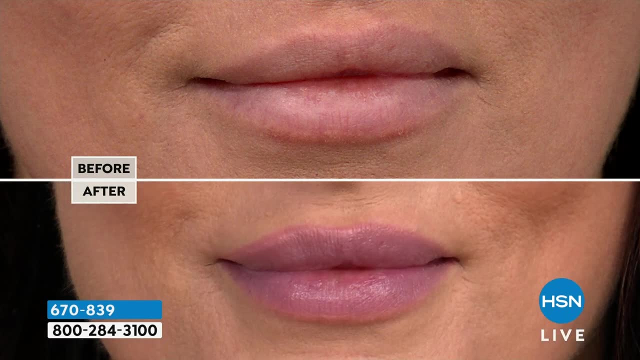 this, uh, and if you did find one, it'd be more than fifty dollars a pop for one lipstick, right, and what's so unique about this is it's different. take a look at angie again, if you look at that before, if you are just tired of the lip balms and all of the heavy lipsticks and all the 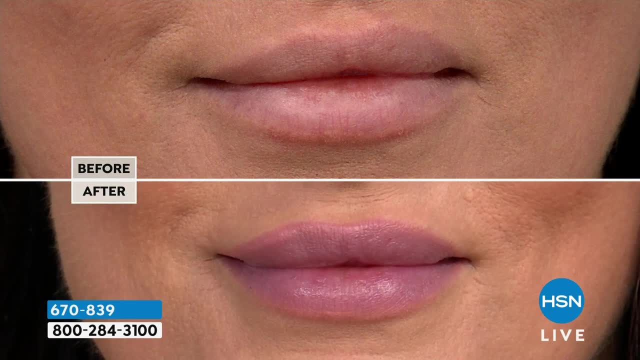 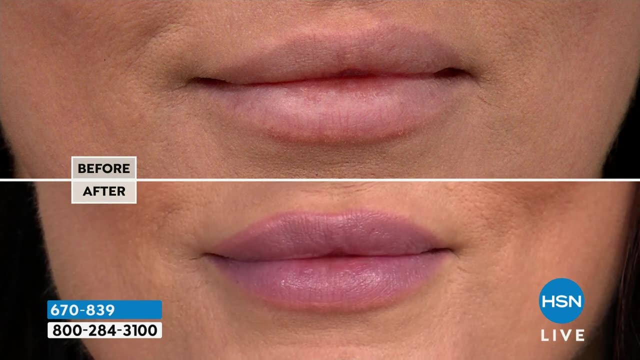 glosses that you apply and then they're: they're off of your face a bit off your lips a few minutes later because they're slick. this is a very, very unique technology. it's a hybrid between a gloss, a stain and this emollient lipstick that's really long lasting. it's unlike anything you guys have. 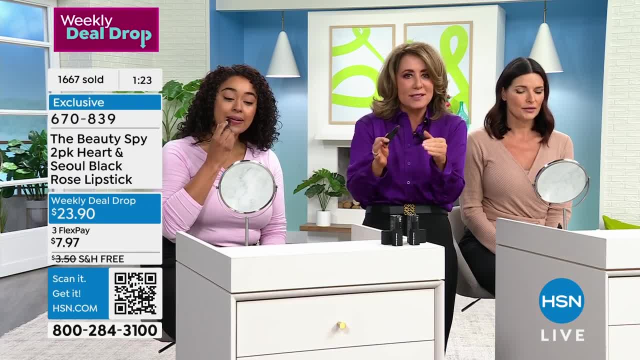 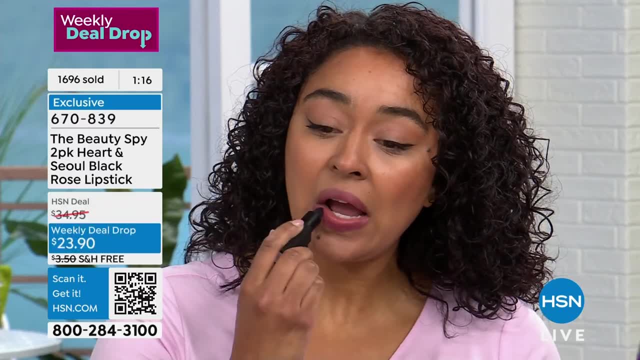 ever tried. when we say that it's only here once a year. you can't buy one, get one free. and you guys can google it like: look at the last time we were here, it was this time last year. because these incredible roses, we're going to show them to you. live from south korea. on may 1st, it is fields. 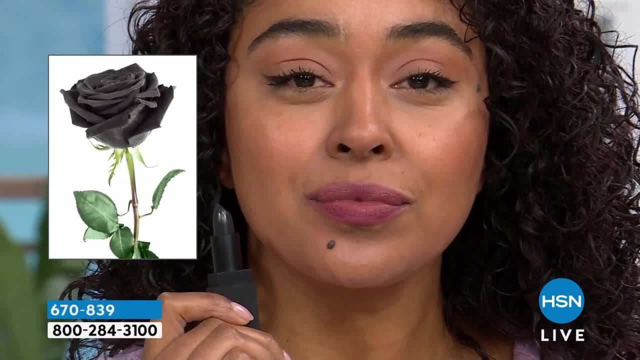 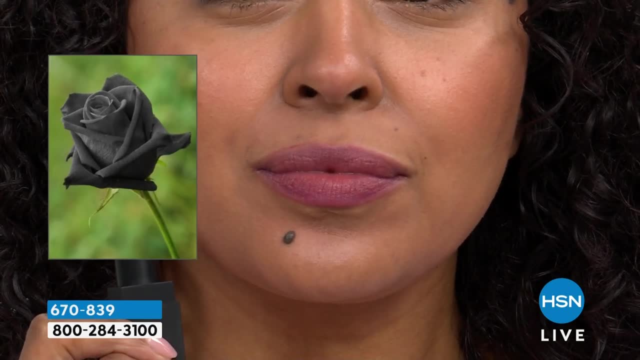 and fields of these incredible black roses. they are actually a really, really deep purple. there's no such thing as a black rose. it's a deep, deep, deep purple that looks almost black and in person, in real life, they are so exotic and beautiful and it's overwhelming. and the fragrance and the scent. 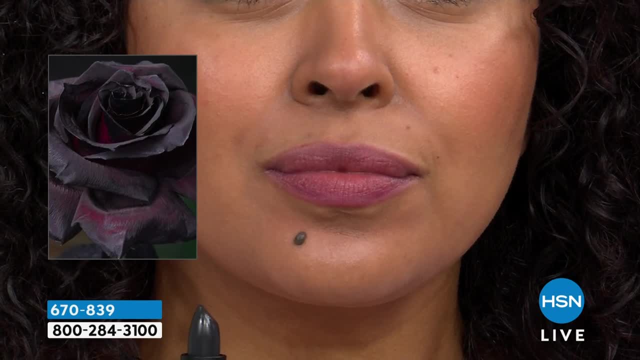 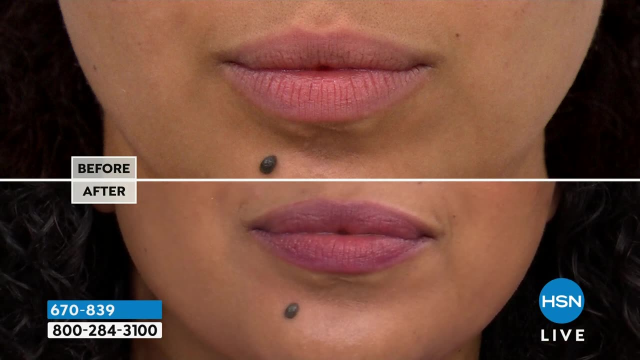 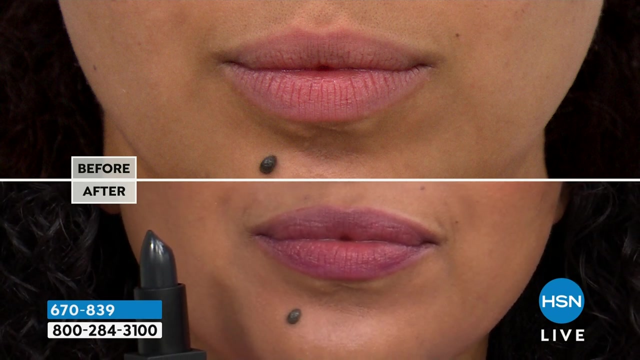 and we extract that oil and we pour it into the heart and soul of this lipstick and create a lipstick that is so unique that it looks natural. it looks like the color your lips were when you were a child, right, when they had that natural kind of juiciness that doing this- uh, by the way, question coming in real quick, what's? 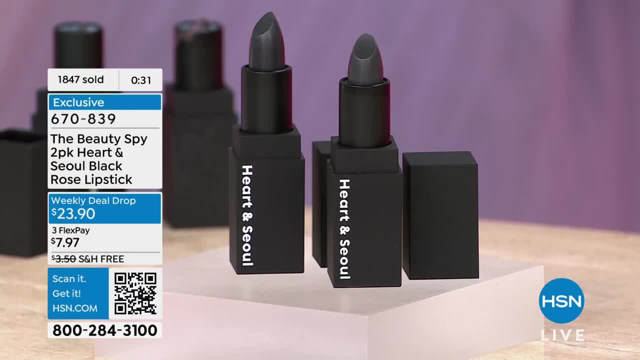 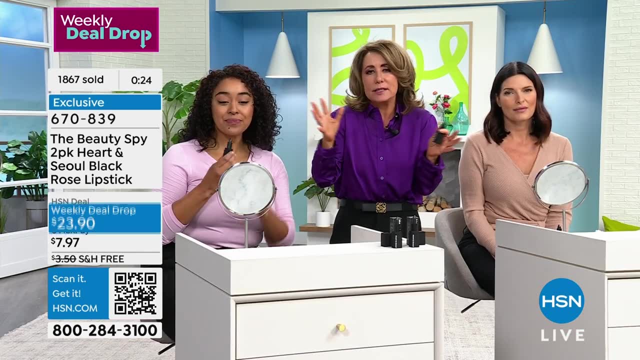 the shelf life of the lipstick, because everybody's getting uh more than one so easily, three years from the time that you, you know that you open them. so okay, yeah, just keep them like in a nice place, obviously not in the heat. just put them, you know, under the sink or somewhere you know where they'll be taken care of. you don't. 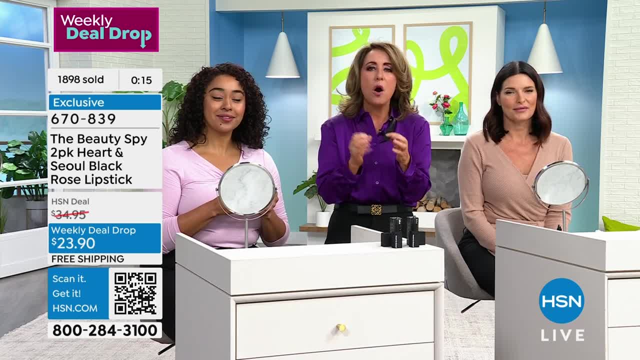 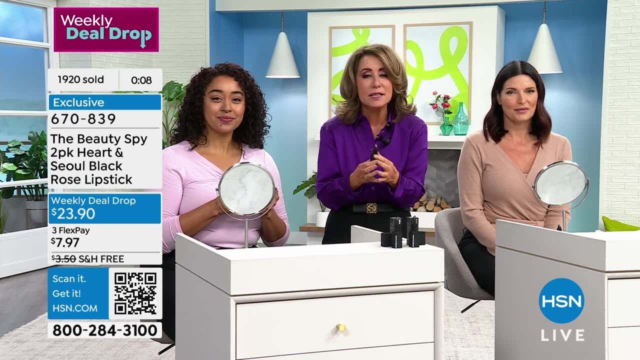 want to have them in heat. other than that, you guys are good to go. it's heart and soul. it really is a unique opportunity and i know i sound really excited. i i get this way with this product because we only can get it once a year. so i'm not trying to rush anybody, but if you've read